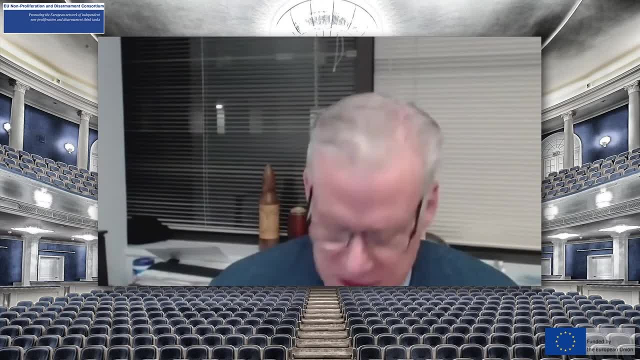 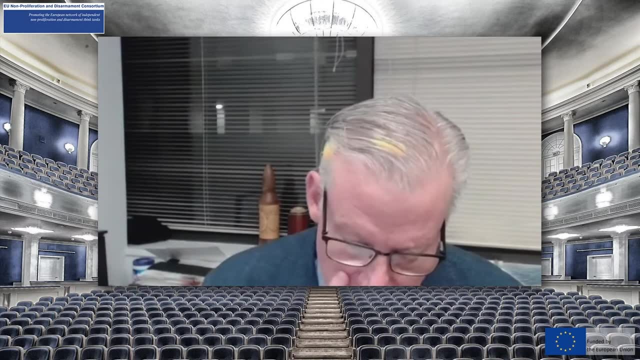 And so I really welcome the opportunity to be able to chair this session, And we have three great speakers, which I- whom I will introduce shortly, but I want to thank the consortium IAI and the organizers, Federica and everyone, for the opportunity to chair the session. 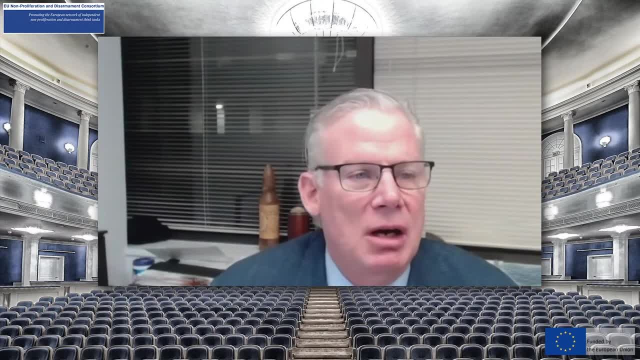 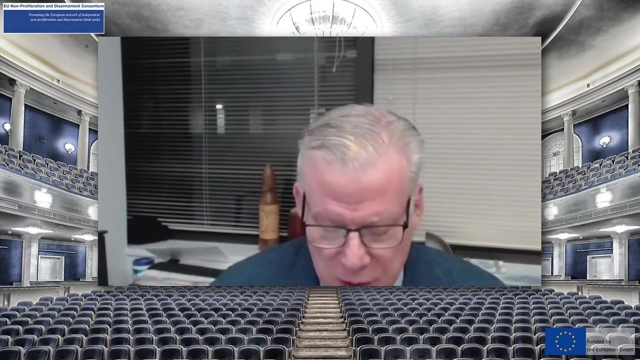 Now the title of our session is quite clear and I think everyone knows what it's pointing towards. You know I look. I've been looking back at arms control agreements that have occurred over the last six, seven centuries and there have been about 40 notable attempts to ban or control different types of arms and we really haven't seen much success, except during the Cold War. 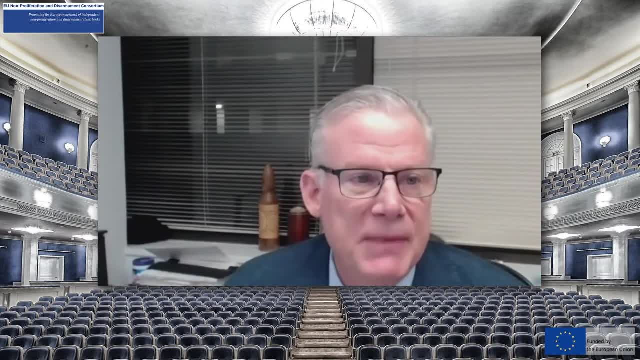 And, in fact, arms control became a central feature of the Cold War, where the mechanisms of arms control and the outcomes- And, in fact, arms control became a central feature of the Cold War, where the mechanisms of arms control and the outcomes sought to slow the arms race or the arms buildup, the number of weapons. we might call it quantitative arms control. But they also examin�� the means to control the quality of some of the weapons with the multiple independently retargetable reentry vehicles, things of that nature, improvements in accuracy. but they also examin disrupted, difficult and unusual weapons. But they also examin distorted, uns, expedited similar orders, regardless of the type of operation or movement. 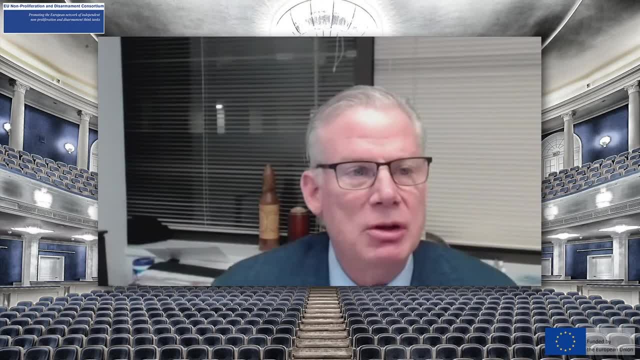 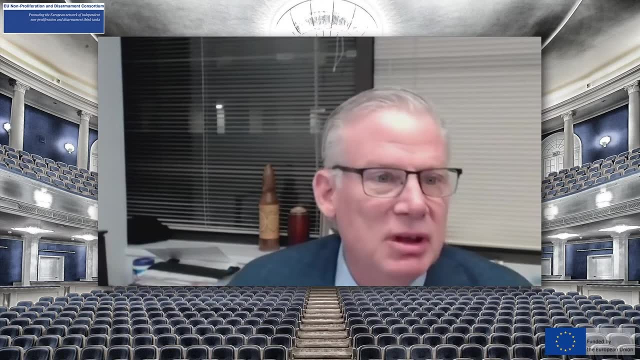 But they also examin distorted, uns, expedited similar orders, regardless of the type of operation or movement. While they failed to simulate or see despair in our city, they ended up chat fighting it like every day, Exactly Just like some決ting giving you some ideas in the media. they need to be controlled. 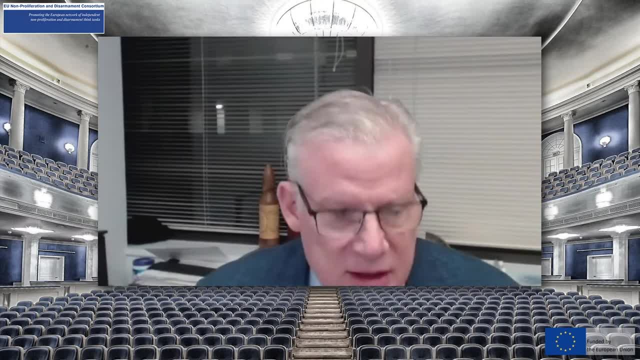 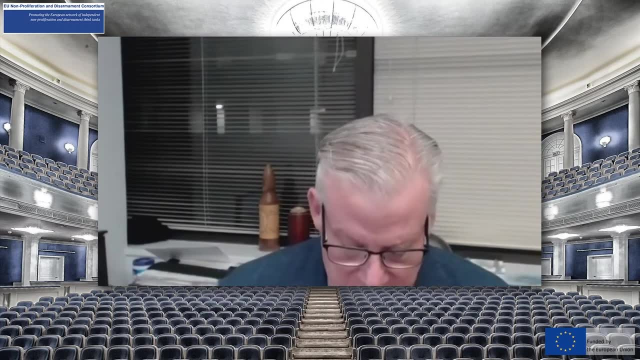 like some regulations on37, they need to be reformat. So you had those two features, and I think it was Thomas Schelling and some of the early thinkers during the nuclear era that described arms control as a mechanism for strengthening strategic stability, whether you're talking about crisis stability or arms racing stability. 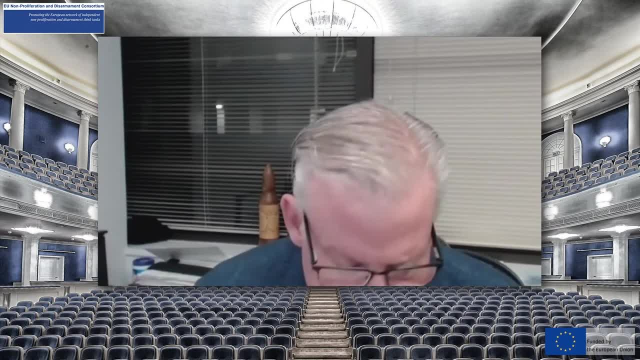 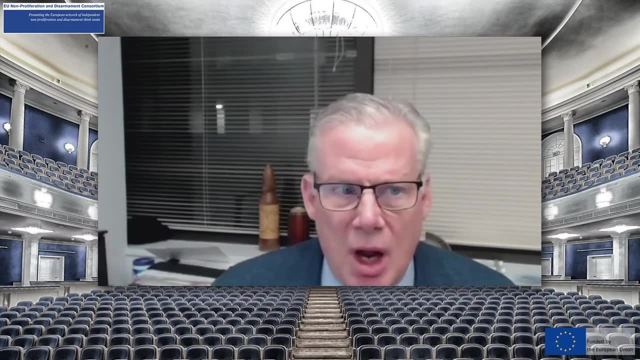 And then that's in fact what you saw during the Cold War, once the Soviet Union kind of caught up in terms of the numbers and the quality of their weapons relative to the United States. Arms control also provided greater predictability and, as a result, some confidence between the two sides, knowing that if you had some mechanisms to—. 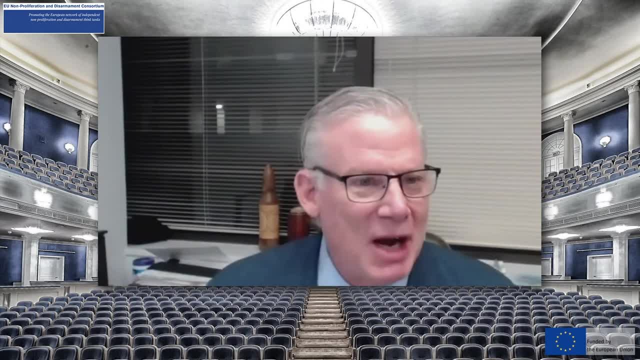 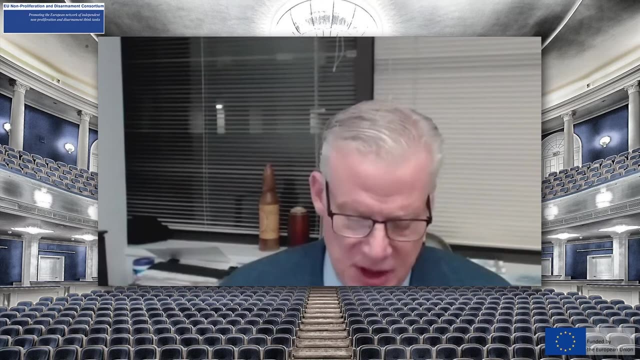 moderate or manage the behavior of your opposite number. you could have greater assuredness that you weren't falling behind. you didn't have to spend on all sorts of contingencies, And I think that's often lost as one of the beneficial aspects of arms control. 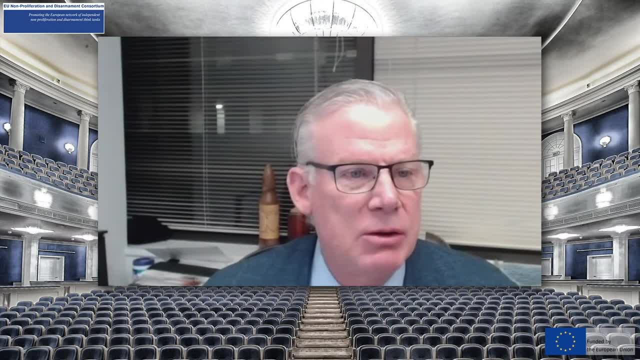 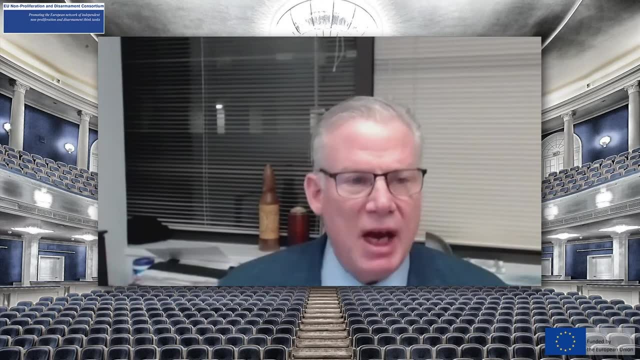 Now there was also what I call a collateral aspect to the arms control process, And that was dialogue. The strategic dialogue that was held between the Soviet Union and the United States was actually very important. Both countries were able to better understand the thought processes, the risk assessments that their opposites were making. 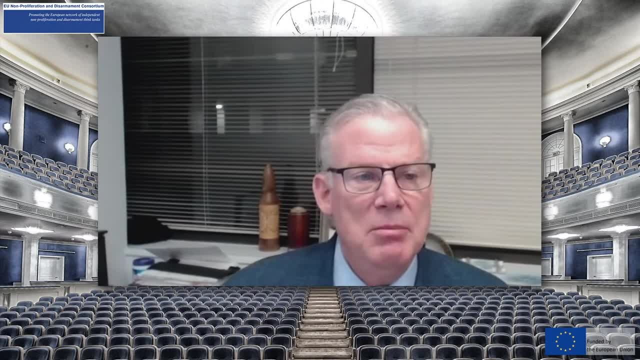 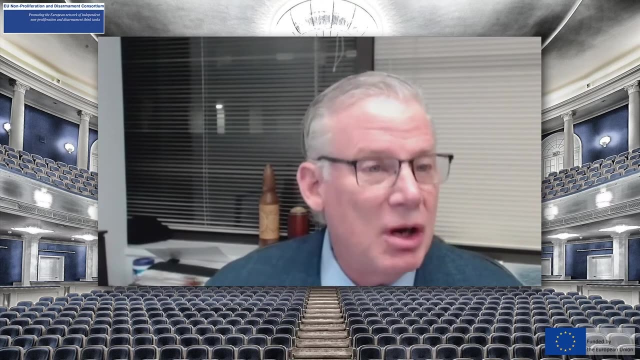 And I think this contributed maybe not so much to the fact that the Cold War never went hot, But when the Soviet Union— When the Soviet Union collapsed in early 1990s- you saw an ability of the two sides to talk to each other and for the kind of peaceful resolution to the Cold War. 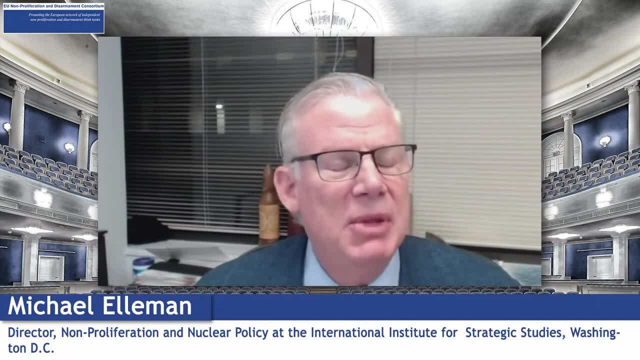 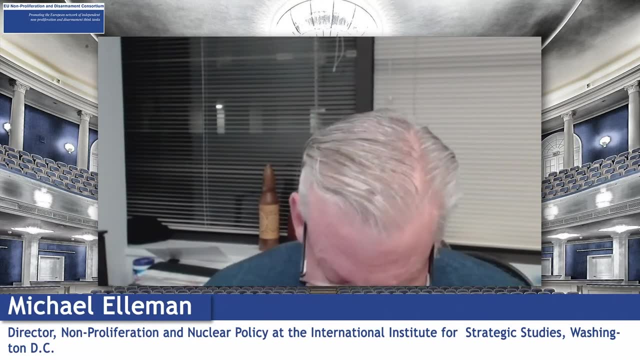 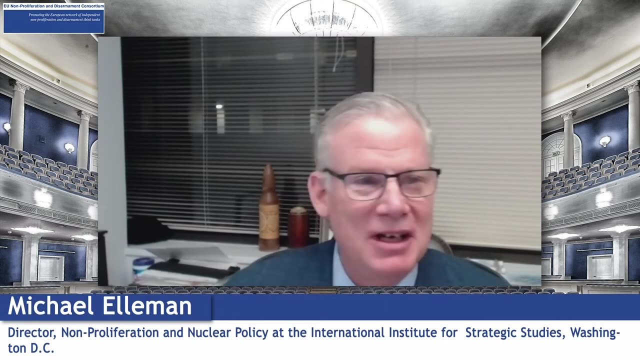 I think that's often overlooked by some strategic thinkers in terms of the values of arms control. Unfortunately, since about the turn of the century, we've seen the crumbling. Unfortunately, since about the turn of the century, we've seen the crumbling. And I think that's one of many of the very fundamental aspects of the Cold War. I mean it started with the United States choosing to withdraw from the anti-ballistic missile treaty, which was to me one of the most important aspects of the early arms control agreements. 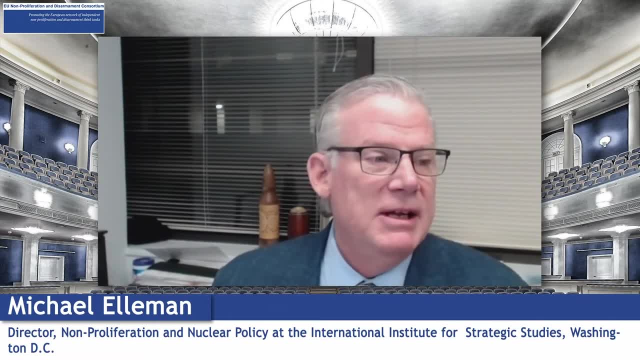 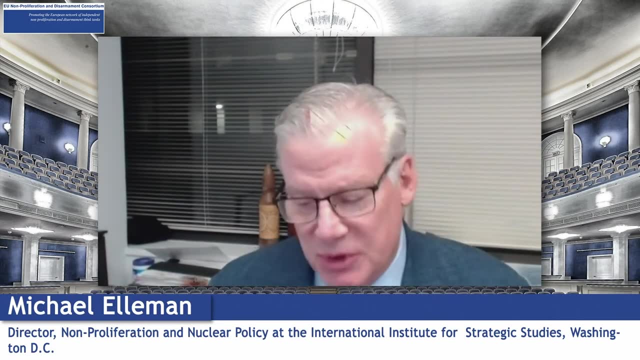 Because they tried to one tamp down the expansion of these defenses and you know the resulting expansions of offenses to overcome the defenses. Because they tried to one tamp down the expansion of defenses and you know the resulting expansions of offenses to overcome the defenses. 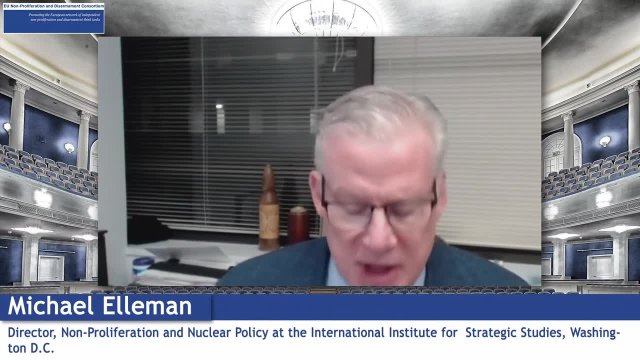 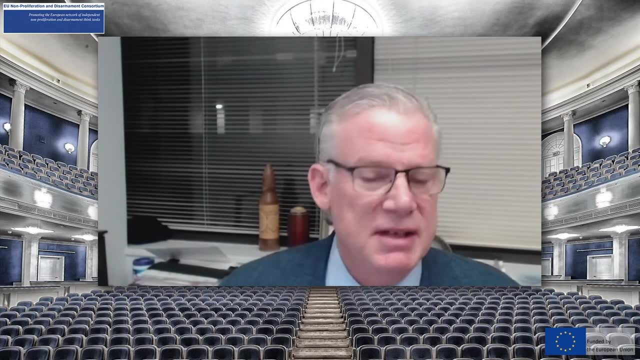 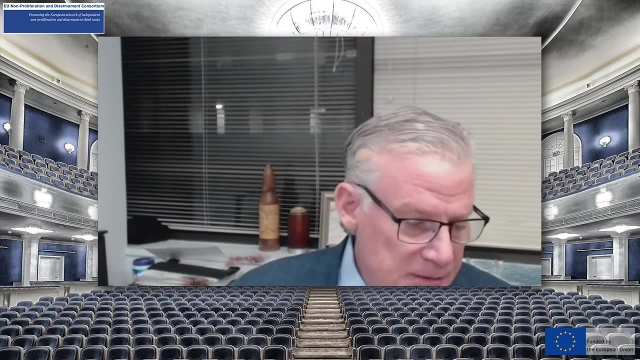 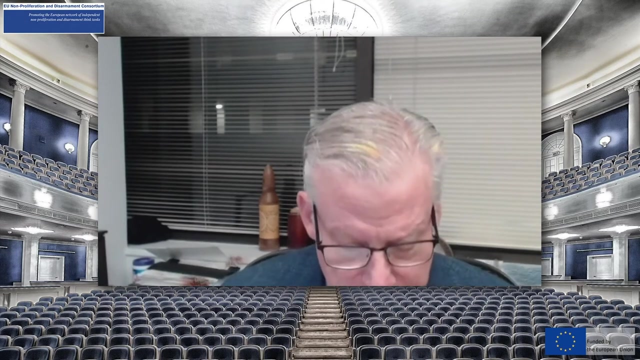 It would really have become not only an arms race nightmare, but it would have threatened crisis stability, And we see some aspects of that playing out today in the discussions between the Russians and the United States. So the—I guess the evaporation of the ABM Treaty was kind of a beginning of what we see today in more vivid colors. 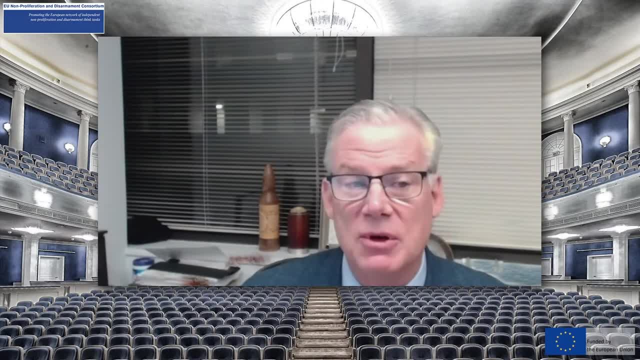 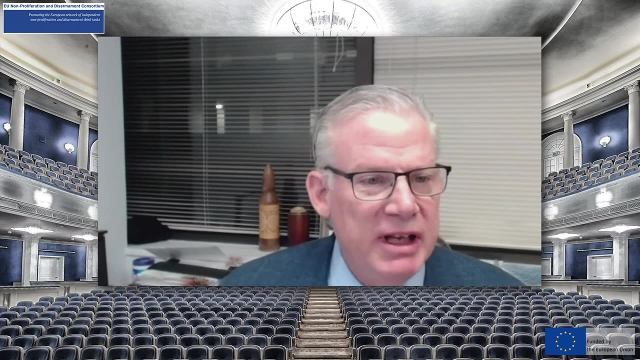 The collapse of the— I think many of our younger participants weren't around during the height of the Cold War- and the value of actually banning a weapons category. It was a very seminal event in the Cold War And I think it led to a lot of what happened after 1987. 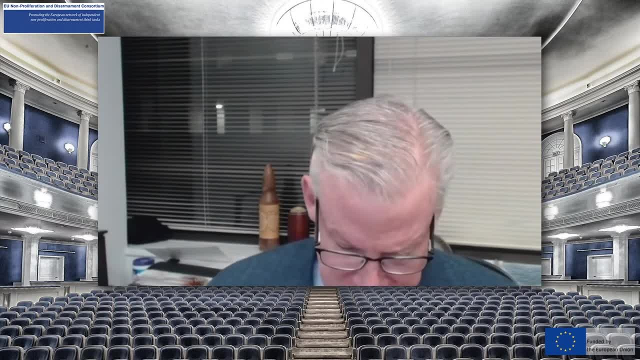 And unfortunately that treaty is no longer in force. But it'll be interesting to see, if there is a—with the election of Joe Biden to be the president of the United States- whether there's a resumption of arms control discussions. But you know, just this week the US withdrew from the Open Skies Treaty. 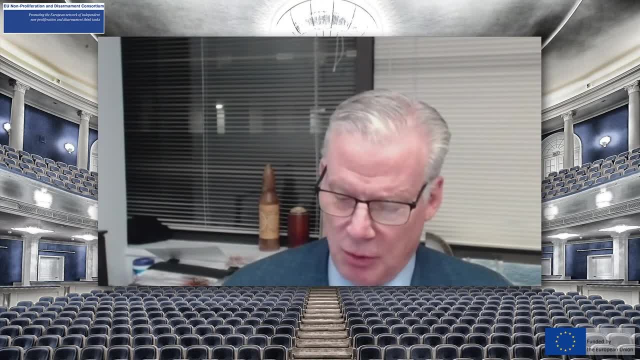 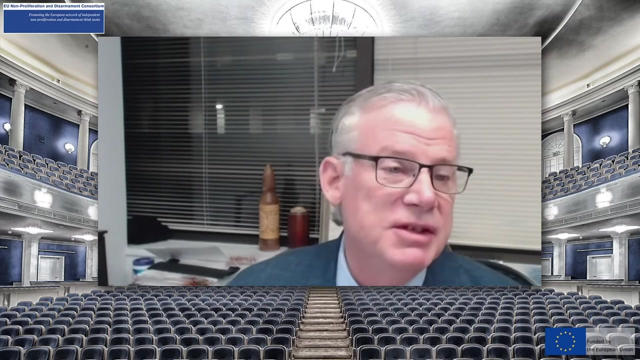 I'm still at a loss to explain exactly why they had made such a decision, because their arguments, in my view, were quite weak And the New START renewal process ground to a halt for a number of reasons: Missile defense is one, but also the desire on the part of Washington to include China. 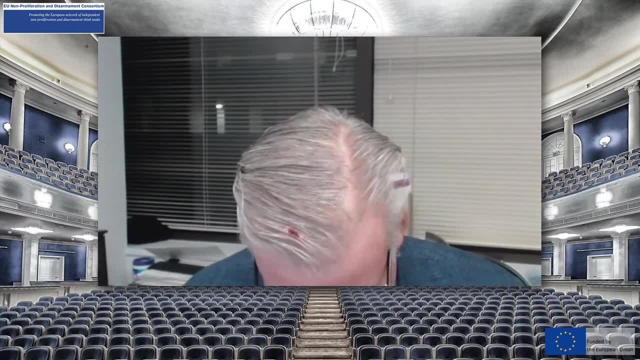 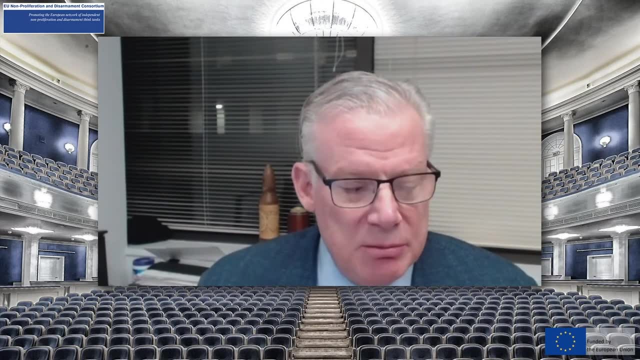 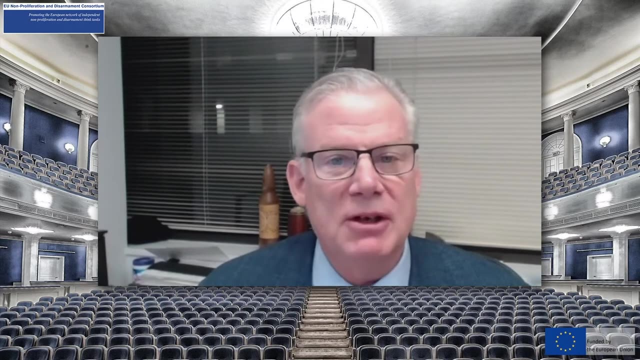 In those talks it seemed to be a real stumbling block. There were others as well, And this raises an important question. I mean, bilateral agreements are very difficult to reach. Trilateral or multilateral are going to be even more difficult. And what does that say about the future of strategic arms control for nuclear weapons? 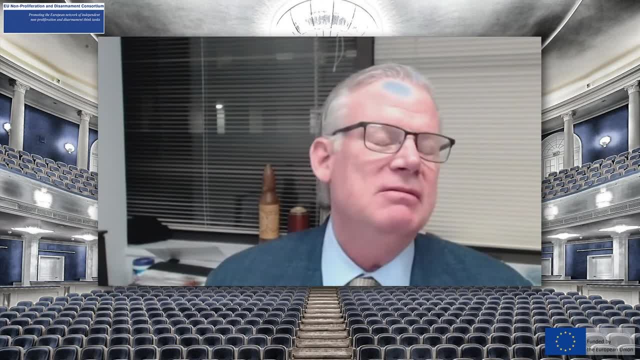 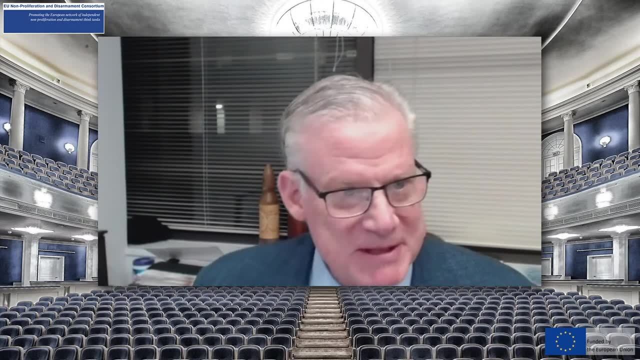 If the major powers don't start reducing their weaponry, as they have committed to do under the Nuclear Nonproliferation Treaty, what becomes of that? We're already you know—. We've also seen the US withdrawal from the JCPOA. 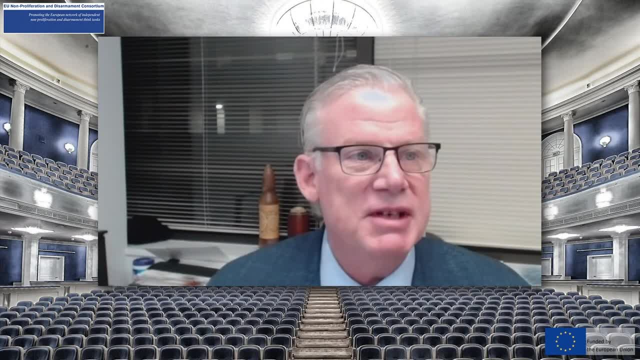 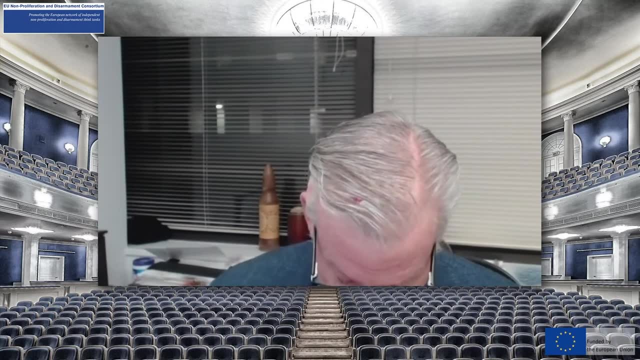 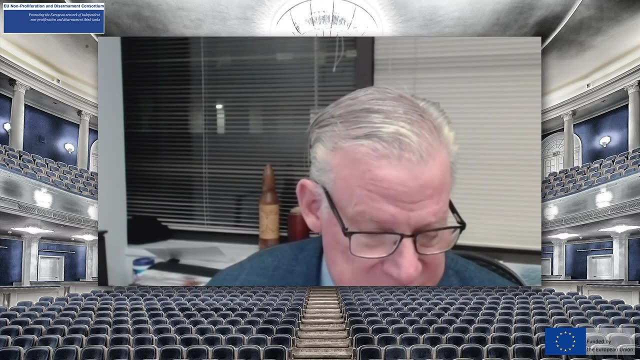 There was a failure to really go into serious negotiations with North Korea. So the proliferation of weapons is going to be first and foremost in the minds of many going forward. So with that kind of scene setter, I'd like to turn to the assigned speakers for their thoughts on this. 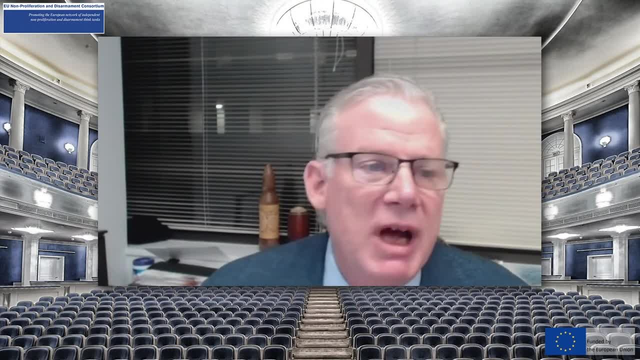 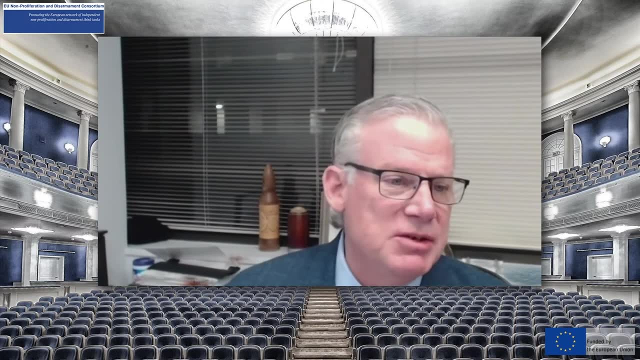 I'm very excited to hear what they have to say. You have their bios, I think, in the packets, But I'll give a short introduction with each of the speakers as they come on. We'll start with Naomi. She's a PhD candidate in political science at Cornell University, where she researches the politics of multilateral arms control, nonproliferation and disarmament. 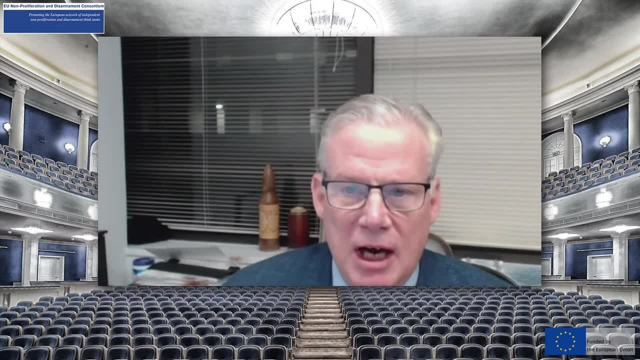 It's also the subject of her dissertation. Naomi is also the Jan Dolan Nuclear Security Visiting Fellow at the US Department of Defense. She's worked at the Truman Center for National Policy. She's worked at the Council of Foreign Relations. 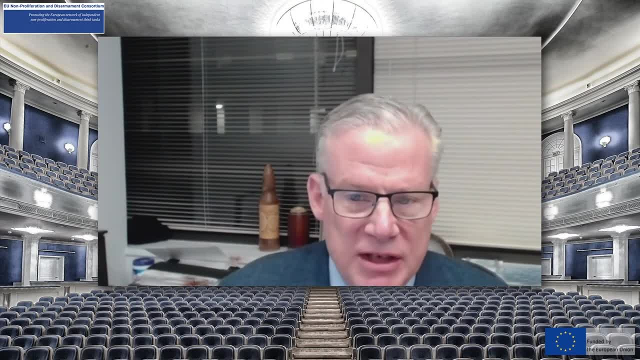 She's published in the Nonproliferation Review And she has a bachelor's from the University of California, Berkeley- Go Bears, Sorry, I couldn't help myself- And an MA from Cornell University. So with that I want to hand, I guess, the microphone over to Naomi. 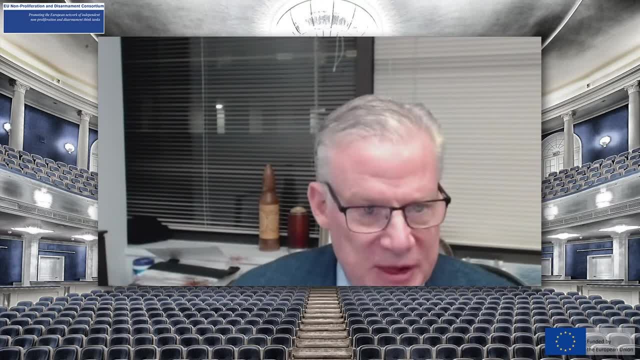 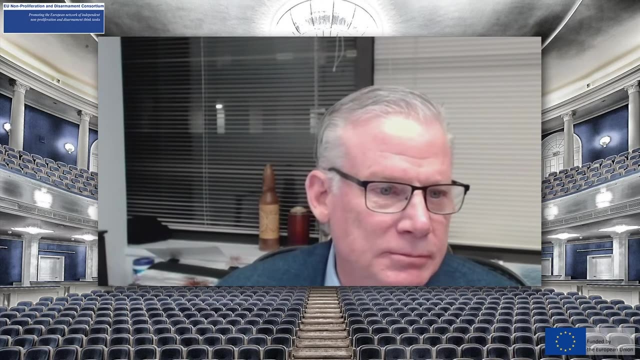 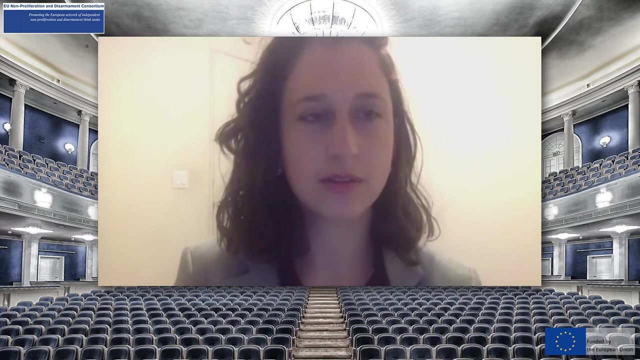 She'll speak for about 10 minutes And then she'll be followed by the other two speakers And then we'll move to questions and answers. Thank you, Naomi Great. Thank you so much, Mike. Just one second while I get my slides going. 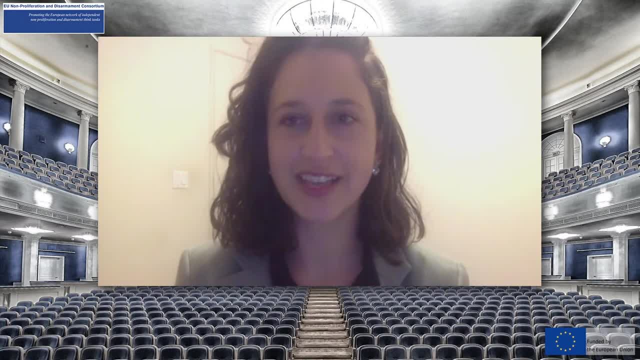 There we go. Can you all see my screen And can you hear me? Great. So I'm delighted to kick off this panel on the future of nuclear arms control and nonproliferation in an era of crumbling treaties. And I'm going to be a little bit provocative today and ask whether arms control and nonproliferation 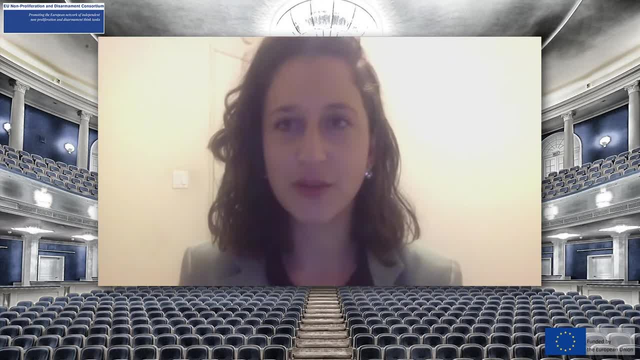 really is crumbling. I'll then assess what's new and different about this current moment And, looking towards the future, I'll offer a menu of options for how we can think more expansively going forward. So first I want to question whether arms control and nonproliferation really is crumbling. 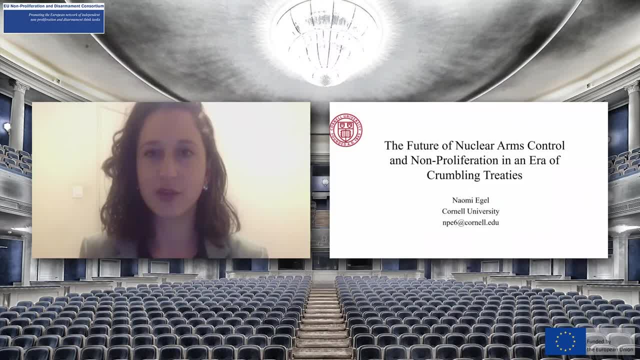 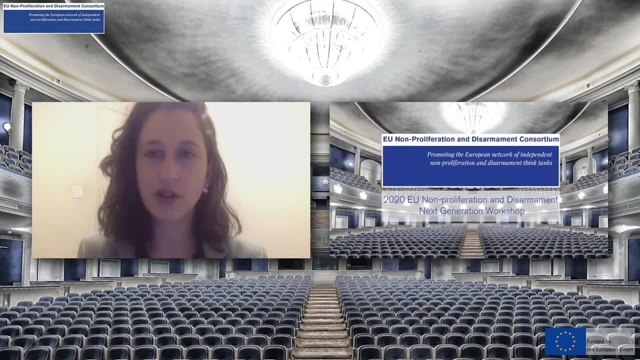 So first I want to question whether arms control and nonproliferation really is crumbling quite so much as we often say it is. The first point I want to make is that arms control and nonproliferation has never been easy. 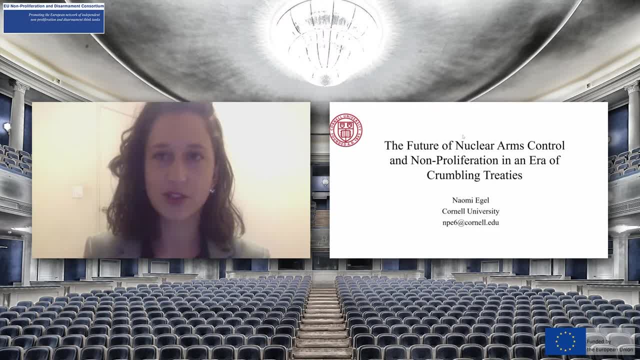 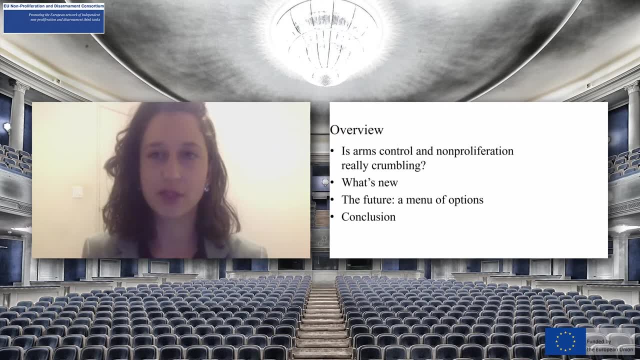 To take one example, the NPT, which is, of course, the cornerstone of the nonproliferation regime and one of our most successful agreements. the NPT took over 10 years from when it was first proposed by Ireland to when it opened for signature. 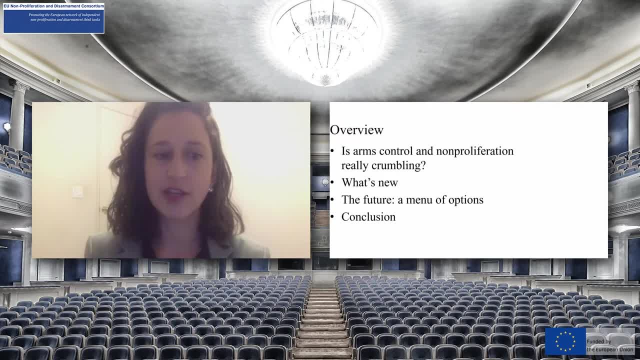 And treaties are preceded by years of confidence-building measures, And my interviews with negotiators from different treaties and different decades emphasize the time it took for trust to be built up. Agreements are never certain until they happen, and it's striking how much of some of the 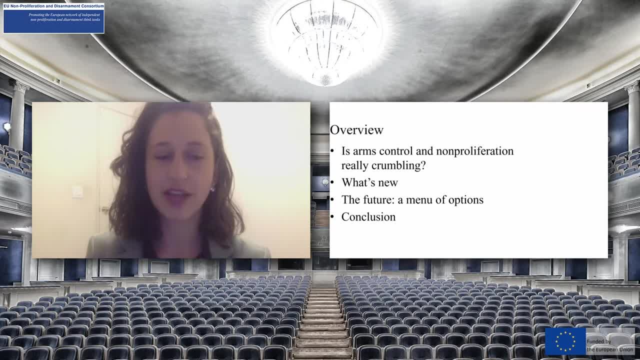 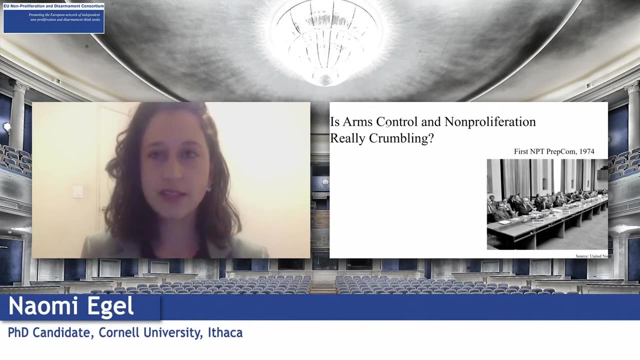 core components of treaties is agreed only at the last minute, And so we shouldn't underestimate the difficulty that past negotiators had in reaching agreements. The second point I want to make is that we have to understand that the long-term goal of a treaty is to be a noncompliant treaty. 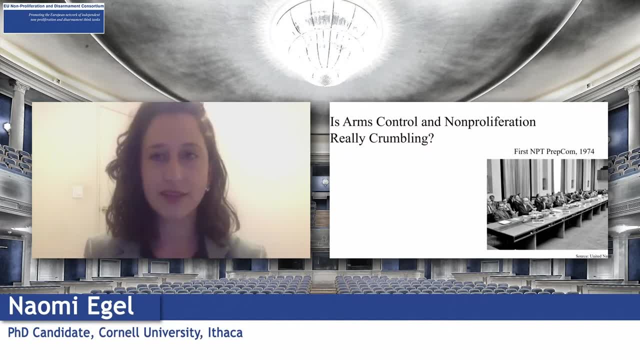 The second point I want to emphasize is that compliance is rarely perfect. Compliance is something that is assessed, not assumed, and many agreements have mechanisms for dealing with challenges to compliance. For example, New START has the bilateral consultative commission. Now, that's not to say that compliance is never a fundamental challenge to treaties. 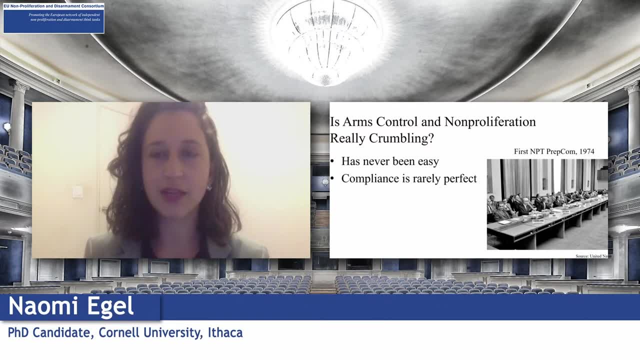 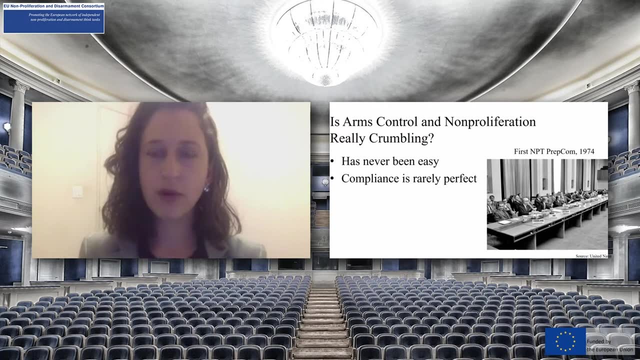 and issues of noncompliance are not. but it's to say that noncompliance can, under many circumstances, be dealt with within the context of a treaty. But the second point I want to emphasize is that compliance is rarely perfect. But the third point I really want to emphasize is that pessimism towards arms control and 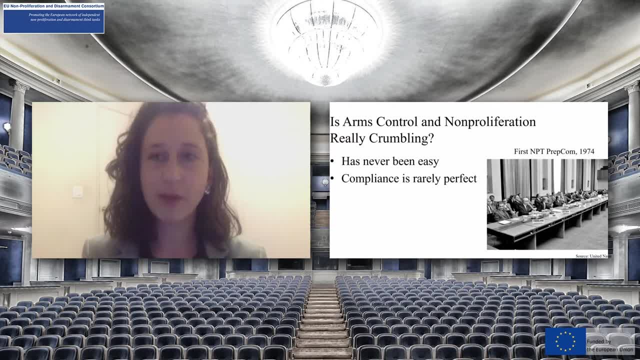 nonproliferation is also not new. Today, many policymakers and analysts emphasize how challenging the political environment is to making progress, the lack of political will and the need for new leadership. But if you look at writings from the 1990s, 1980s, 1970s or 1960s, you'll see similar 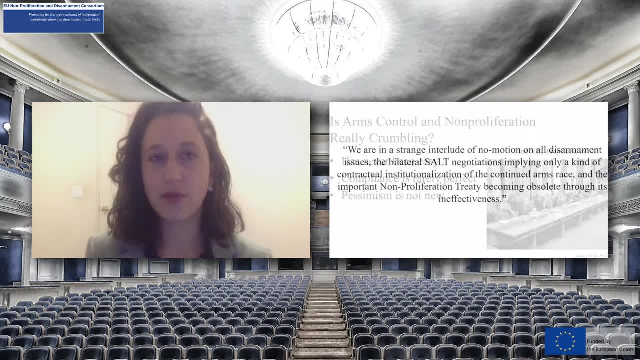 statements. So this quote, for example, that we are in a strange interlude of no motion on all matters, on all disarmament issues, the bilateral SALT negotiations implying only contractual institutionalization of the continued arms race and the important nonproliferation treaty becoming obsolete. 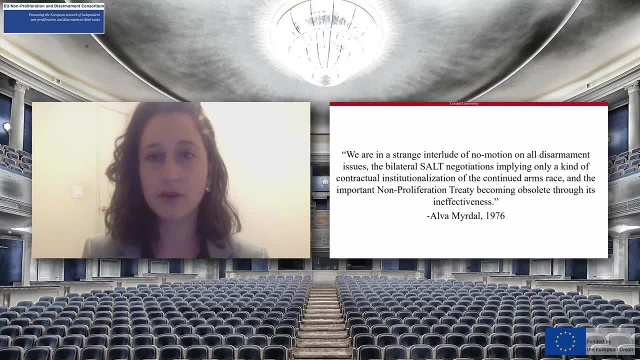 in its ineffectiveness. This is a quote from Oliver Murnall, who was the Swedish representative to the NPT negotiations and many other negotiations, And it's a quote from 1976. And yet it's striking how similar it is to much of the discussions around arms control. 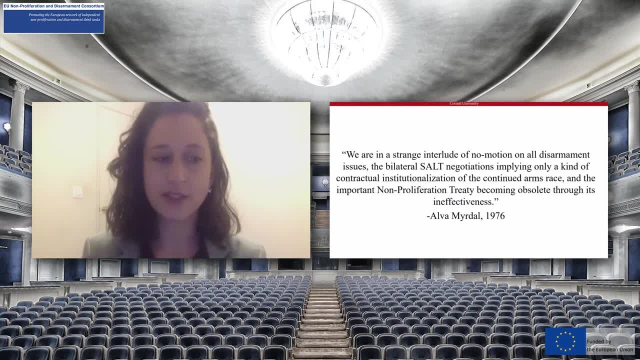 and nonproliferation today. To take another example, the Belfer Center's Stephen Miller wrote in 1980 that the previous 25 years of arms control contain as many failures as successes, has had little impact in terms of limiting the arms race or reducing the risks of war, and is to quote dead in the 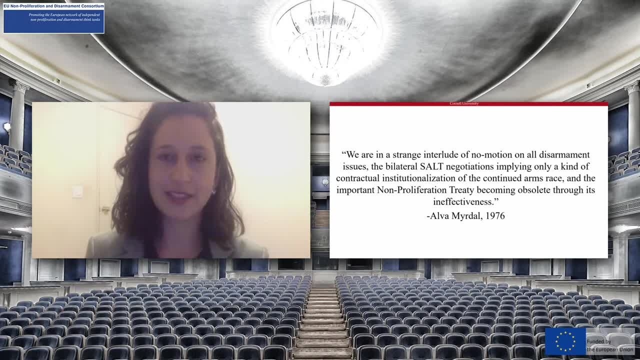 water, And I think, looking back at the 1960s and 1970s, we might assess that situation slightly differently today, And so the point I want to make is that it's easy to look back and say that things have been obvious in the past, but they weren't obvious, and that many of the same challenges 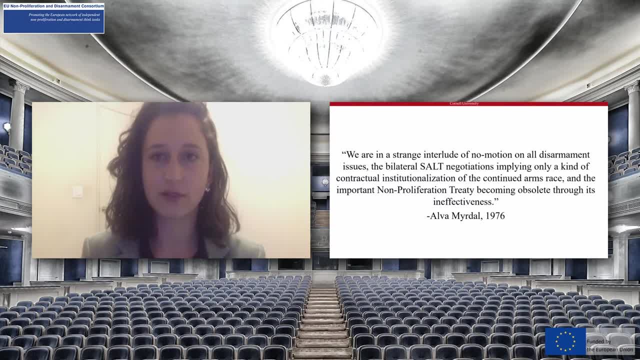 we find ourselves facing in arms control and nonproliferation today are perhaps not new, but are perhaps challenges, because arms control and nonproliferation is hard to do Now. that's not to say that there's nothing new or different about our current situation. 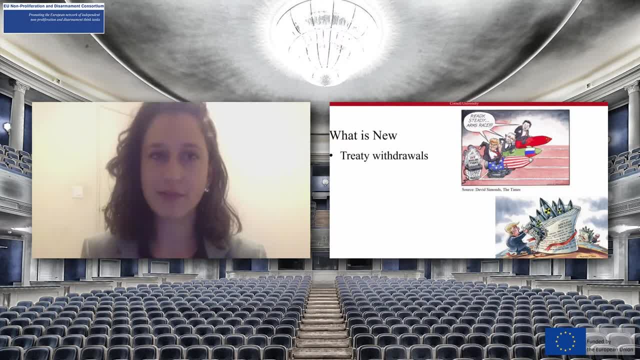 today And of course, the most obvious example is treaty withdrawals, particularly by the United States. This does pose a serious challenge and it is more frequent than in the past, But I do also want to stress that the response from others, particularly in Europe, condemning 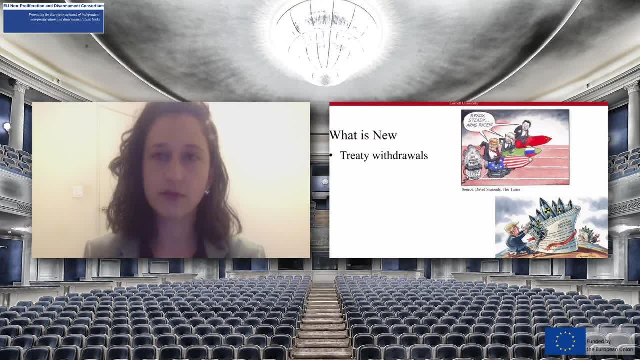 such actions indicates that there is still strong support for these treaties and the commitments in them, And European states have been pressuring the US administration to return to these treaties, and we'll see what happens in the upcoming months with the new US administration. 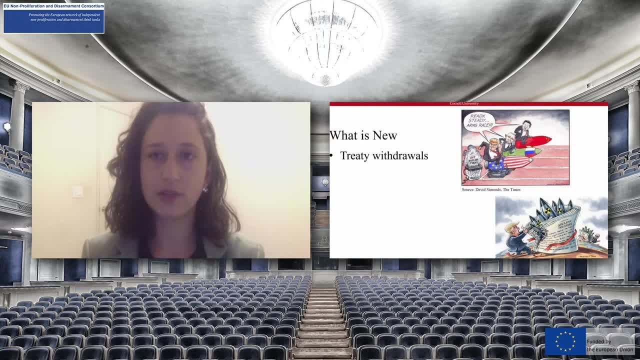 But the Biden administration has already prioritized extending those treaties And we'll see what happens in the upcoming months with the new US administration. But the Biden administration has already prioritized extending those treaties And we'll see what happens in the upcoming months with the new US administration. 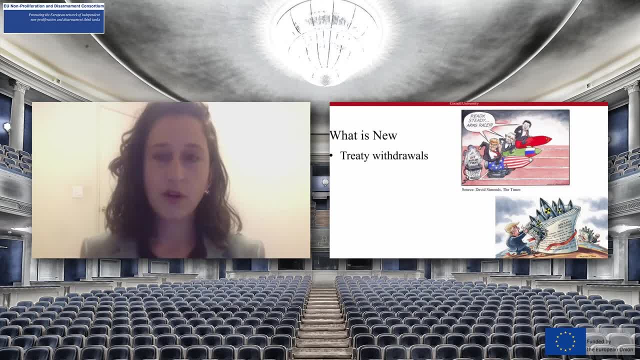 And we'll see what happens in the upcoming months with the new US administration, So as the US administration continues to set itself up for a new start and returning to the JCPOA—moreover, although withdrawal is clearly not a good thing for treaties, the effect depends on a specific circumstance. So to take a treaty that is not technically a nuclear treaty but has been in the news quite a lot lately, if the rest of the parties to open skies continue their overflights, the effect of US withdrawal is more muted. And withdrawal does not necessarily lead to the collapse of agreements. For example, North Korea's withdrawal from the NPT did not lead to the collapse- not lead to the collapse of the NPT Now. changing geopolitics certainly do pose a challenge for arms. 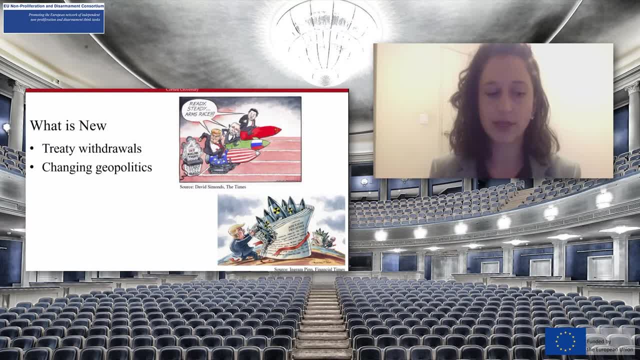 control and nonproliferation. Arms control has primarily been a US-Russia endeavor And yet, as we all know, China has risen as a global power and a geostrategic competitor. Now, as we also all know, China has far fewer nuclear weapons than either Russia or the United States, and is 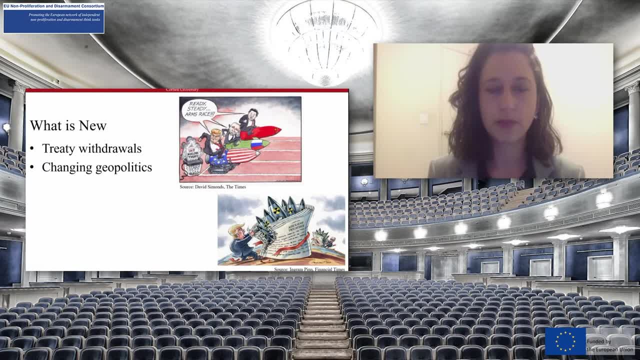 consequently disinterested in participating in arms control, And so the situation makes arms control poorly suited to alleviate the tensions between the United States and China, And yet at the same time these tensions inhibit cooperation between the two countries on nonproliferation. The third challenge is domestic challenges to treaty ratification, particularly in 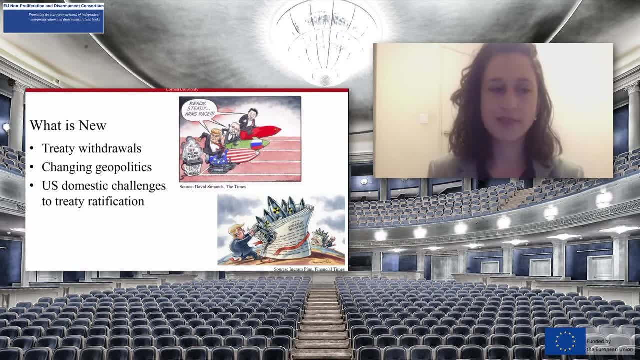 the United States, But I also want to point out that this may not be as new as it seems as well. In 1998, former arms control negotiator George Bunn was already writing about the need to pursue informal alternatives Given the challenges to treaty ratification. in the US Senate we see many similar recommendations. 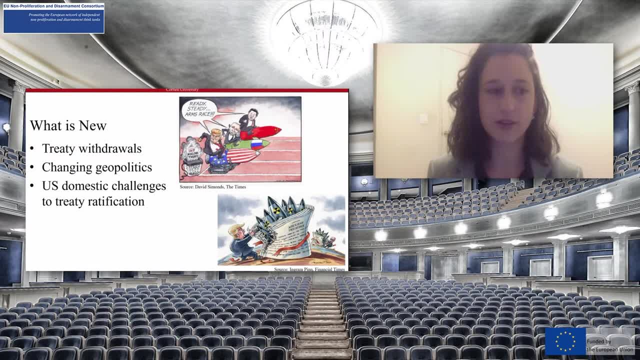 today to the recommendations he was making over 20 years ago, And it's also important to assess what exactly challenges to treaty ratification prevent. So, for example, extending New START does not require ratification by the US Senate, And so, in this vein, it's important to think about: 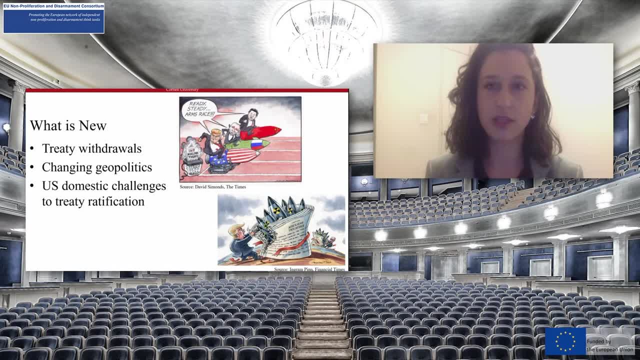 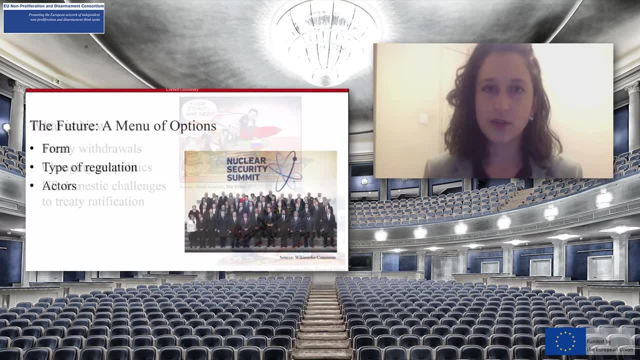 how we can make progress on arms control and nonproliferation in ways that minimize the domestic challenge. And so, in this vein, looking towards the future, I want to offer a menu of options for making further progress on arms control and nonproliferation. These options offer a more expansive view than 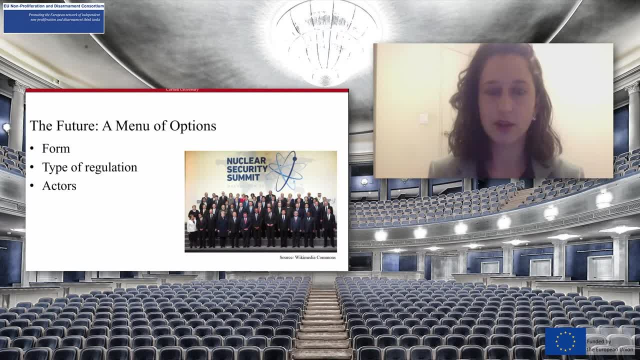 sticking to the models of the NPT or bilateral US-Russia arms control, And they also involve a wider array of actors than the nuclear weapon states alone. So the first set of options concerns the form that these agreements can take And, of course, one 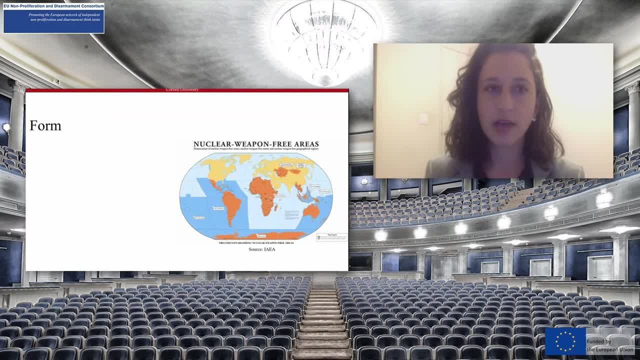 important distinction is whether they're legally binding or not, And while legally binding agreements are often seen as the gold standard, I suggest that, especially in nonproliferation, they may not necessarily be necessary. So, to take one example, export control regimes do not require treaties. 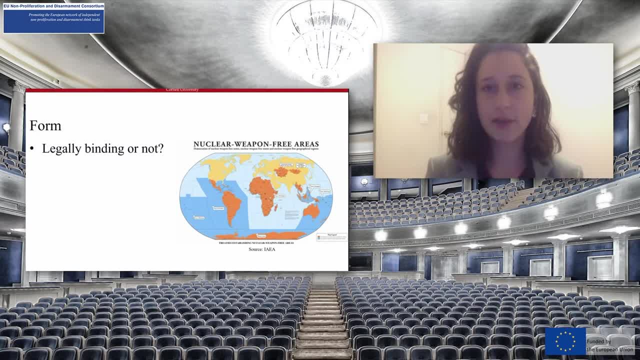 do not require ratification by the US Senate and have been incredibly important in limiting the spread of nuclear weapons worldwide. Another important question is whether agreements should be bilateral or multilateral, And I think that's a really important question And I think that's a 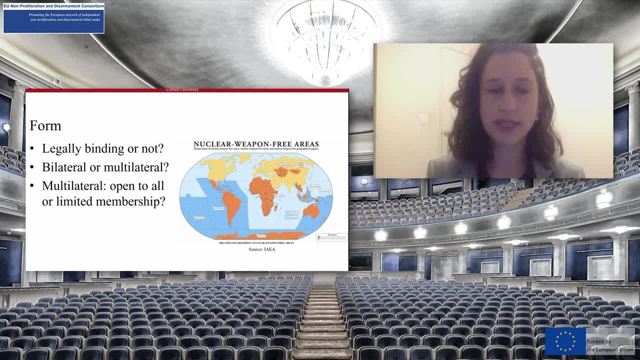 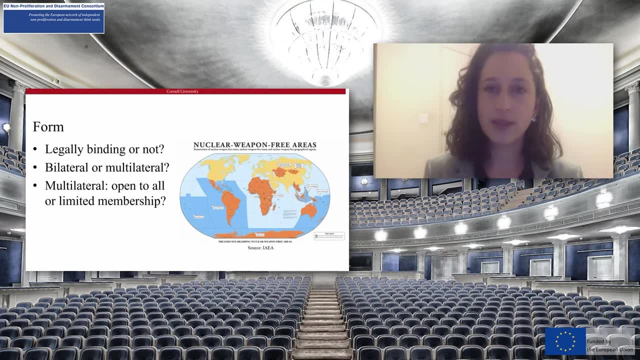 really important question- And I think that's a really important question- And if they're multilateral, whether they should be open to all states or limited in membership. So, for example, nuclear weapon-free zones are limited by their geographic membership, whereas other initiatives. 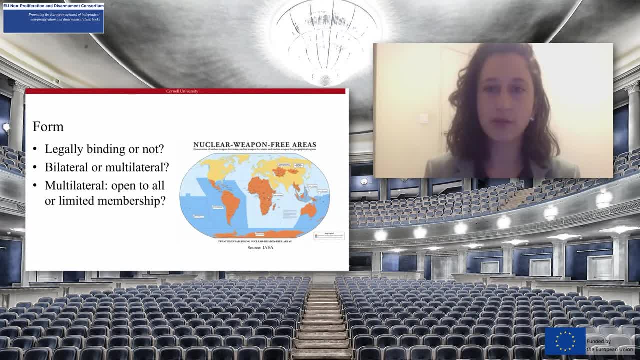 like the Nuclear Security Summits or the G8 Global Partnership, are limited by political factors. But the point I want to stress is that, rather than assuming one form should be what we are striving for, we should assess what actors and what form of agreement is most conducive to. 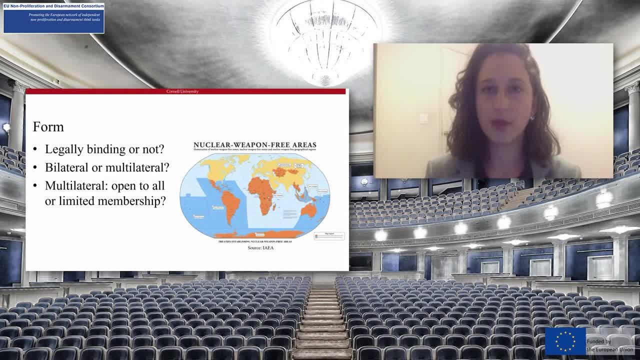 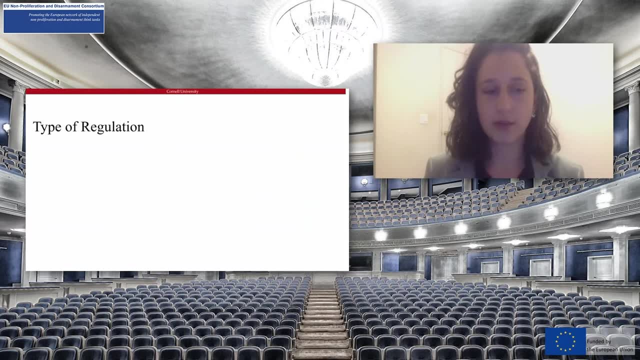 advancing nonproliferation or arms control, And I think that's a really important question, And I think that's a really important question, And I think that's a really important question. The second type of option I want to explore are the types of regulation, And here I identify four. 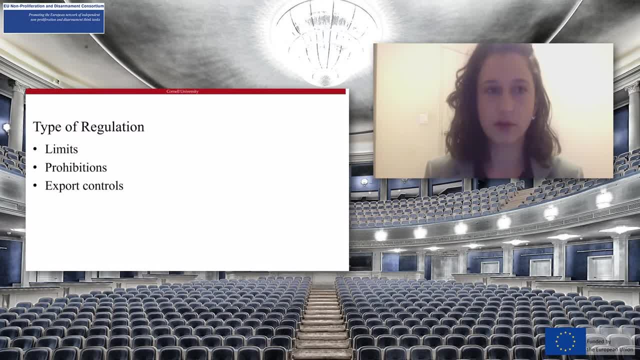 types of regulation involved in arms control and nonproliferation. Limits and prohibitions refer to limits on weapon systems delivery vehicles, as well as behavioral limits and prohibitions referring to what systems can be deployed and in what numbers. I've already mentioned export. 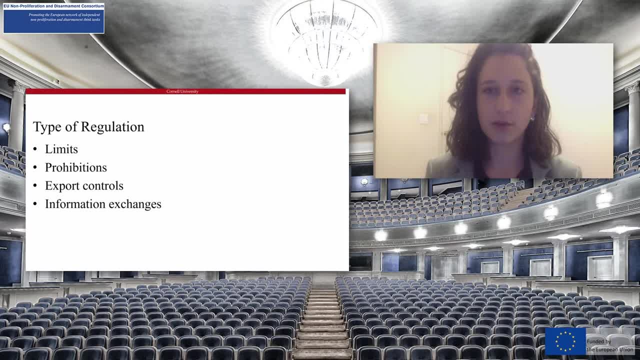 control, which is a very important element of the US Senate, But I think that's a really important controls, but these are a fundamental element of a nonproliferation regime. And finally, information exchanges, which receive far less attention than some of these. 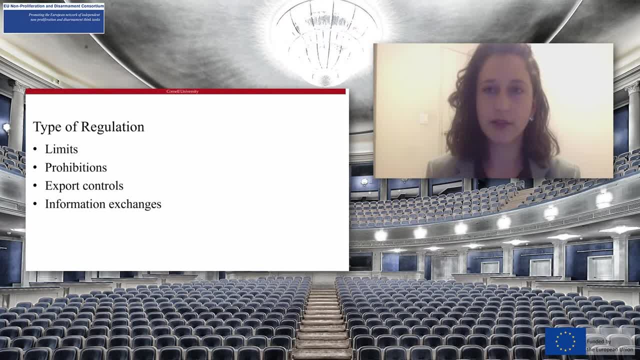 other types of regulation, but are an essential component of any arms control or nonproliferation agreement, an essential precursor to any of these other types of regulation. The last set of options I want to explore is sources of leadership for arms control and nonproliferation, and here I want to stress the importance, as we move forward, for leadership. 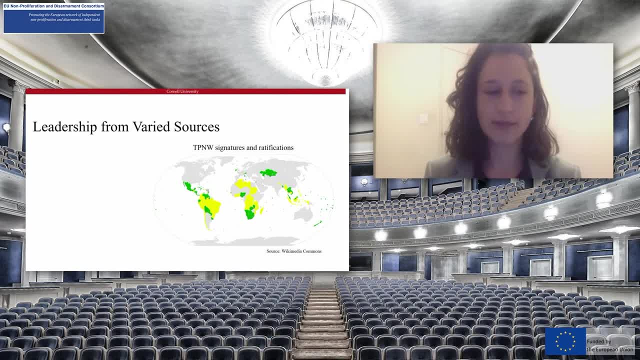 from beyond nuclear weapon states. So, to take one example, the TPNW has changed the debate on nuclear weapons and is an important example of an agreement not led by nuclear weapon states, but led mostly by states in the global south, although of course Ireland was very important as well, and I know Emily. 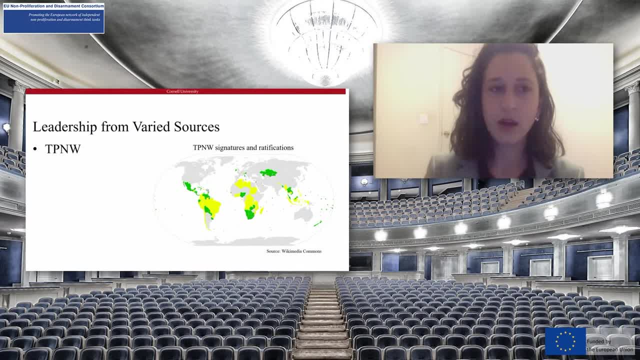 will talk more about that in just a minute. Another important example are nuclear weapon-free zones which, again, were largely led not by nuclear weapons. They were led by nuclear weapon states, but by states in the global south, And these are an important reminder that we have precedence for nonproliferation. that didn't. 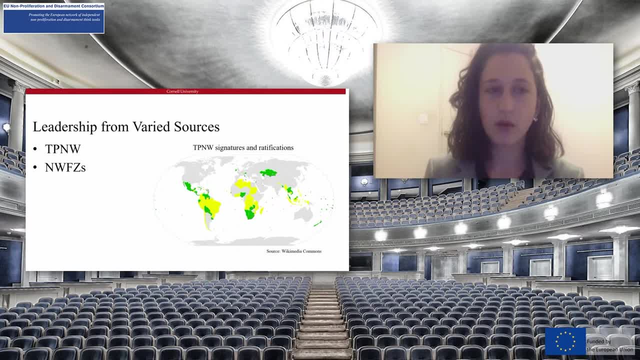 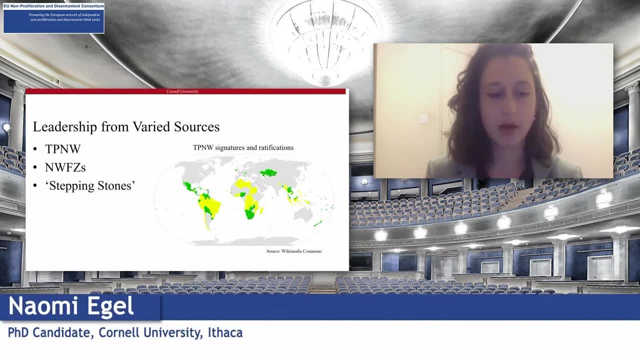 require leadership from nuclear weapon states. One third example is the stepping stones approach initiated by Sweden, now involving a wider array of states, which is a different model, not led by nuclear weapon states, And so going forward as we move away from models of arms control and nonproliferation. 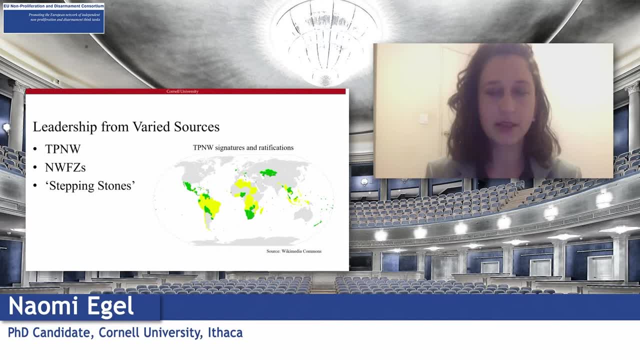 that are led exclusively by nuclear weapon states. I think the states in Europe are going to be particularly important in bringing together nuclear and non-nuclear states to advance these goals. So I'll conclude just by emphasizing that arms control and nonproliferation has always 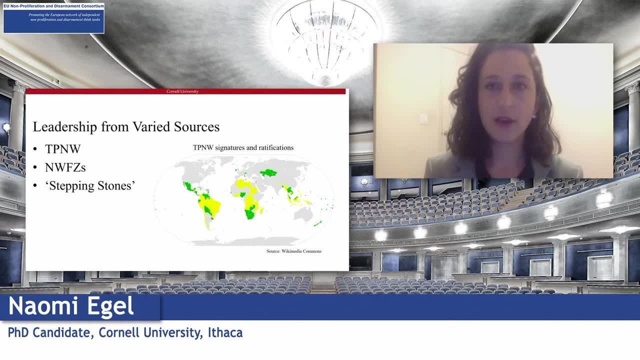 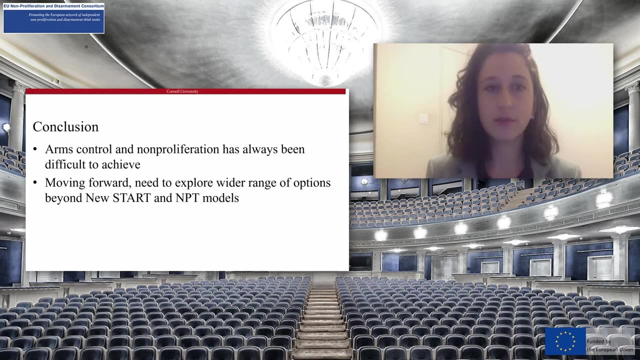 been extraordinarily difficult to achieve and that, although there are certainly challenges we face today, we should not overemphasize how different some of these political challenges are from political challenges that past negotiators have faced. Moving forward, however, we need to move beyond the model of arms control and nonproliferation. 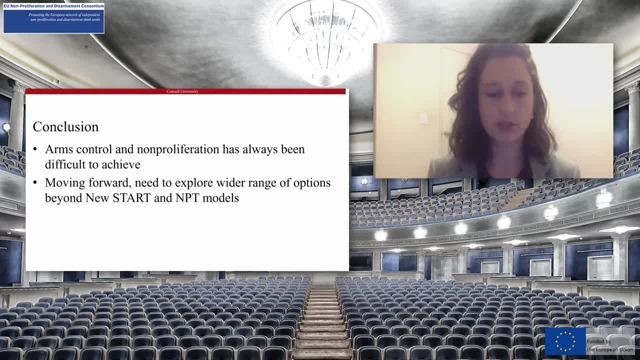 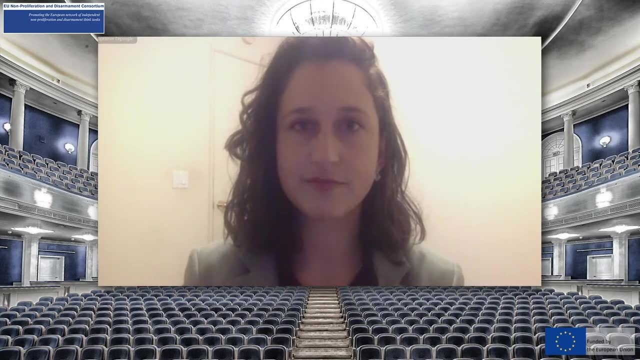 We need to look at models of NPT and US-Russia bilateral arms control and look to a wider array of forms, types of regulations and actors leading arms control and nonproliferation. Thanks very much and I look forward to your questions and comments. 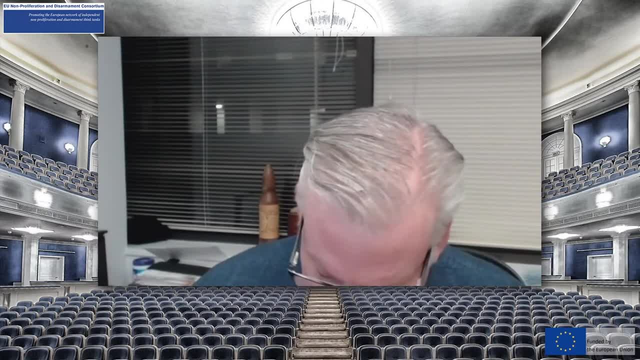 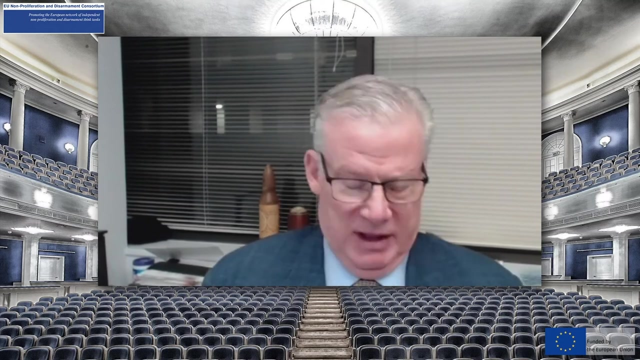 Thank you, Naomi. That was a wonderful presentation. It raises a number of questions in my mind which we'll get to after the next two speakers. I'm especially struck by the domestic component to arms control and the treaty ratification elements. As you know, here in the United States it's a pretty—well. domestic politics is a real. 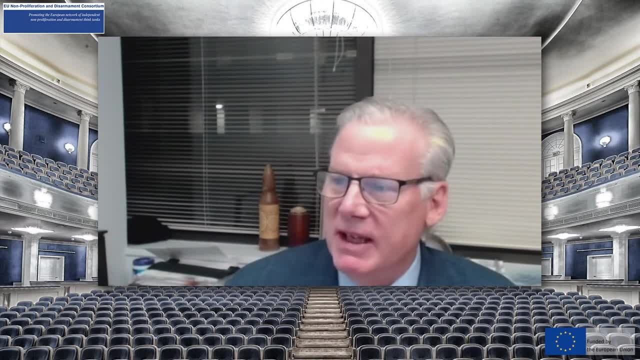 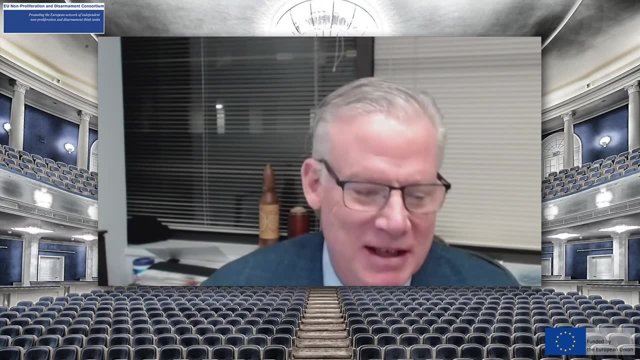 contact sport, as we say. Our next speaker is Noah Mayhew, who is with the VC and DNP in Vienna, where he's a research associate. I see it focused on nuclear nonproliferation, IAEA safeguards and nuclear verification. 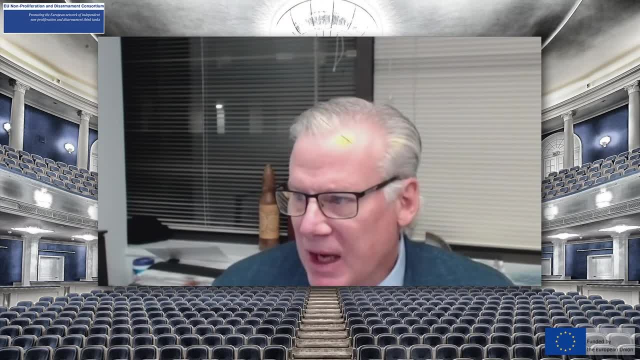 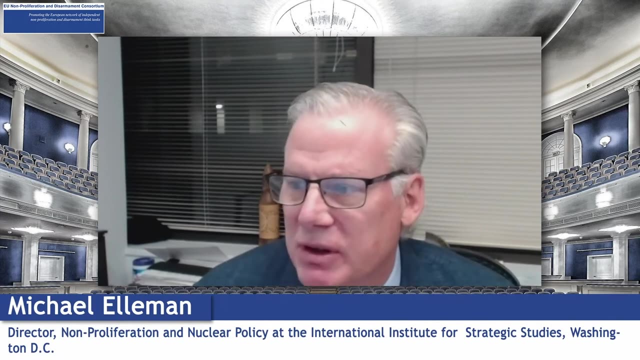 arms control in the US-Russia relations. He is widely published at such a young age, which I find impressive. He's also contributing to some of the ongoing work at the Vienna Center project on the nexus between the peaceful uses of nuclear science and technology and nuclear security. 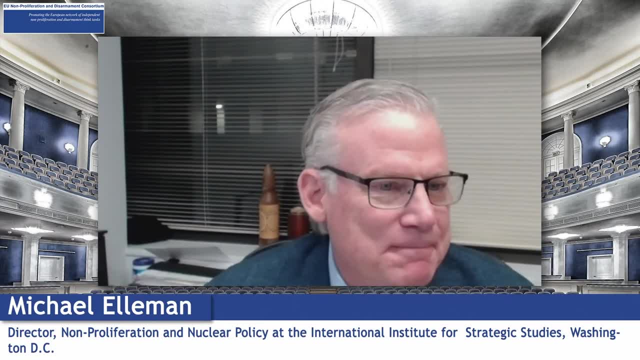 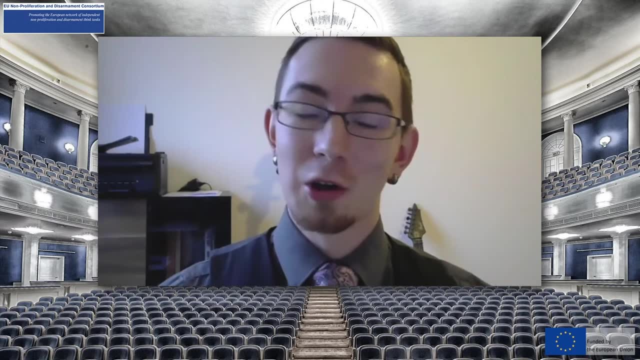 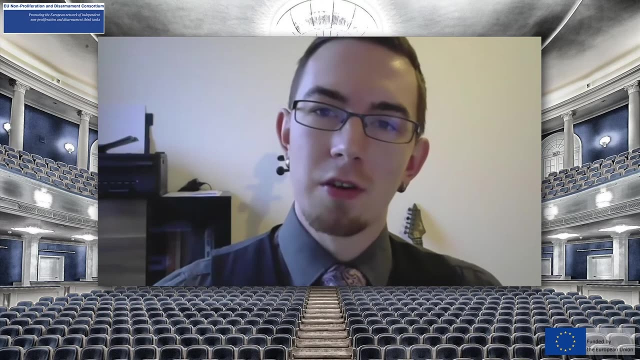 With that, I'll hand the microphone over to Noah. Thanks, Mike, and hello, and good morning, or good evening, early morning, to all of you, as is appropriate. First, before I get started, I would like to thank the EU. Nonproliferation and Disarmament. 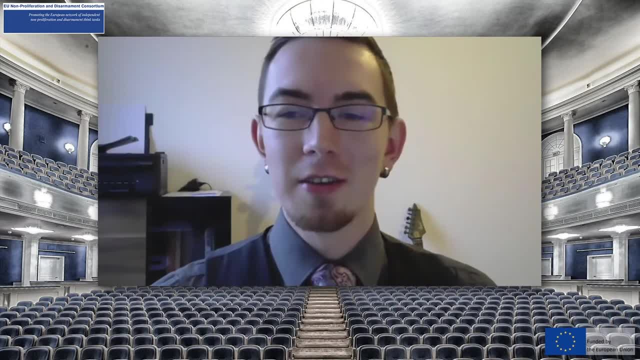 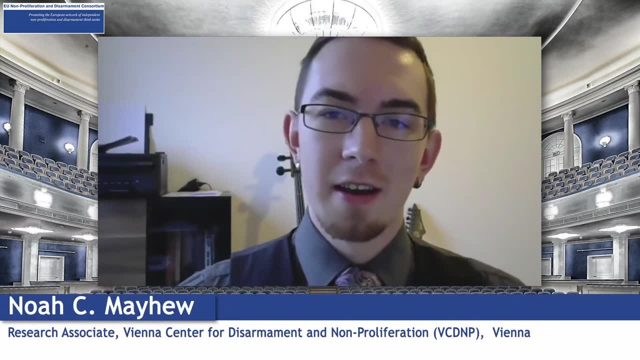 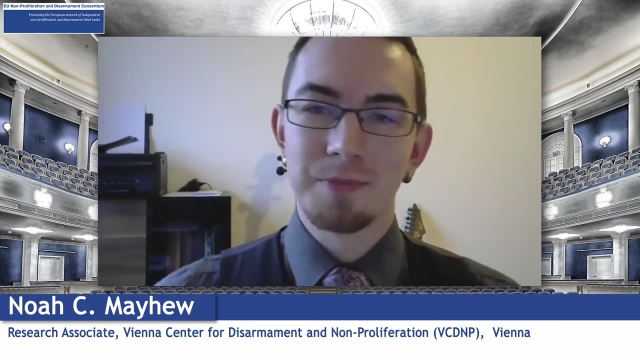 Consortium and the—I will try my Italian here—Istituto delle Internationale for the invitation to speak today, and particularly well done to the IAI for at least a composition of this panel, If I do say so myself, because, as Naomi, cast doubt onto whether or not arms control and 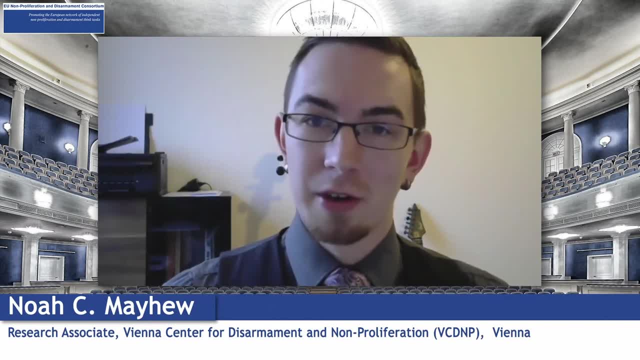 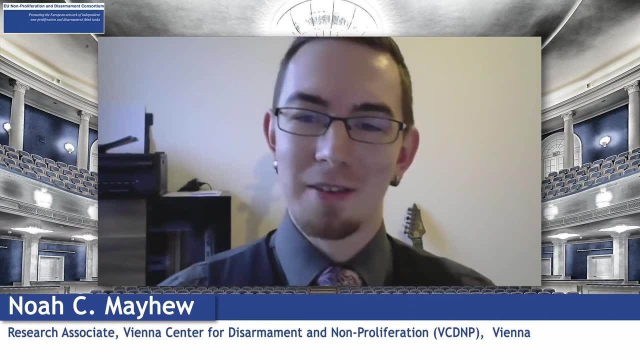 nonproliferation is crumbling as we know it, raising very fair and very important questions. I'm going to start my presentation with a very gloomy picture of where we're at. I'd like to talk about what it is we can hope to do with nuclear arms control as the arms 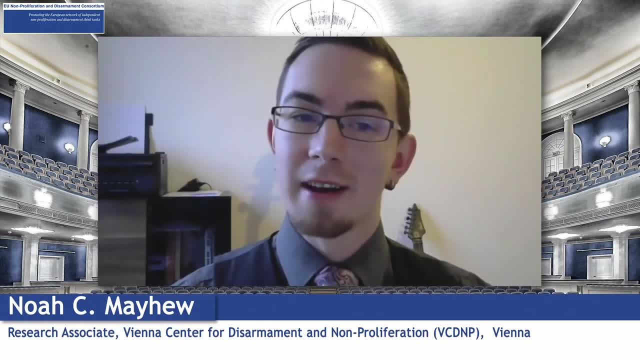 control architecture as we know it is in fact deteriorating in my view, Thank you In an unprecedented way, and Naomi outlined some of those ways. In the US-Russian context, one can certainly point to the outgoing US administration as 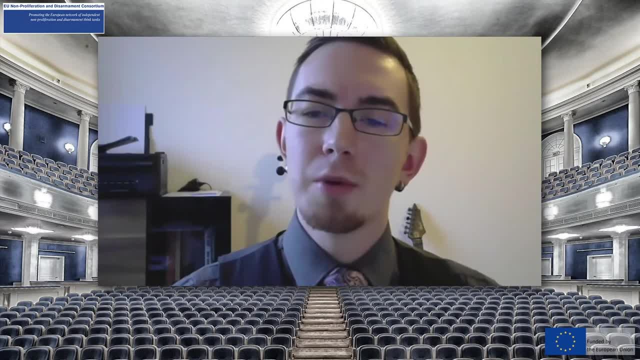 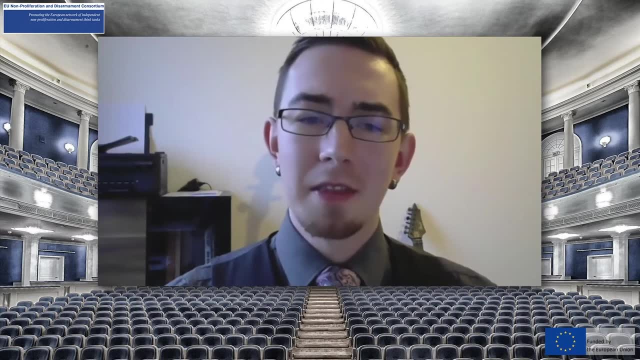 to why this is deteriorating, but in my view, President Trump's destructive policies towards arms control and nonproliferation were really more of a symptom of the problem than the problem itself. As I see it, the problem we face today is the disturbing decline in the priority that 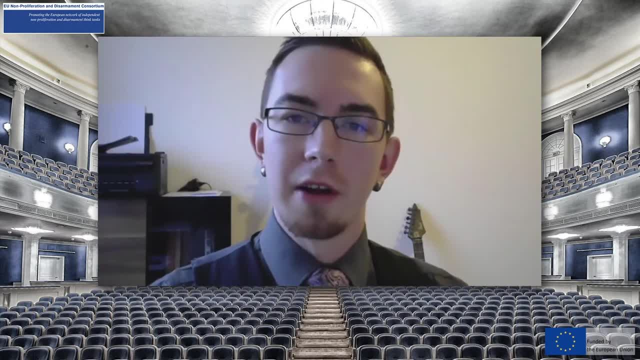 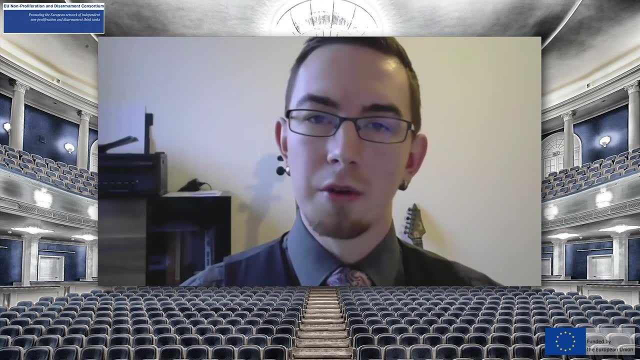 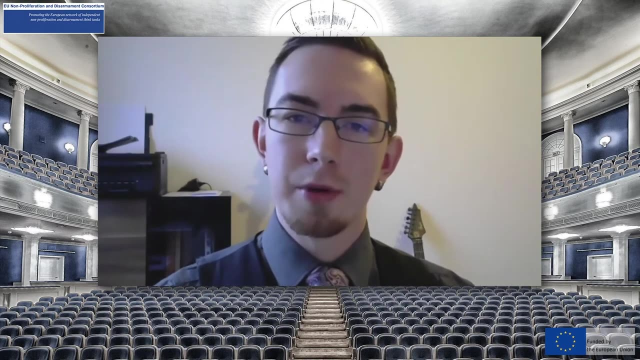 powerful nations seem to put on multilateralism and on multilateralism. As Mike said, I work in Vienna, home to many international organizations, including the International Atomic Energy Agency, where we've seen the so-called Vienna spirit, famous for putting compromise and cooperation above all else, decline sharply in at least the 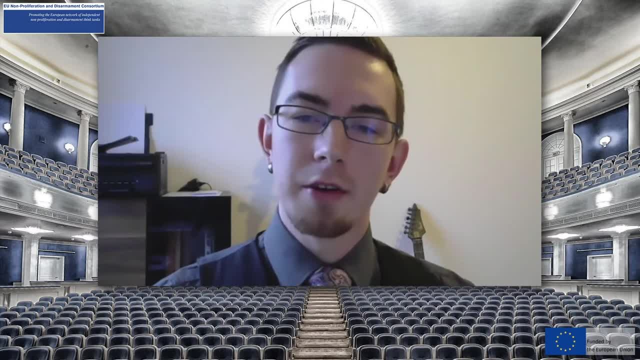 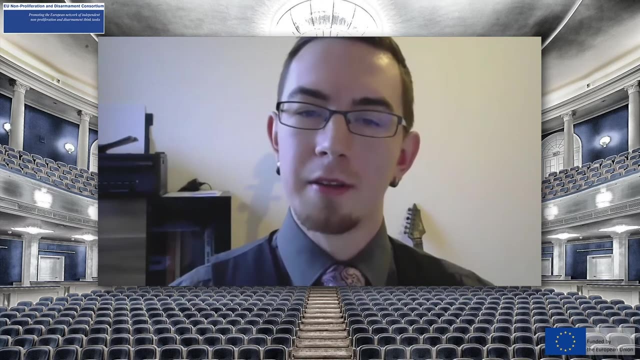 past decade, But I think the problem really dates back to the early 1990s, when the world order that we had grown so accustomed to during the Cold War was rapidly changing, was rapidly evolving. Of course, during the Cold War we got used to a bipolar world order, divided between 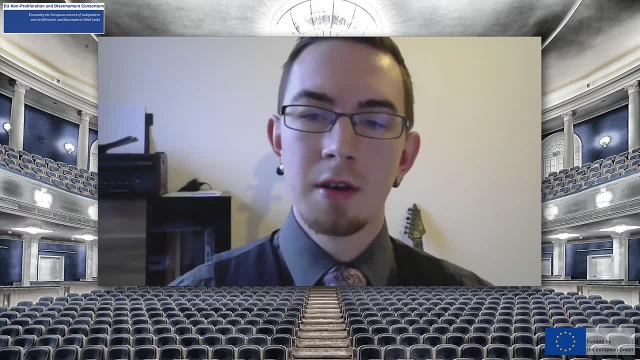 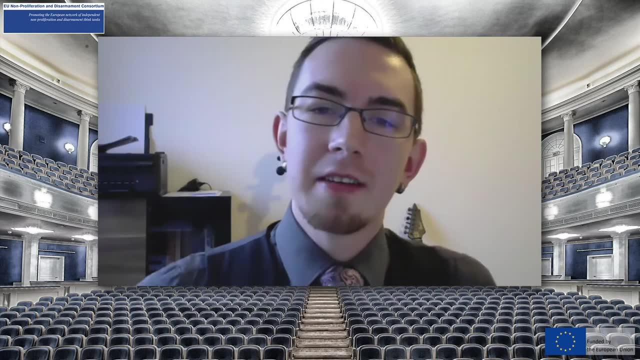 the influence of the United States and the influence of the Soviet Union. China at this time was, of course, not the economic powerhouse that it is today, But then, in the 1990s, the United States became accustomed to a unipolar world order, and I think in some respects the US is sort of stuck there, if only in mentality. But today we're in a multipolar world order where we don't just have the same kind of interests. We have to consider the interests of the US, Russia and indeed China, but also other powerful. 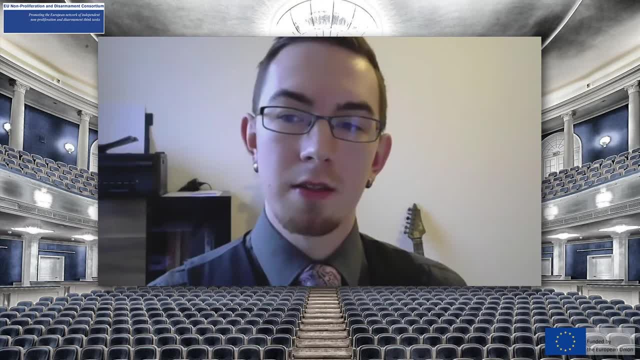 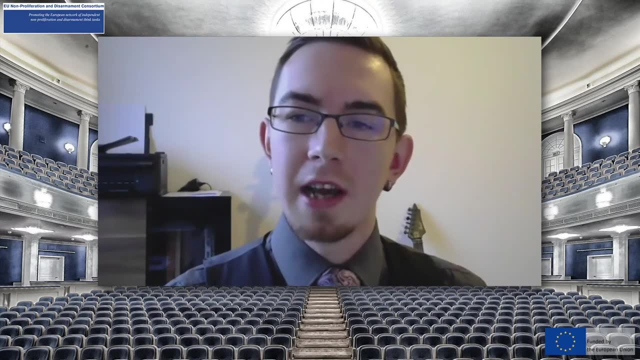 nations and groupings like the European Union, of course, and the group of 77, just to name two, And I think that failing to evolve our world view in alignment with the changing world order has led to some really faulty decision-making, especially in the area of arms control, and 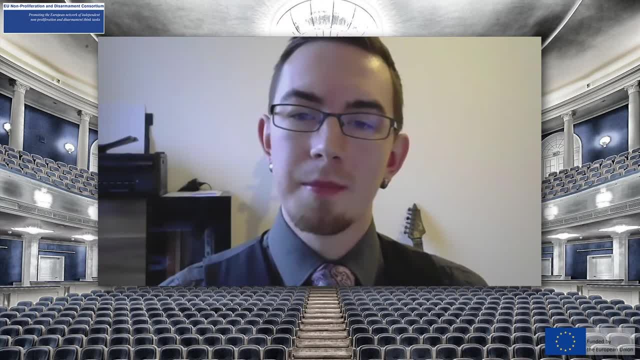 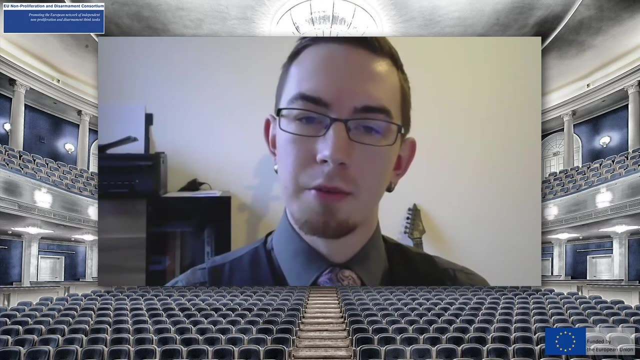 nonproliferation, where at one time the nuclear weapons arsenals were rapidly decreasing in numbers. And so we're faced with a situation in which not only is arms control as we know it changing, but the only arms control treaty left standing between the US and Russia will expire in. 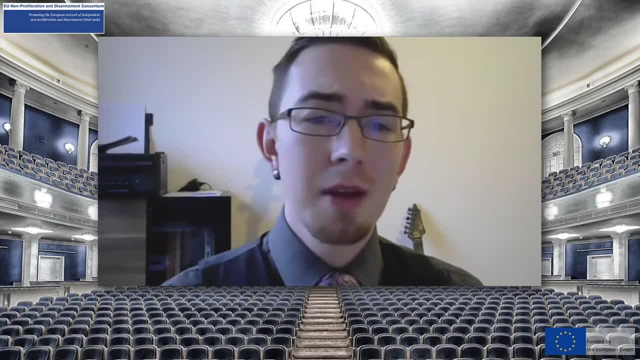 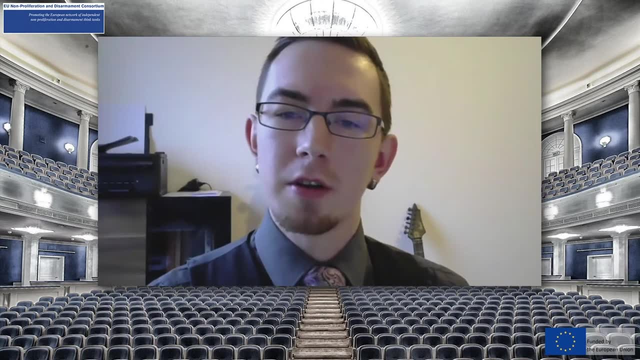 February of next year if it's not extended. And rather than recognize New START for its intrinsic value and predictability and transparency, the Trump administration has been caught in last-minute efforts to achieve an extension of the treaty on its terms. rather than extending the treaty as is and immediately beginning, 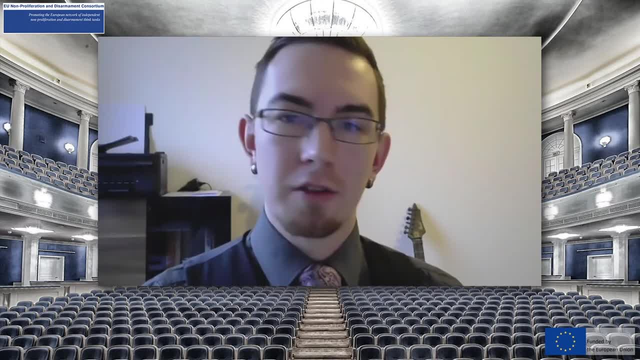 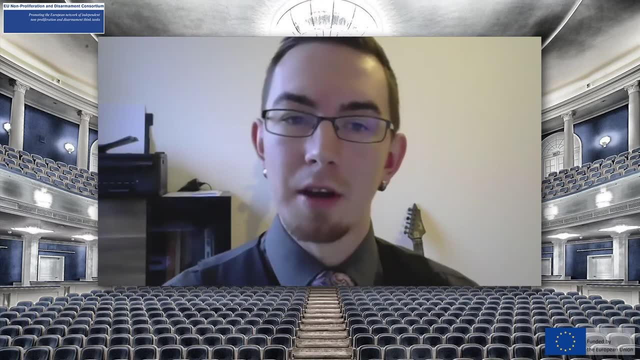 negotiations on a follow-on treaty. Now, there's a lot to unpack there, but you know, without diving too much further down that rabbit hole, let's talk about what can be done First. it's my sincere hope that the new administration in the US under Biden will move immediately. 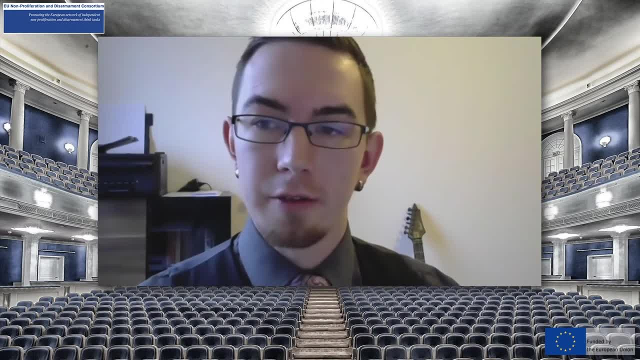 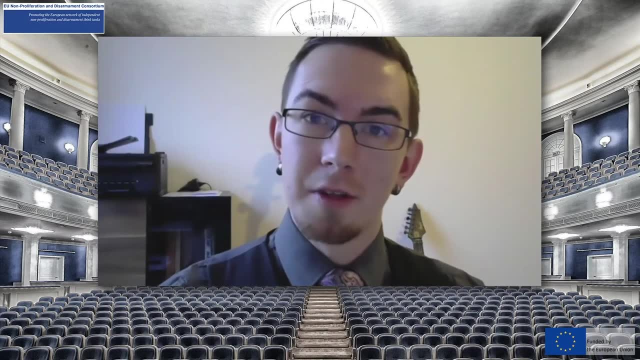 to extend New START when he's able to do so, and I would hope he's already in consultations about that with our Russian colleagues, as he's able. In this regard, I really hope that the slim margin between the US inauguration and the 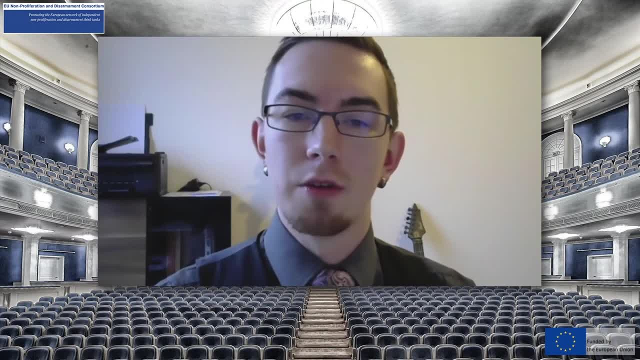 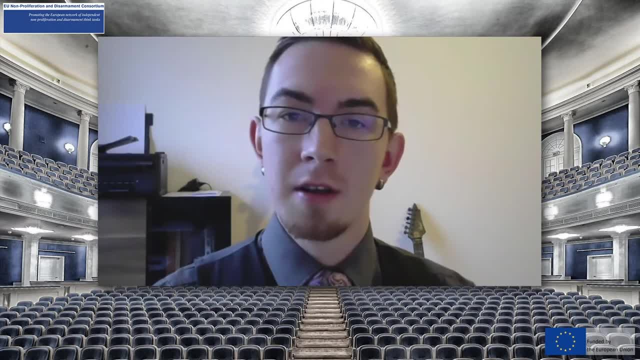 The next step is to extend that extension. to begin with, and we've added a couple of obligations, First of all, as a new authoritarian, the last of the talks will start on February 20.. And New START's expiration on February 5th will be enough. As Naomi observed, New START does not require congressional approval for the US to extend its exchange of letters to extend the treaty, but our Russian colleagues have indicated that the Russian Duma will need more time. I would also hope that President-elect Biden would move to start negotiations on that. 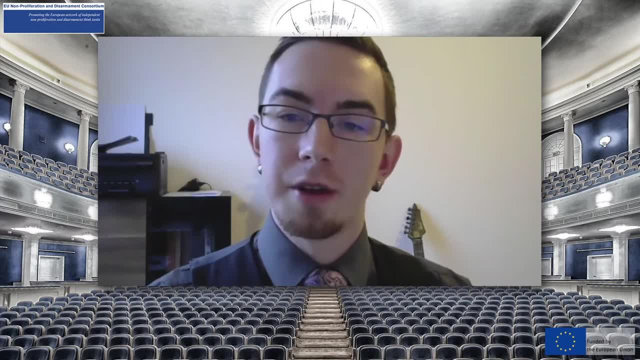 follow-on treaty to New START and to re-enter the Open Skies Treaty as another instrument that provides predictability and transparency not just to the US and to Russia, but also to our European colleagues. If New START is not extended, we will be left again for the first. 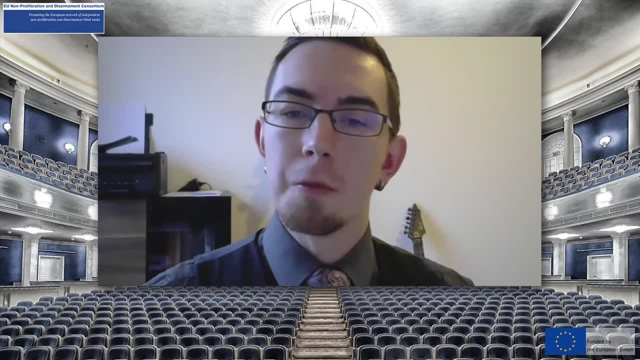 time since the height of the Cold War with no US-Russian arms control mechanism in force, And if this does happen, it could be taken as a sign that the nuclear powers, in particular the United States, are not interested in arms control anymore, And if this happens, other states are. 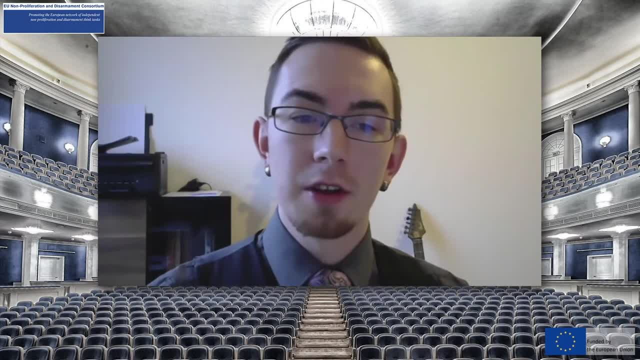 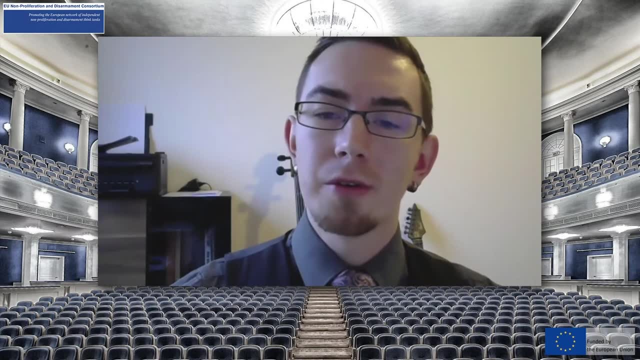 going to need to pick up the slack in new, creative ways And, in particular, Europe would need to champion the continued implementation of the Open Skies Treaty in the absence of the United States, but also throw some significant diplomatic energy into making sure that Russia also stays in. 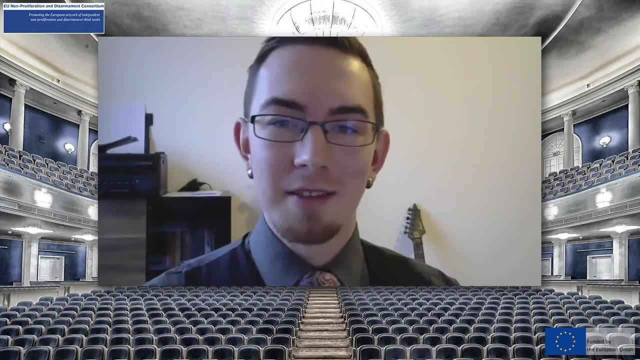 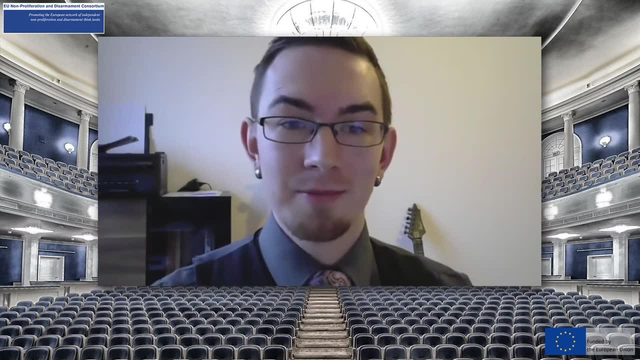 the treaty. You know, all of that doom and gloom aside, I'll choose to believe that for now, I'll choose to believe that New START, at the very least, will be extended And, given Biden's stated belief in the efficacy of multilateral diplomacy, 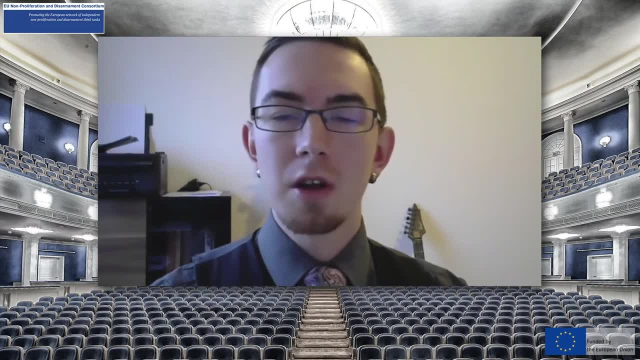 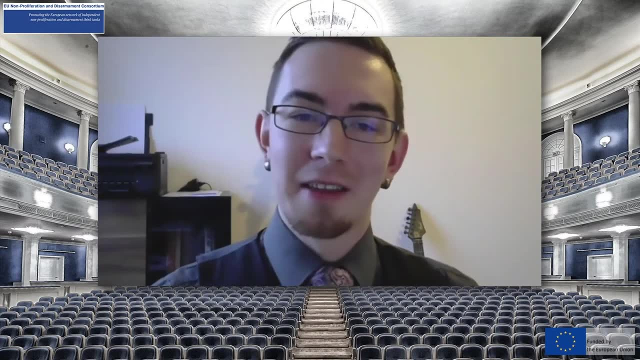 I would also think that he would start negotiations on a follow-on treaty, And the same goes for Open Skies reentry. There's also a lot to unpack there, but I want to touch on a couple of other things while I've still got time. 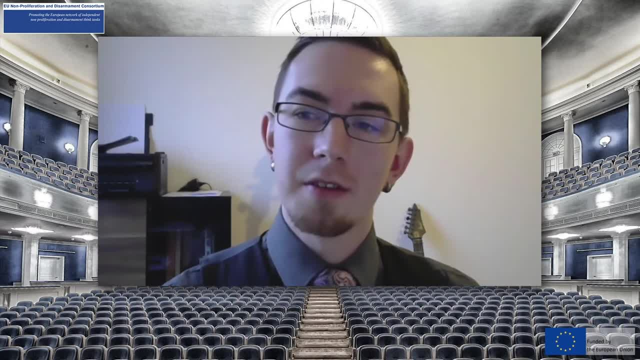 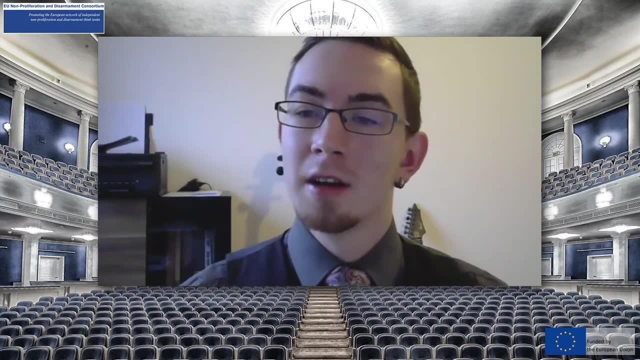 Another divisive issue that we face in today's environment is the Treaty on the Prohibition of Nuclear Weapons, the TPMW, which Naomi also touched on and Emily will talk about more extensively in a minute. It will enter into force on January 22nd of next year. Two days after the US inauguration- And I mention this here because of the unique situation that Europe faces with the US nuclear umbrella promised to protect NATO countries, on one hand, and the EU, which is not entirely composed of NATO countries, on the other hand. Of the European Union's 27 member states, 22 of those states are members of NATO, and not all NATO states are members of the European Union either, which includes, of course, Turkey that has American nuclear weapons posted on its soil. 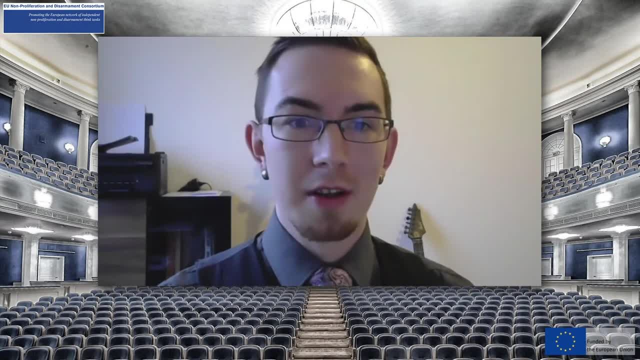 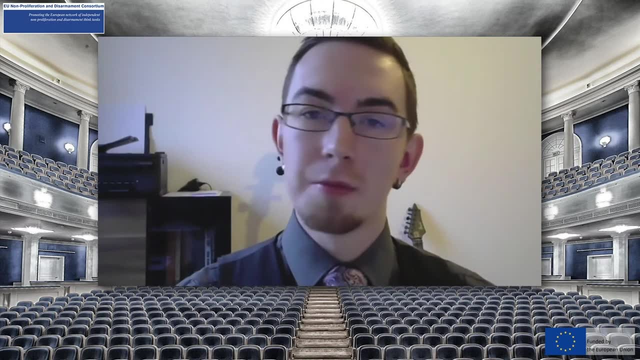 As the NPT nuclear weapons states continue to disregard and, in some cases, demean the TPMW. it's going to be very important for countries on the European continent- EU members, NATO members or not- where the division between the supporters and the proponents 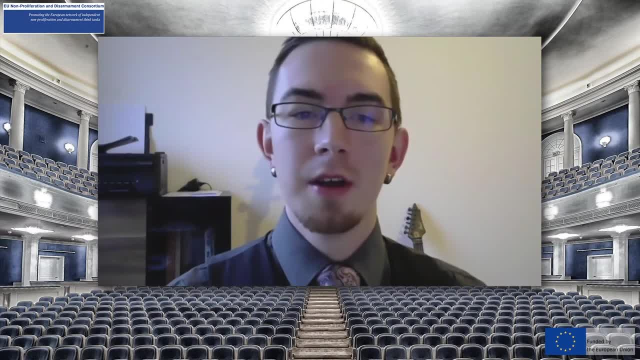 pardon me, the supporters and the opponents of the TPMW runs so deep to continue to be vocal and conduct active dialogue on the TPMW, And I think that's going to be a very important part of this discussion. and I think that's going to be a very important part of this discussion. 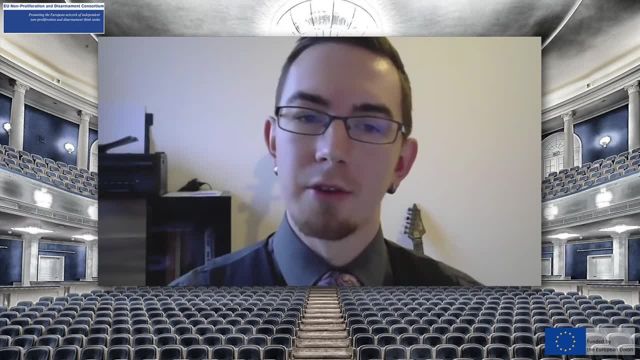 and I think that's going to be a very important part of this discussion- to prevent this divide from widening any further. Another issue that's become- for lack of a better term- fashionable in the non-proliferation sphere is new and emerging technologies with applications to the nuclear field. 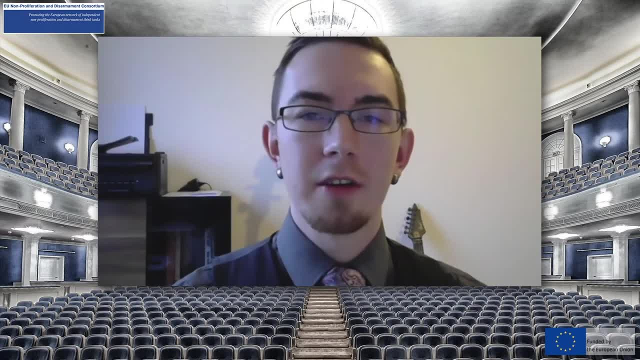 another thing that Mike mentioned in his opening remarks. Each of the technologies that falls under this sort of umbrella term, be it cyber, lethal autonomous weapon systems, advances in biotechnology, hypersonic glide vehicles and so on, really should be handled. 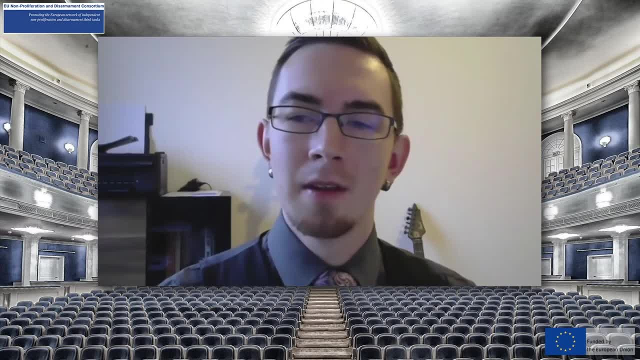 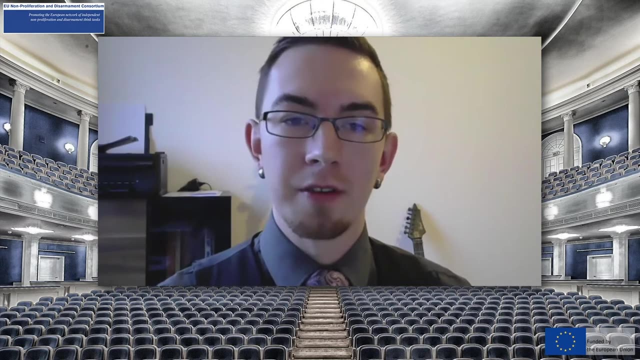 Differently from one another in my view. As a general point, I will add to the many voices calling for meaningful conversations on limiting the use of these technologies in the military sphere, to start now. But in the interest of time, I'll briefly touch upon the cyber issue as a matter of personal interest. 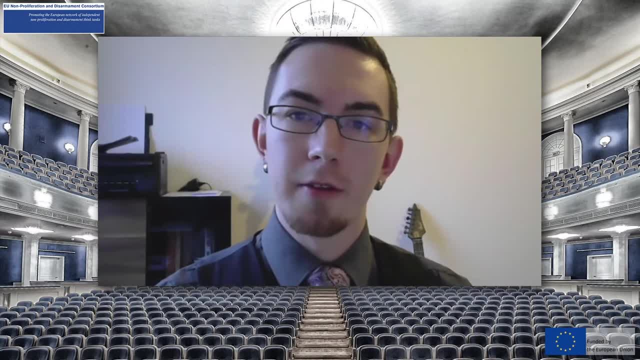 As many of you know, attempts to establish regulations for responsible behavior in cyberspace have been unsuccessful so far, And part of that is because a big part of that, I should say, is because the US and Russia cannot agree to the TPMW. 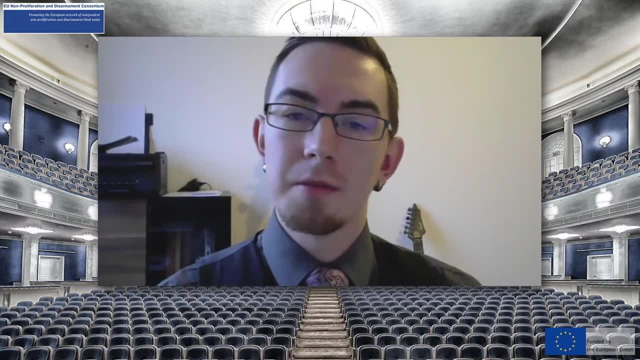 They cannot agree on how to define cyber warfare or on what basis a conversation about this should have, And while we're unlikely to see any sort of comprehensive, legally binding prohibition against the use of offensive cyber capabilities in the near future, I would really like to. 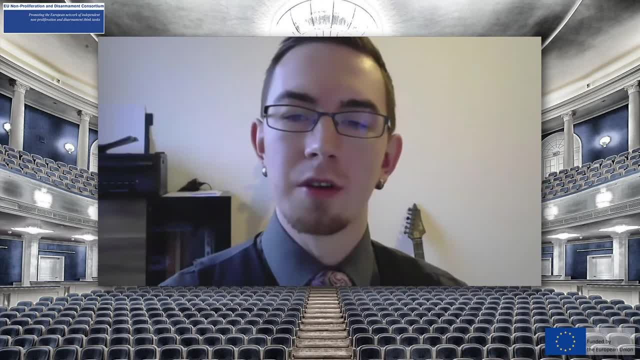 see a serious discussion about at least a political declaration not to use cyber capabilities against nuclear facilities and nuclear command, control and communications systems. We see this as a very important issue. We see some parts of this debate playing out in the UN context right now. 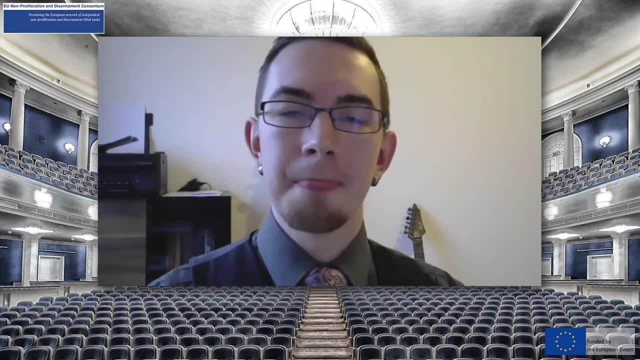 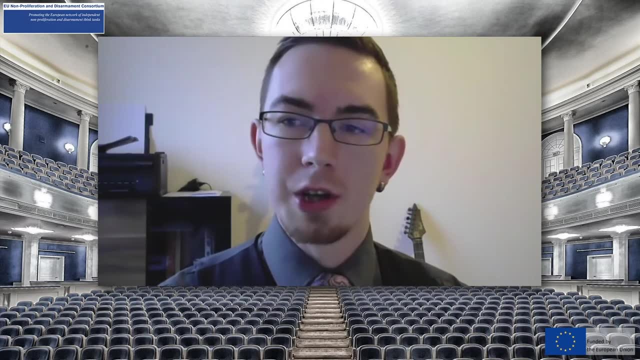 And I would love if such a political declaration could also include a prohibition against what I find to be the very frightening prospect of a cyber, so-called left-of-launch operation in the ballistic missile defense field, which I'll be happy to comment further about during the Q&A. 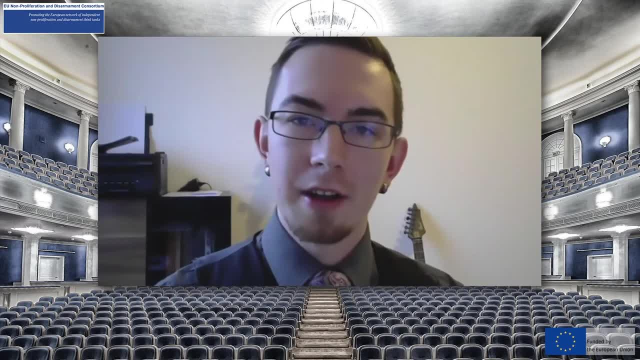 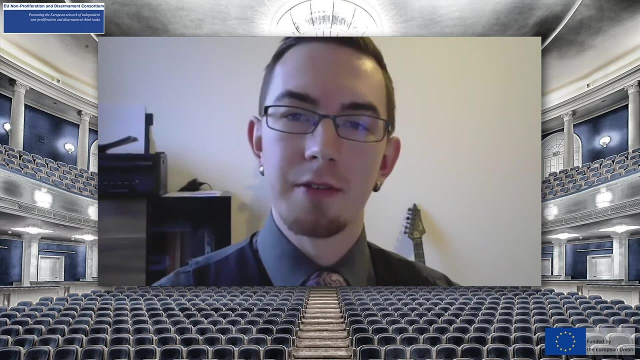 But again, in the interest of time, I can't cover the entire landscape of my concerns in the political and technological channels. I know there are many challenges we face today, but I hope I've outlined two broad points. First of all, we- all of us- need to be prepared to update our understanding of the geopolitical 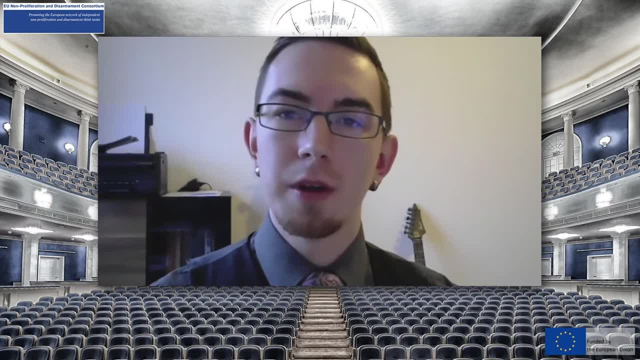 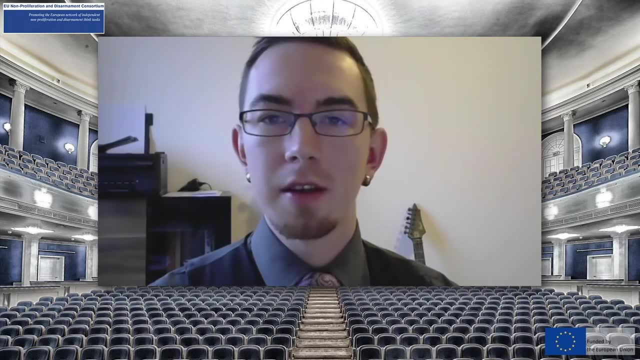 realities that affect nonproliferation and arms control, as well as the weight that individual states' interests have on the feasibility of reaching new arms control agreements and indeed on the health of the nonproliferation regime at large. And second, new and emerging technologies are not a monolith. 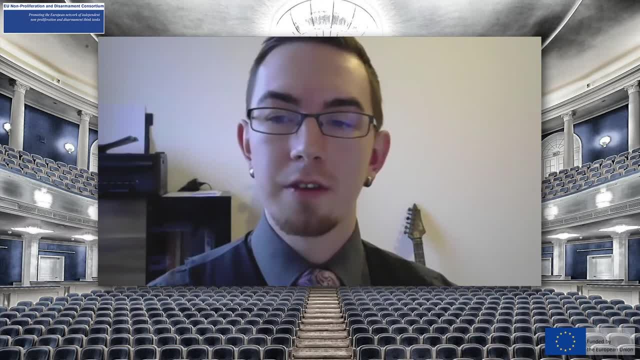 One, of course, that causes me the most concern for the nuclear field is cyber, but hypersonic glide vehicles and lethal autonomous weapon systems carry their own set of unique challenges. So, in closing, I have a few recommendations I'd like us to consider. 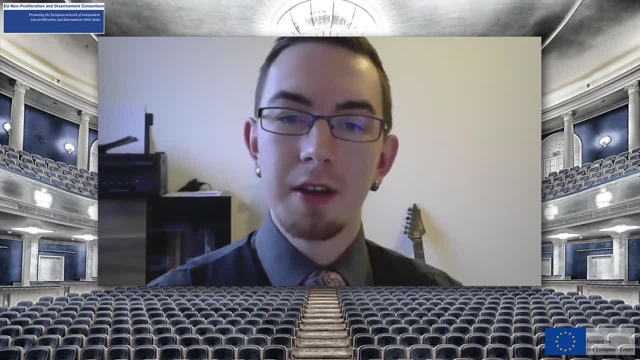 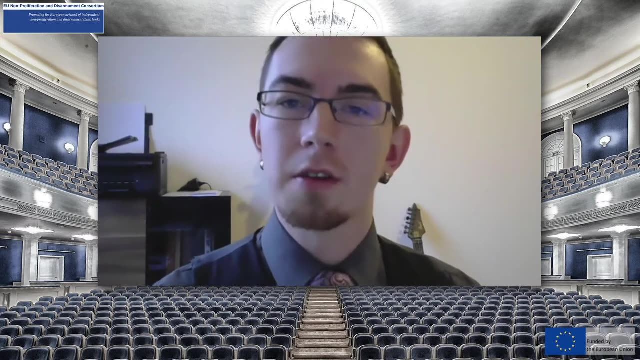 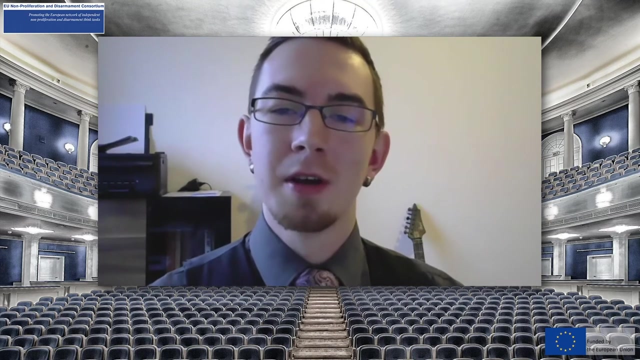 The first one, in the tech field, we need to remember the value of multi-stakeholder engagement, especially with emerging technologies. This means meaningful engagement between the private sector, the technology developers, the civil society and the public sector. And the second: in the tech field, we need to consider the value of multi-stakeholder engagement, especially with emerging technologies such as the. 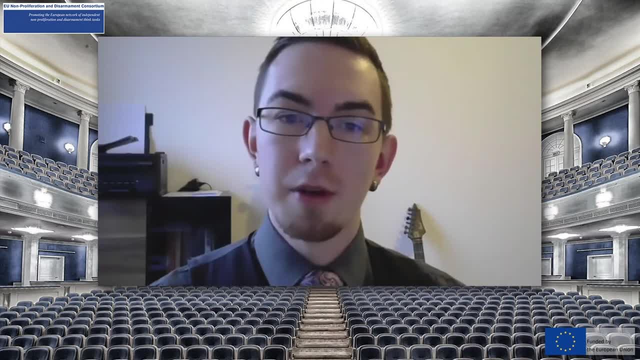 international civil services, government officials, military representatives and so on, And in this vein, I could dream of- if only a dream- a convention on state behavior in cyberspace or something similar to that effect, And this, of course, would require the US and Russia to at least agree in talks on how to talk about cyber issues in an effective manner and in a multilateral format. 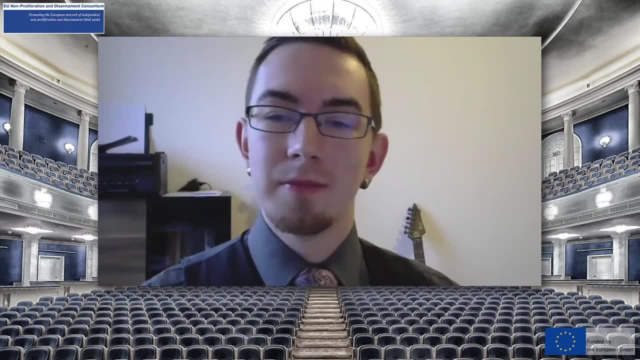 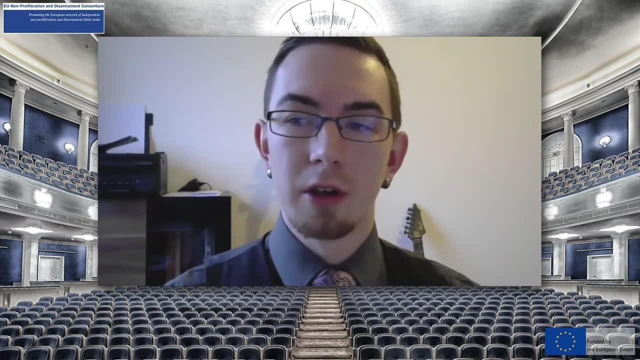 This certainly would not be a simple endeavor. a simple endeavor, Verification would be a nightmare. But the more I see cyber evolve, the more convinced I am that developments in cyberspace with no prohibitions of even a political nature, particularly on the nuclear applications that I mentioned a moment ago. 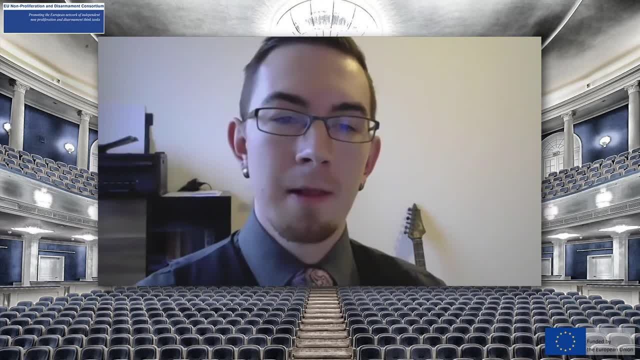 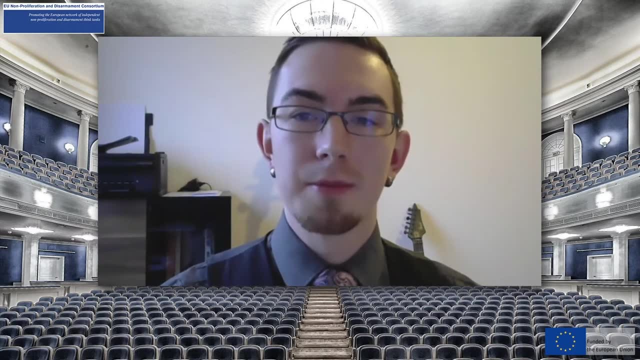 is becoming very, very dangerous. Second, multi-stakeholder engagement, in the political sphere as well, is something I'd like us to try and promote as much as possible, And this would mean us returning to a priority placed on multilateral diplomacy and a reassessment going in of what each 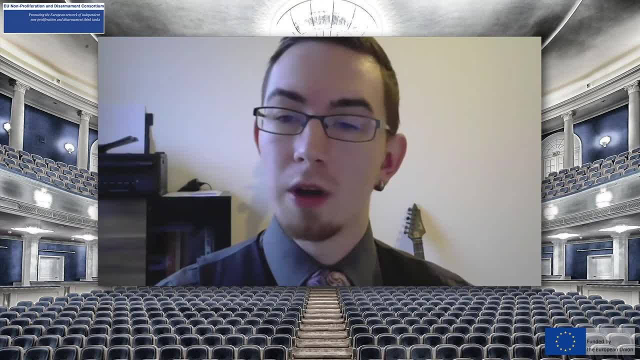 other's strategic interests really are. While with many of these things, it'll take some creative thinking to achieve this, it's not as though we don't have any examples to draw from on this. A follow-on treaty, for example, to the New START treaty, could build on the 2010 model itself. 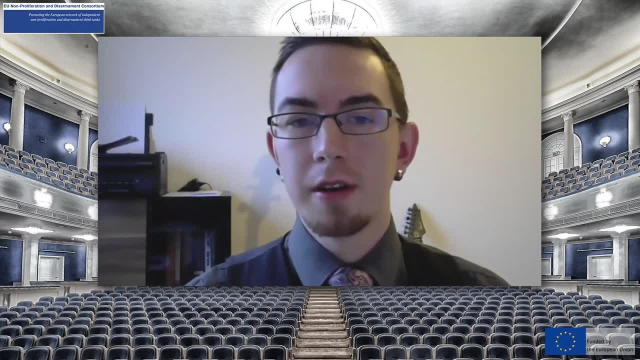 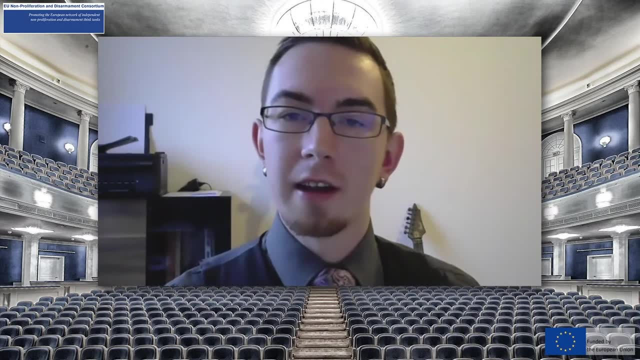 and the negotiators could seek to address areas where the treaty needs to grow to today's conditions, And this includes new and emerging technologies and perhaps important geopolitical players like China. I know I'm just about over time, but responding to something that both Mike and 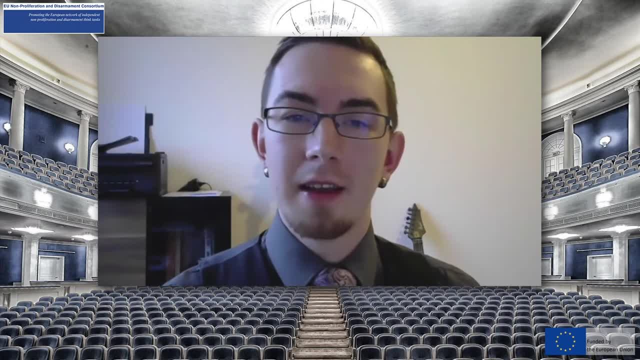 Naomi pointed out, it is my strong sense that a follow-on treaty to New START should at least consider using ceilings for numbers rather than numbers and reductions. In other words, if we want China to come to the table in addition to figuring out the transparency. and verification aspects. it may be much more attractive to say: the parties to this treaty have maximum X number of nuclear weapons and Y number of basic kinds of basing modes and that sort of thing, rather than reduced by X amount. But outside the US-Russia-China context we could also seek to revive old models like the: 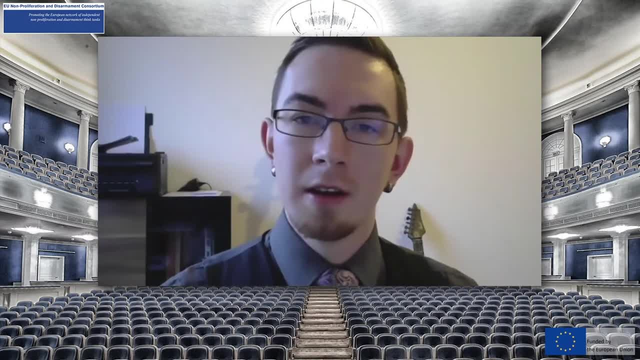 model of the Nuclear Security Summits also mentioned by Naomi, And if championed by a large enough country or group of countries. imagine if something like what the Nuclear Security Summit did for Nuclear Security could be done for another field, or even just a Nuclear Security Summit's. 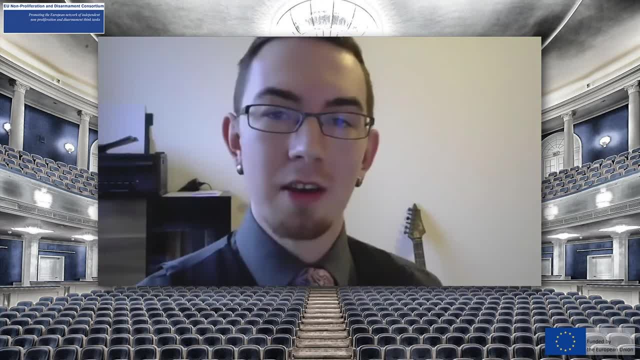 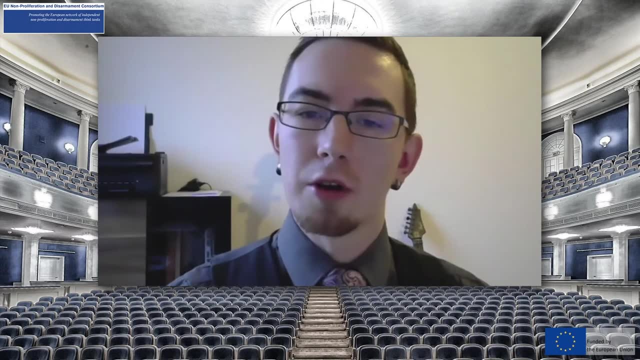 round 2.0.. Third and finally, in the absence of such engagement and such sort of tangible progress, a lot of people talk about norms, for example, against the deployment of missiles in Europe or destructive behavior in cyberspace, And some people talk about norms in a sort of 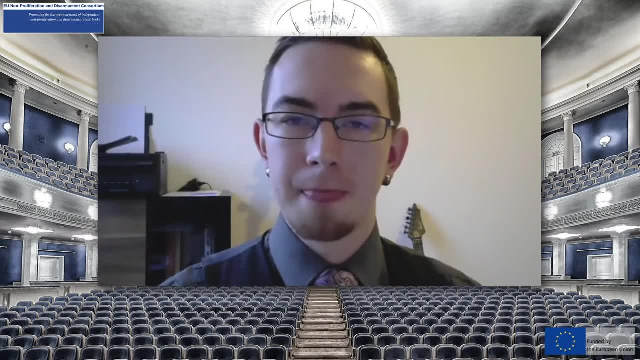 denigrating way, and others talk about norms in a sort of denigrating way. And some people talk about norms in a sort of denigrating way and others talk about norms in a sort of denigrating way, As if they're exactly what we need to be doing. I want to point out that there's nothing. 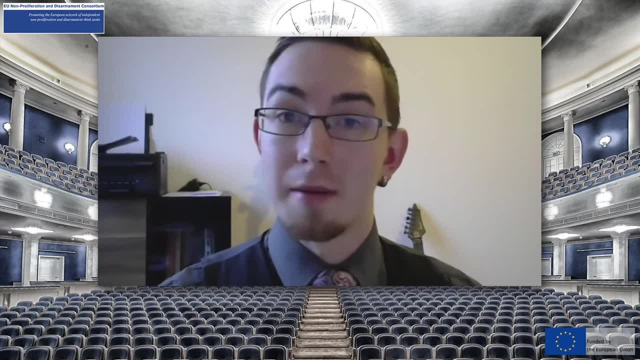 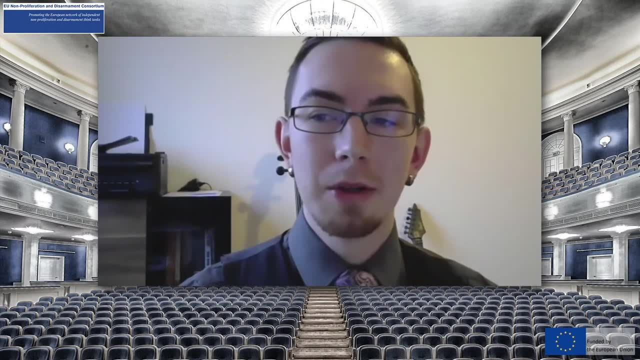 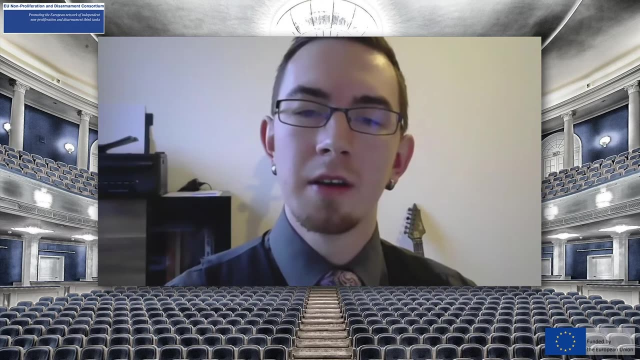 contradictory between norm building and arms control at all- in my view anyway- But also that, in the absence of real progress and momentum, norms can be building blocks to legally binding treaties. And that doesn't mean that talking about norms will automatically just bring treaties into being. It means that as we talk about norms we should focus the conversation. 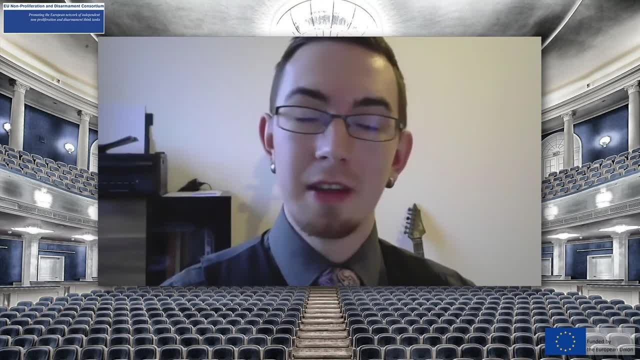 on these tangible outcomes And the TC P and W- be you a supporter or not so much a supporter- is an example where exactly this happened. So I'm quite sure I'm over time. Thank you very much. I look forward to your questions. 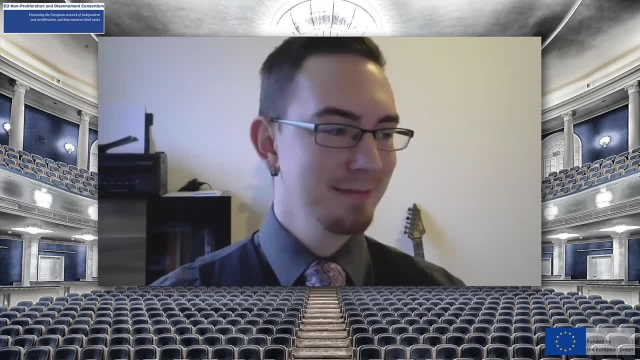 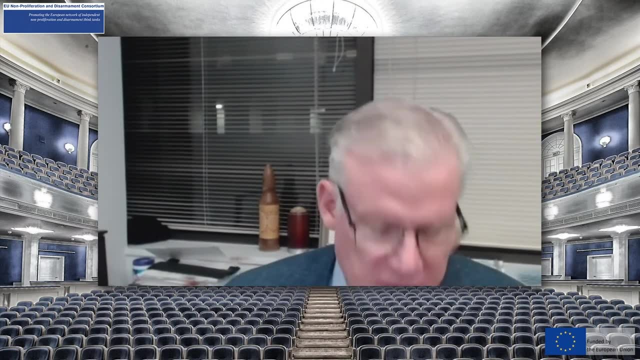 And back to you, Mike Noah. thank you very much. I think you put a lot of food for thought on the table And I look forward to posing some questions I have from your presentation Which I really, really enjoyed. Next, I want to turn to Emily. Forgive me if I pronounce this. 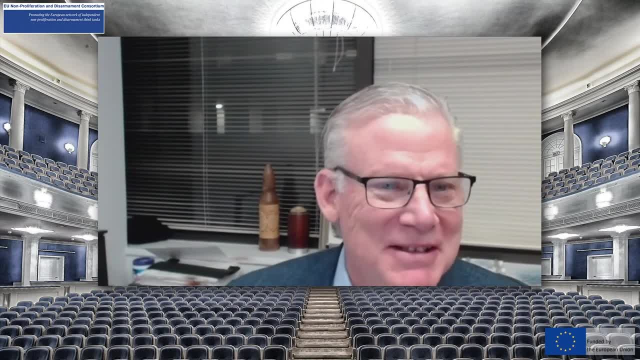 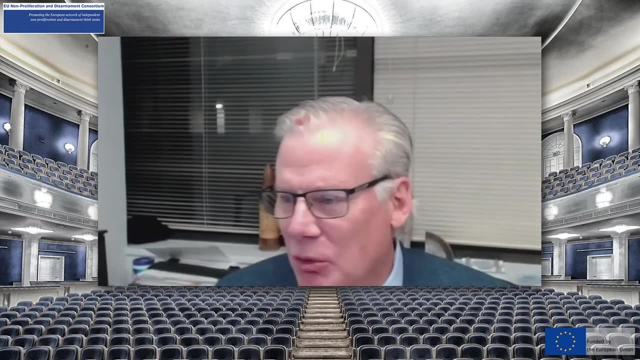 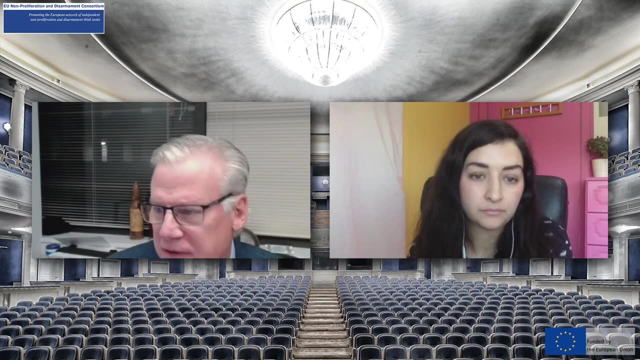 improperly. Is that correct? Okay, Even a squirrel finds the nut once in a while. Emily currently works at the disarmament nonproliferation unit at the Department of Foreign Affairs in Ireland, where she focuses primarily on nuclear and related issues. 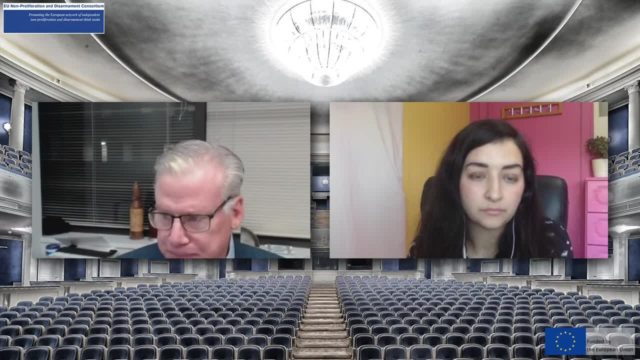 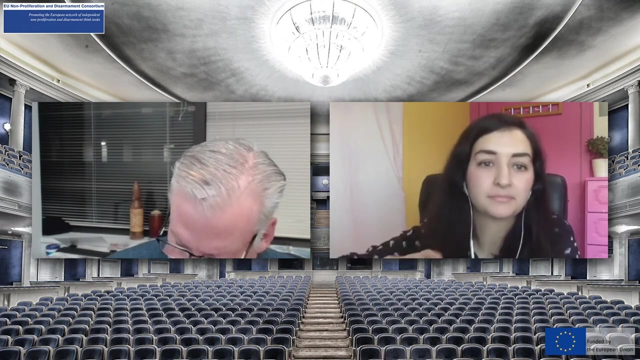 She's previously worked for a number of NGOs on issues of political dialogue, armed conflict and international justice. among other things, She is a lawyer and is admitted to the New York State Bar as an attorney at law. Congratulations, Emily. I look forward to your presentation And I would like to hand the microphone over. 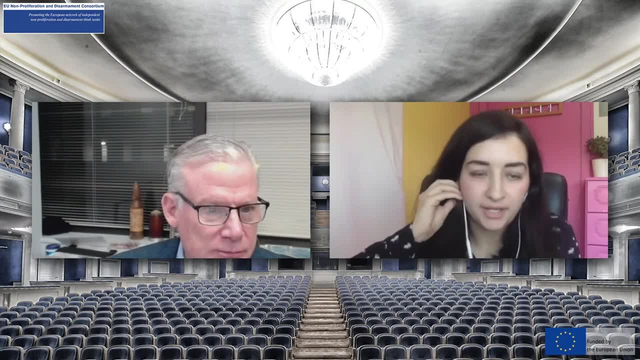 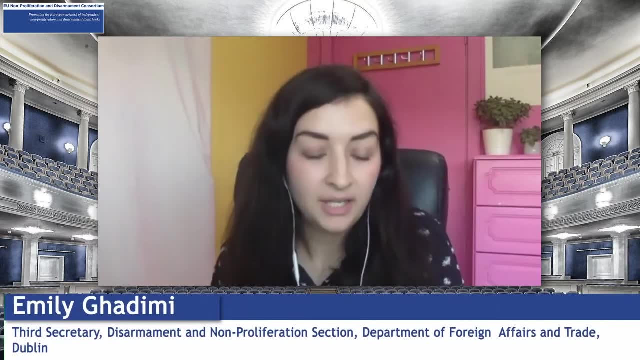 to you at this point. Thank you, Thanks so much, Mike, And thank you so much, Emily, And thank you again. I'll just reiterate the thanks to the organizers for the opportunity to join this panel and to share some of my own views, as Noah and Naomi have mentioned. 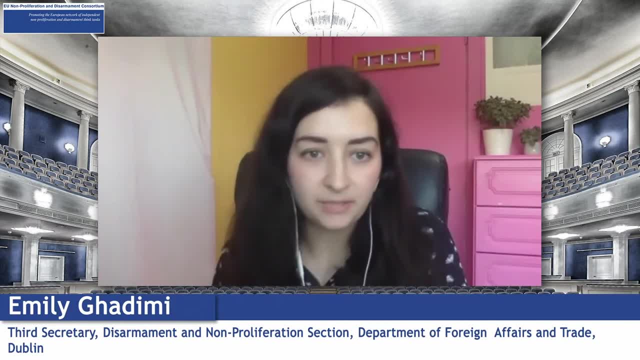 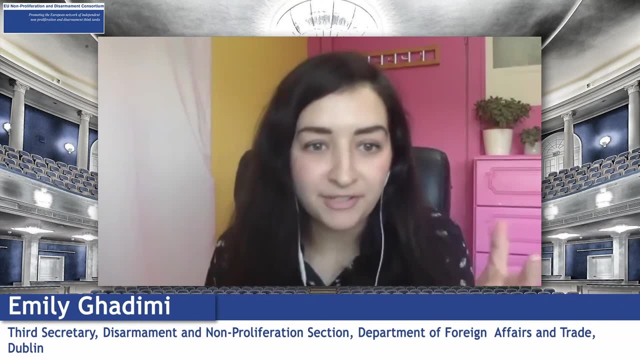 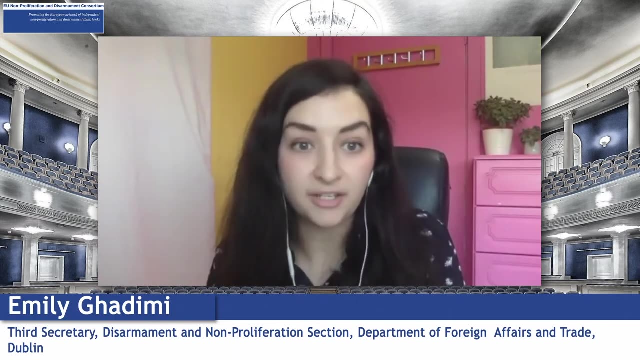 on the TPNW. So I just want to speak a little bit about that And, as Naomi and Noah have outlined excellently, there's obviously a bit of disagreement on whether we are in an era of crumbling treaties or not, But I think we're in a—certainly a sort of challenge. 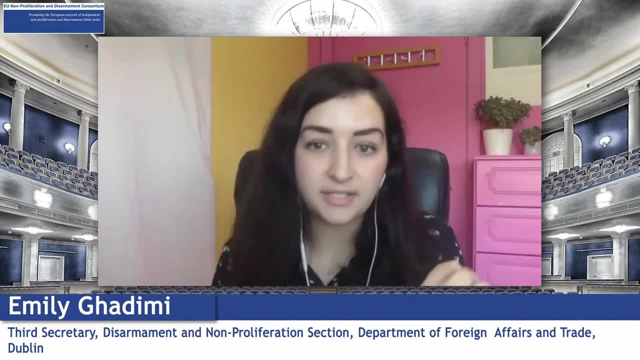 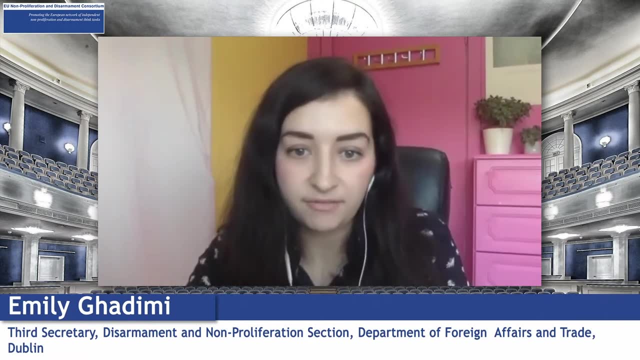 in time, But I think in this context, the TPNW has actually been an exception. It's gained rapid support since it was first adopted in 2017.. Both panelists have also alluded to the criticisms and that it has very vocal critics, But it does have the support of the 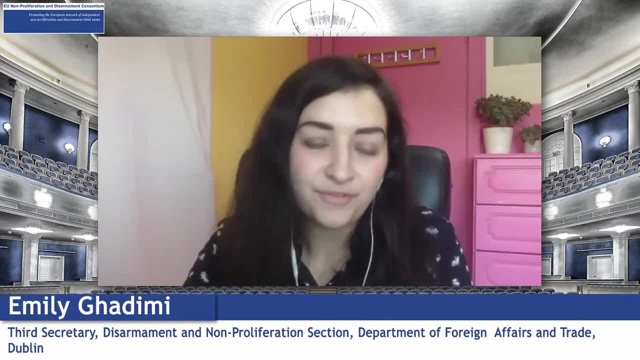 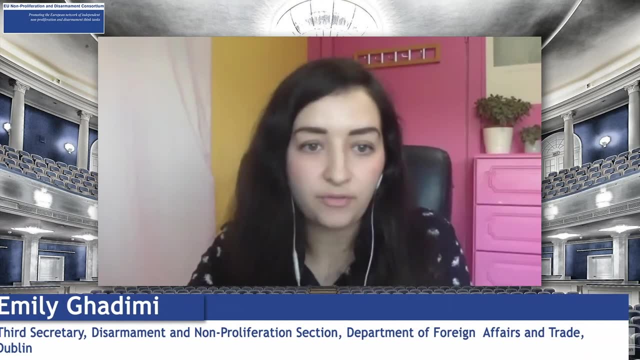 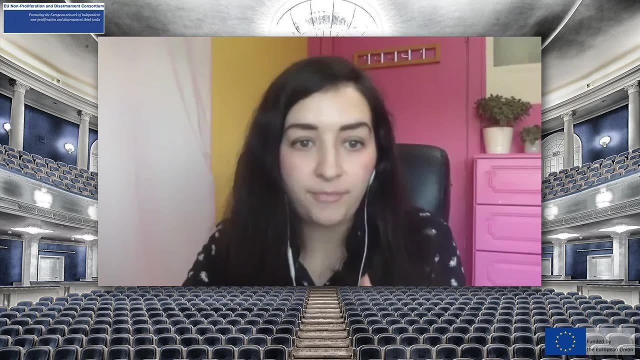 majority of states, including Ireland, which ratified the treaty on the 6th of August this year. So I just want to touch on three different issues, Or three different aspects of it today. Firstly, just some lessons that might be taken from the approach of the TPNW negotiations. A bit of an outline from my view of the context. 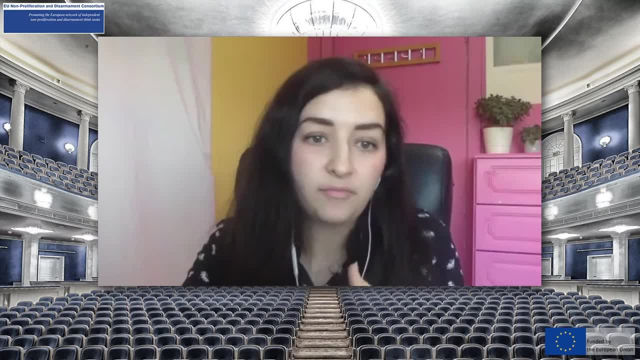 that led to the treaty, And then some—I would say speculation maybe—but some ideas about the potential impact of the imminent entry into force, including on the NPT. So firstly— Secondly, on the negotiations: they were particularly distinctive in this area, for 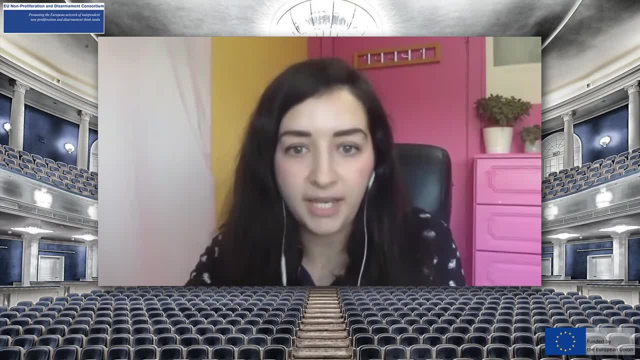 a number of reasons. There was diverse engagement from voices that aren't traditionally heard in disarmament spaces, from developing countries, from small island states, survivors of nuclear weapons testing and from the Hibakusha. It was also notable how many women were active in the proceedings, which I can say is a start. 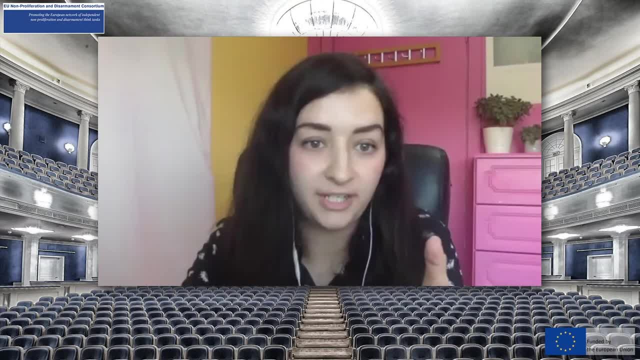 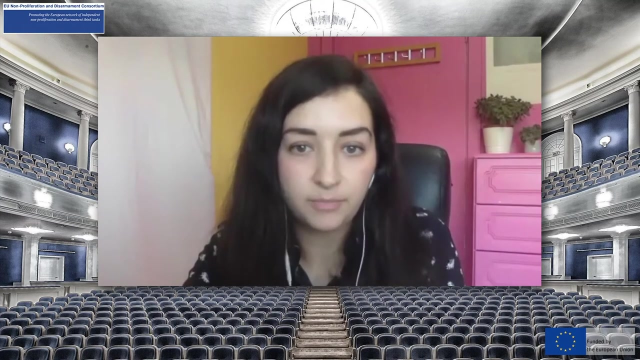 contrast to what we'd usually see- although thankfully we're seeing more sessions like this with a strong female component- But the personal interventions from people who had direct experience of nuclear weapons use and testing had a really significant impact and greatly contributed to the innovative provisions that were ultimately included in the treaty. On the point of inclusivity, it's also worth noting that there's a result of such a large number of women that were involved in the treaty and also involved in the process of the negotiations. There were times when it was a case of the treaty being overlooked. 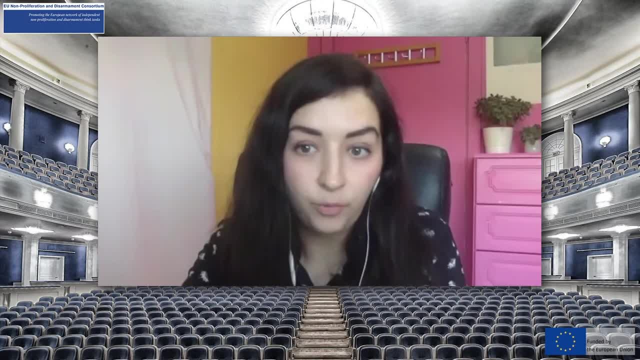 and that's not the case. otherwise, if we look at the outcome, it's still a bit confusing, But it's a fair example of the impact that would be reflected in the results of the negotiations. also worth noting that the negotiations were open to states and others who were opposed. 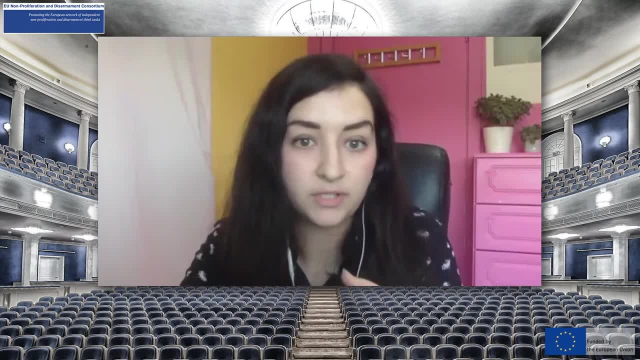 to the treaty and I think it was unfortunate that many chose not to participate. I see the TPNW as a tangible example of the human-centred view of nuclear disarmament really put into practice. It gives a vision beyond the traditional frameworks of negotiation. 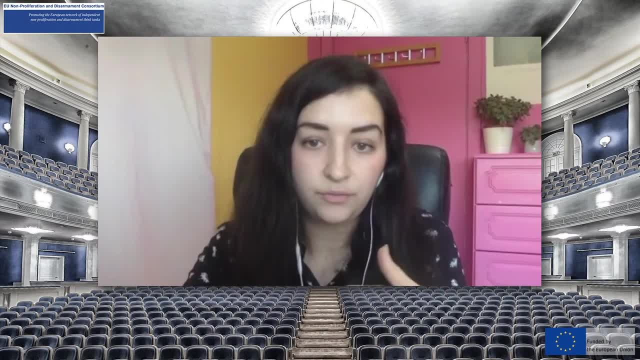 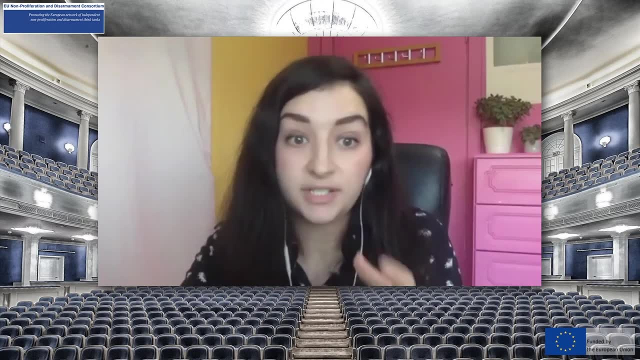 These are often at a high political level and don't necessarily include a broader range of voices or stakeholders. But that said, the humanitarian view of nuclear disarmament is not new. It has its roots in the origins of the NPT. It has its roots in Irish foreign. 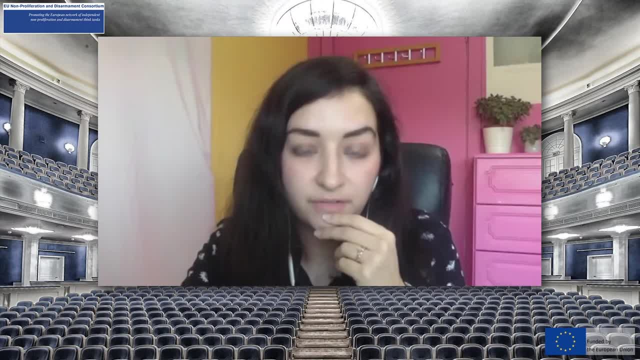 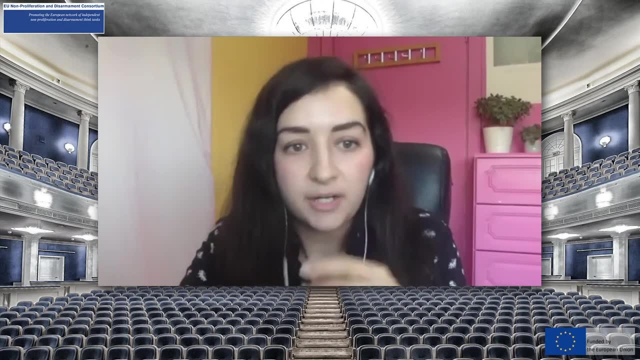 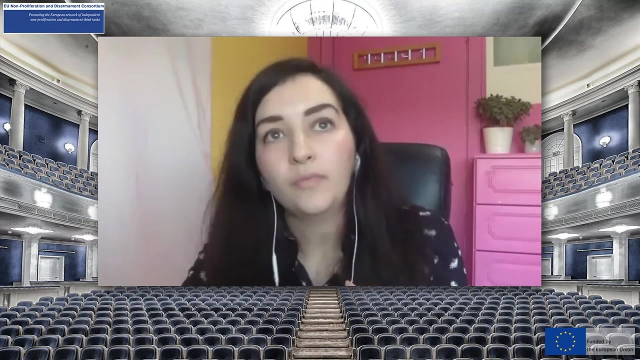 policy from the early days of the UN. That was something that was put forward by Ireland at the time And it was very much a realisation of…. It was a concern shared by a lot of states about the real existential threat posed by nuclear weapons, posed by the proliferation of nuclear weapons, to humanity and the planet. 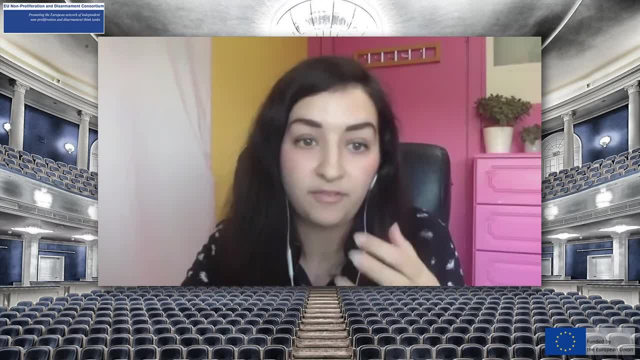 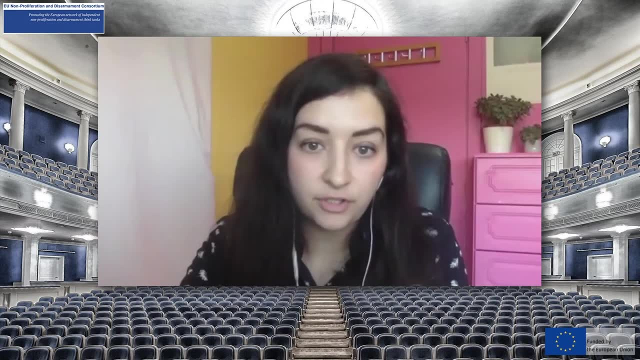 And of course, the critics of the TPNW have been very vocal about the myriad problems that it's going to pose: That it doesn't take account of the security environment, that it's not compatible with the NPT framework or that it might actually undermine the NPT. 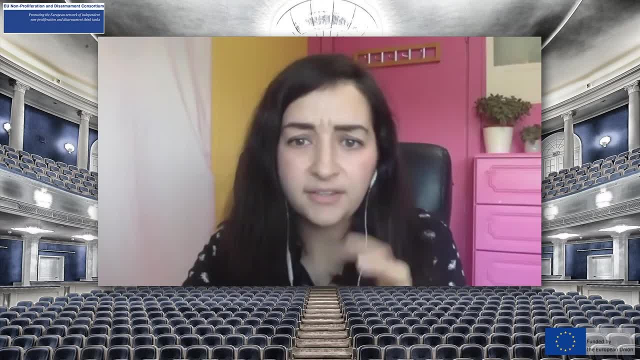 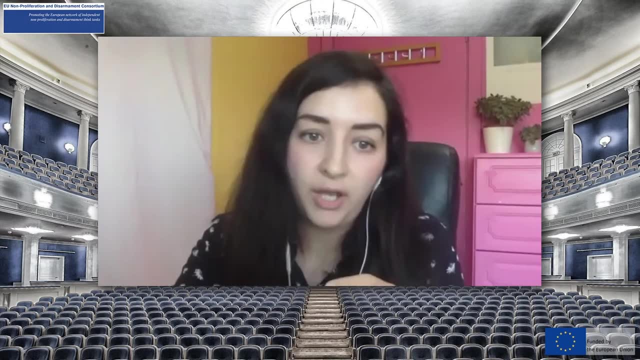 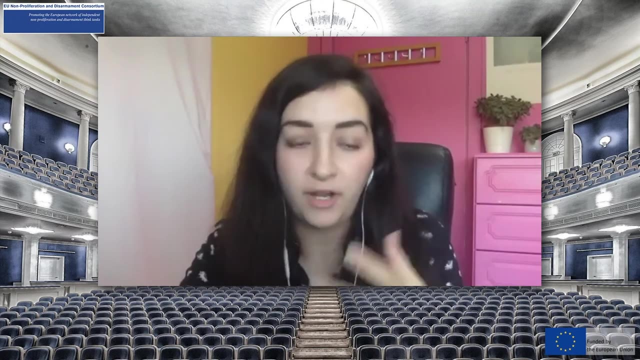 and other non-NPT, And I think there's a number of elements within this which I just want to explore a little further. I think it's important to look at the environment that the TPNW grew from. Mike, you alluded to following at the end of the Cold War and in the decades following, there wasn't really. 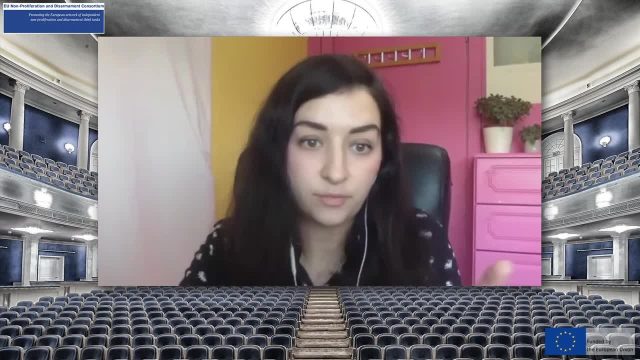 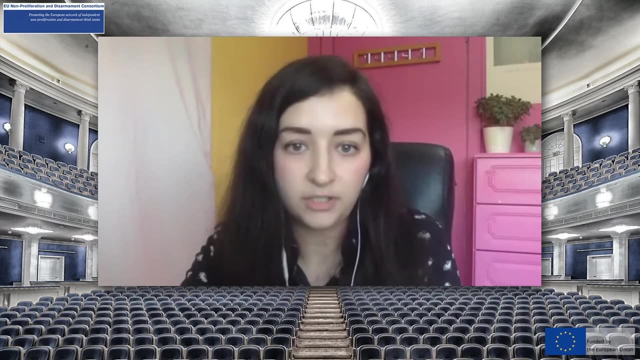 much progress made on nuclear disarmament And actually the trend was starting to go the other way, with greater modernisation, increased investment And at the same time we also saw a very concerning deterioration in the security dynamics in a lot of situations around the world. The causes of which are deeply complex, interlinked, far too detailed to go into in this context, But just suffice to say there's a growing mistrust, particularly between nuclear powers, an increase in geopolitical rivalries, all of which have bled into multilateral disarmament. 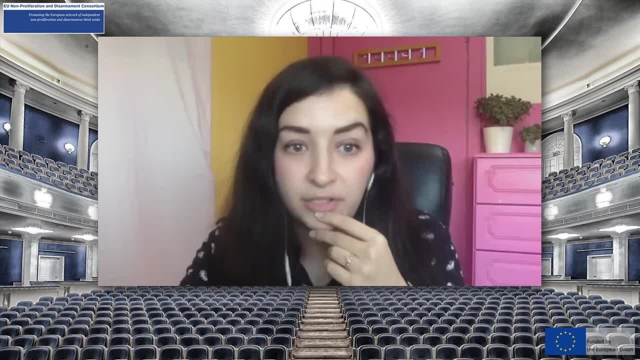 And Noah also mentioned this- even the Vienna spirit that was, you know, about consensus building, and all of this has- we've seen it- come under strain, And we've seen this, of course, in particular with the dismantling of the agreements between 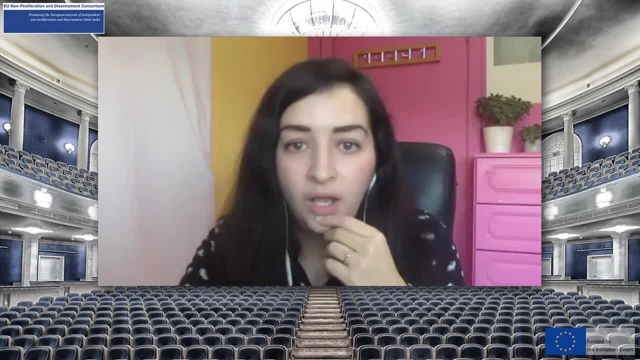 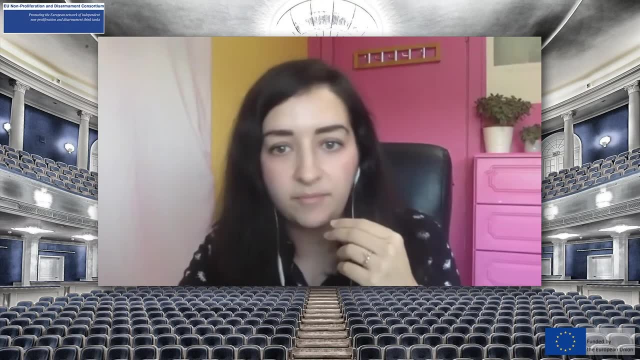 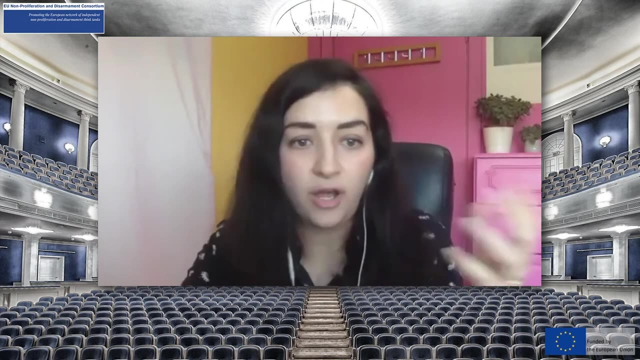 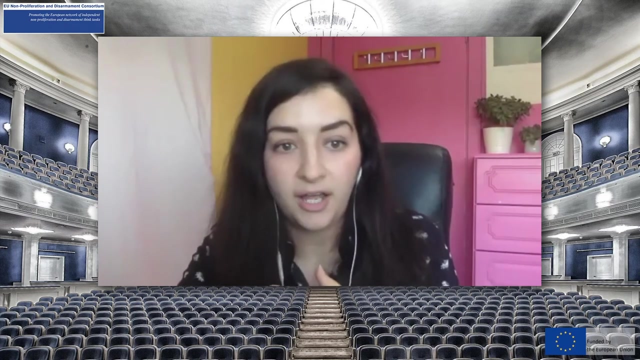 the two largest nuclear powers. And one obstacle I see in this area is the way that competing positions seem to be presented, That they're somehow put forward as this dichotomy, on the one hand, between naive and idealistic TPNW evangelists and, on the other hand, nuclear powers that are coldly indifferent to the 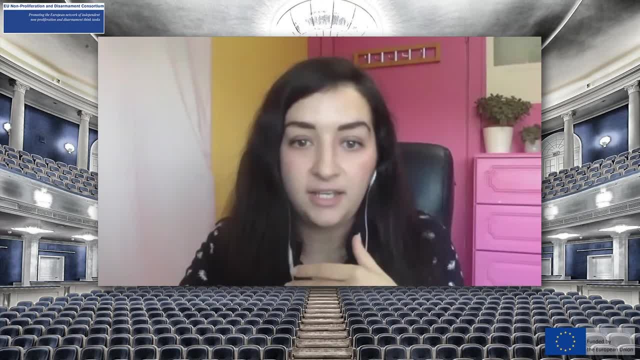 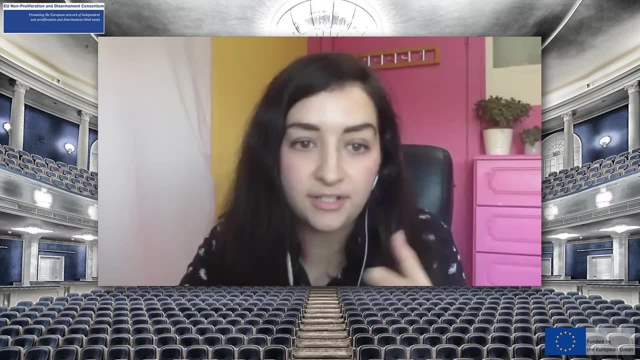 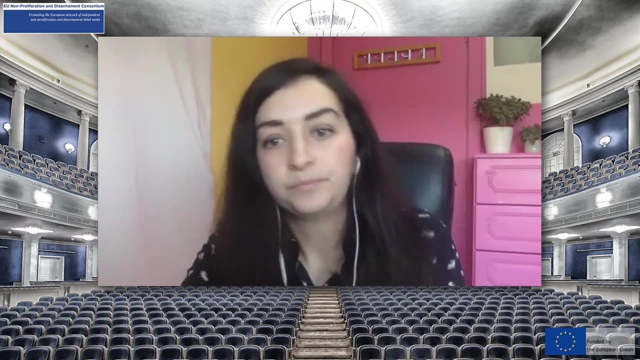 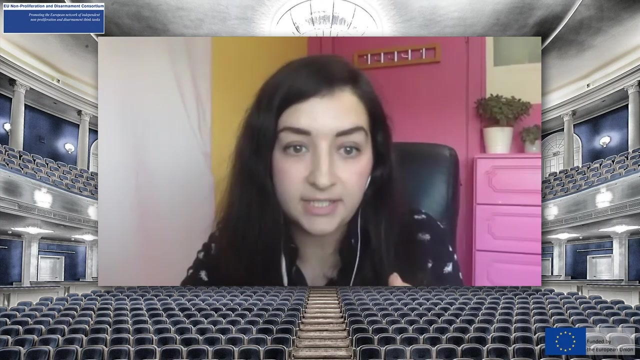 consequences of nuclear weapons. I think this is a completely oversimplified characterisation of the situation. It's not accurate. It's not an accurate description of either position really And, most importantly, it's not conducive to any progress. The supporters of the TPNW, though, sometimes viewed or portrayed as being unrealistic. 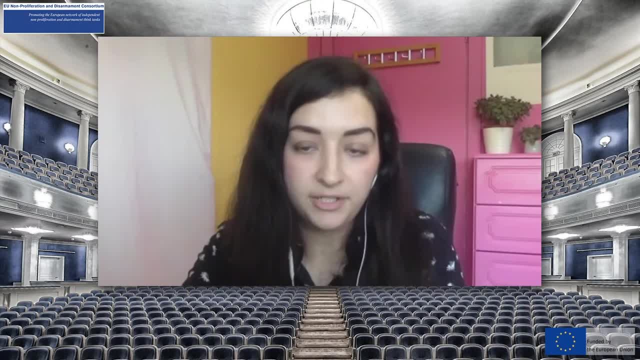 very much share the concerns about the security environment, And many states have been increasingly concerned about the growing risks of nuclear weapons use. In fact, I think the view that we could afford to wait for a more stable security environment before we can make progress. 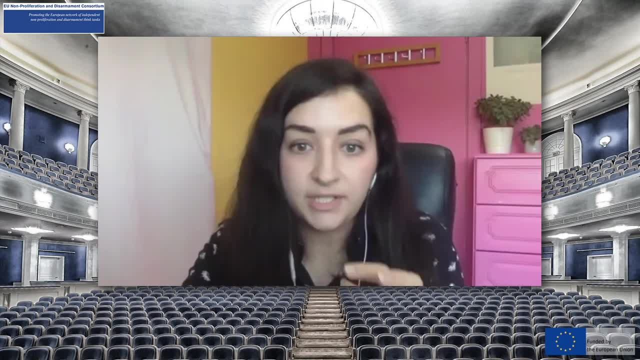 Is the more unrealistic one. It's precisely when we see the risks most that we have to address them, And I think Naomi also excellently outlined you know how challenging these negotiations can often be, And it's not unusual that they're difficult conversations. 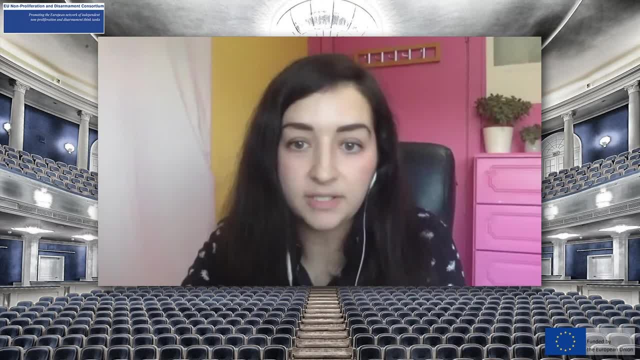 But it doesn't mean that we can't make progress. in these situations, And just to mention the series of conferences that led up to the TPNW on-air, I think it's important to highlight that the risk of an accidental or deliberate detonation 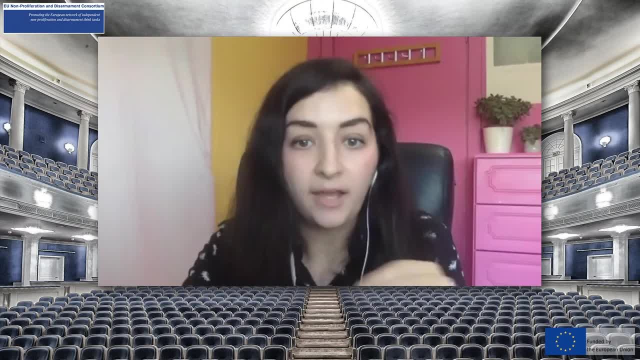 was much higher than had previously been thought And also that it would be frankly impossible to mount an adequate global response to address the aftermath of any detonation, And I think this really galvanized states to develop the TPNW to begin to address these. 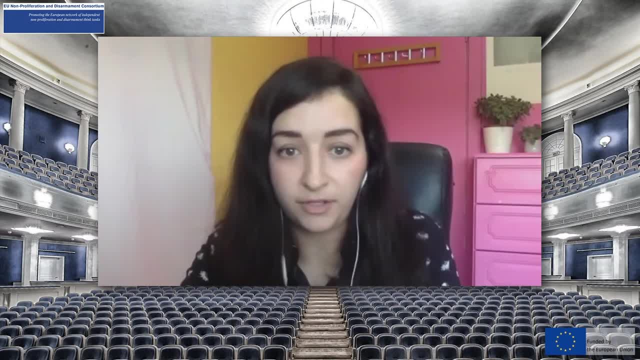 risks And actually, I think, Far from stifling progress, the discussions on humanitarian consequences and on the TPNW have actually been a catalyst for a growing number of conversations on disarmament-related issues. Two that come to mind, for example, within the NPT framework, the conversations on risk. 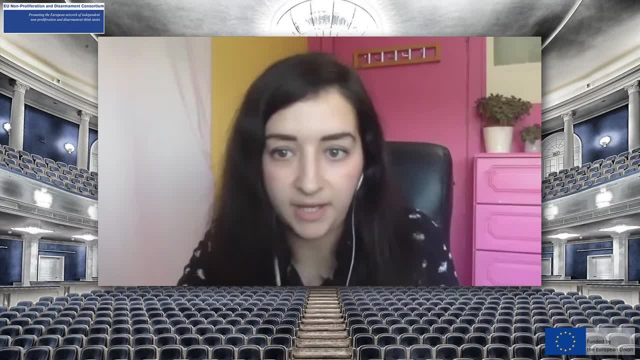 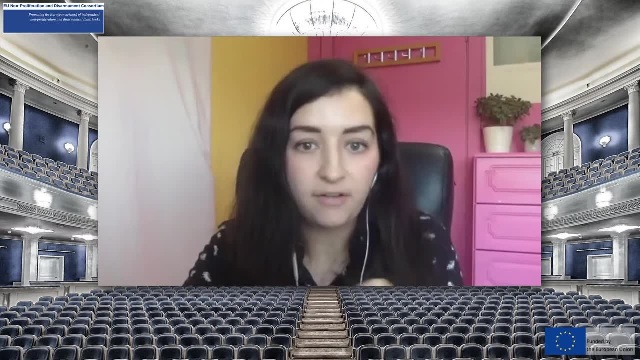 reduction and verification, But I think there's quite a number of examples And I think this has the potential now to bring states with divergent views closer together and find some common ground. I'm really, if it wasn't clear, not convinced by the argument that the TPNW is actually 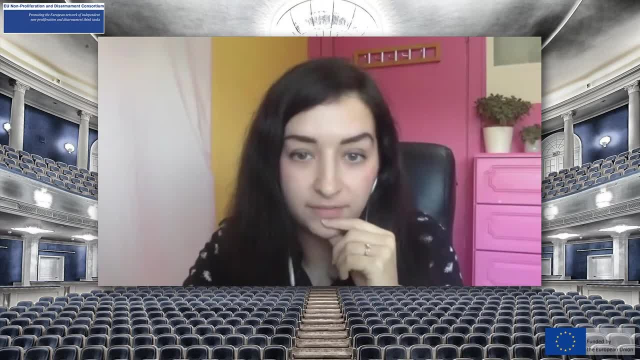 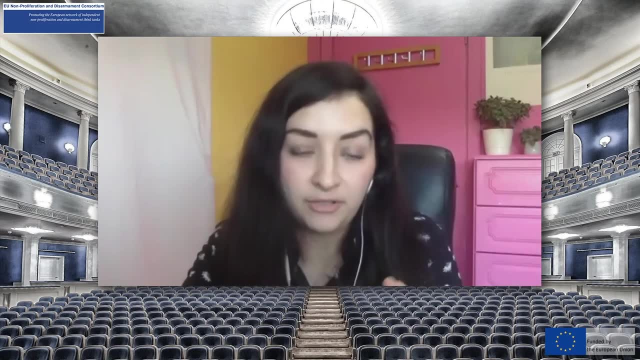 jeopardizing disarmament efforts or increasing security risks, And I think it's as much as it has galvanized support on one side. it's also become a convenient target for blame, where I think there's many other complex factors that have led to the. 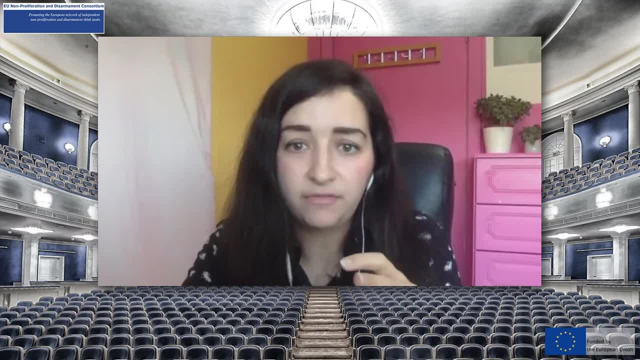 situation that we're in And I just want to touch briefly on the question of nuclear deterrence, And I think we need to properly interrogate the effectiveness of deterrence and to really ask what sort of security is actually derived from it. And I think that's a really important question. 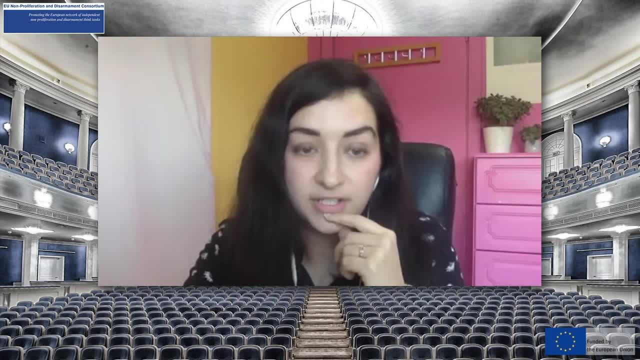 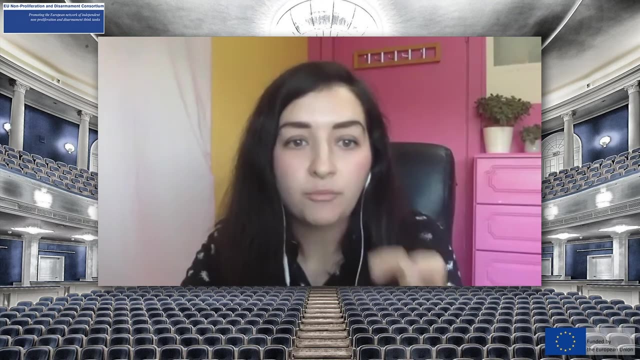 And there's a wealth of academic consideration of these questions that I cannot do justice to, But I'd note the contributions of Chatham House, Unidear and many others for their excellent work on this. that I think is really essential. But that said, we're not much closer to proving whether deterrence actually does what it says. 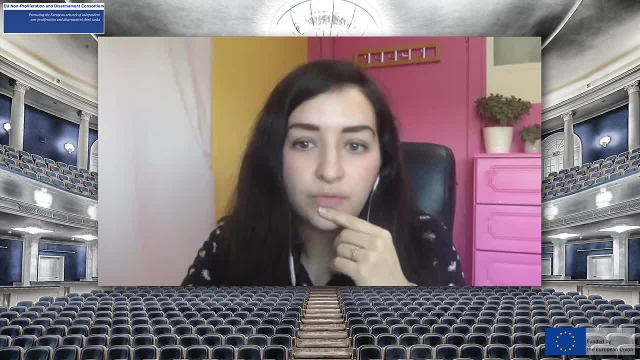 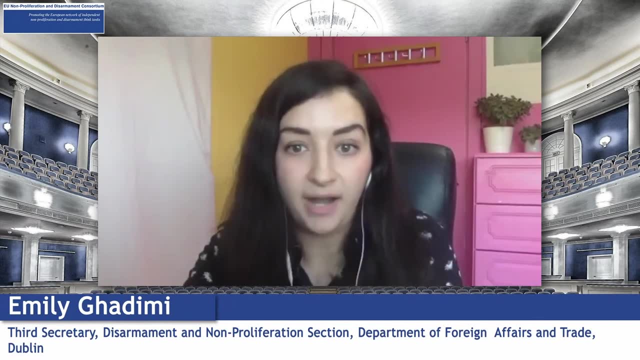 And I don't think we would want to test it. We don't really have any conclusive evidence that it actually functions to prevent nuclear weapons use, And I think it's starting to become more apparent that the current approach is really perpetuating the level of instability that we're in. 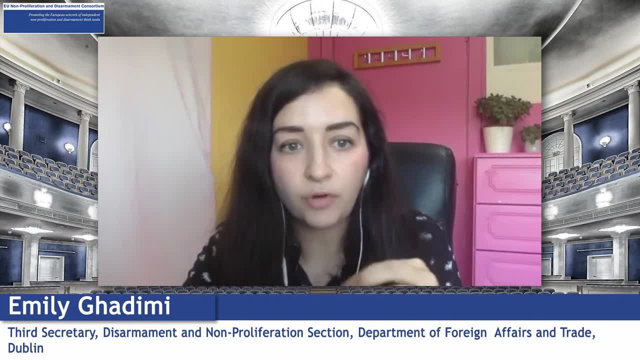 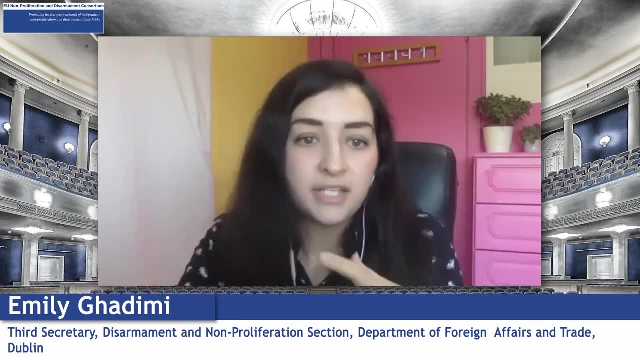 But putting that aside, I also think there is a growing body of scientific and medical evidence of the impact of nuclear weapons that I think is becoming increasingly difficult to see the logic or justify the enduring existence of these weapons, And actually this is something that's really important. 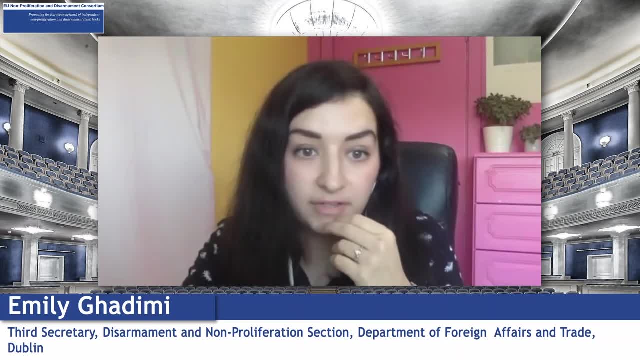 And actually this was already recognized with the adoption of the NPT and in the lead up to the NPT. But it's unfortunate that the bargain struck 50 years ago still hasn't been implemented, And I think we've reached a point now where we need a meaningful reckoning with the question. 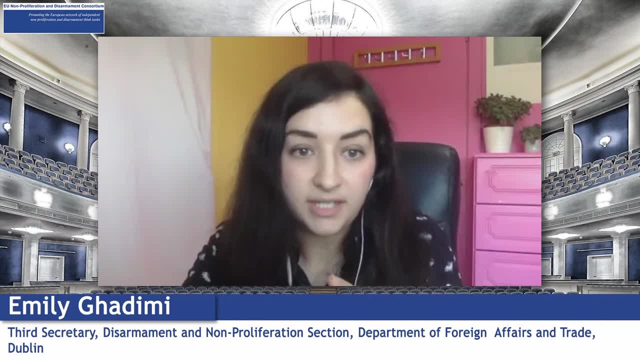 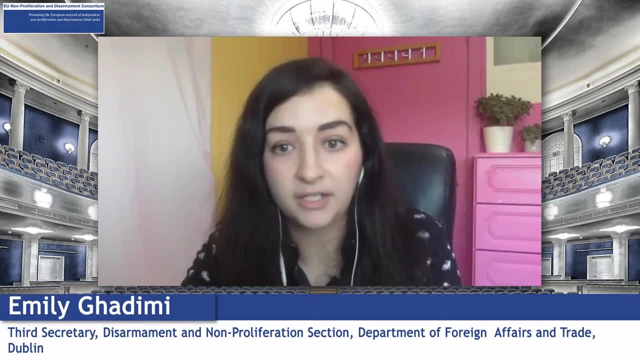 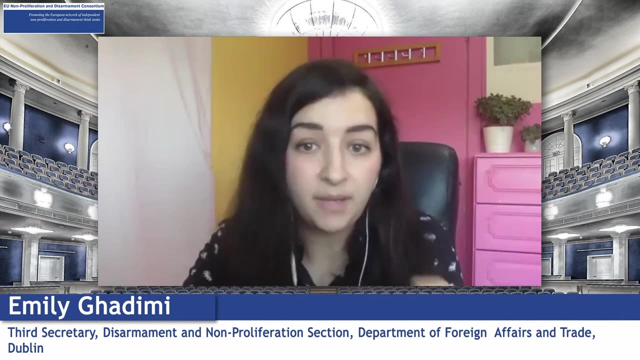 of whether the status quo is sustainable, whether it's effective, whether it's compatible with Article 6 of the NPT or if it's actually threatening, And I think these are questions that we need to consider when we're examining what the impact of the TPNW might be on the NPT. 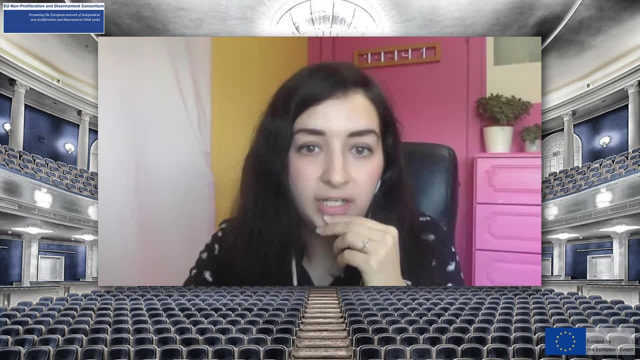 I will just briefly say I don't really agree with the argument that the TPNW is not compatible with the NPT. It's mentioned in its preamble. It explicitly notes that it won't prejudice any other obligations. It's not, And there's established treaty law that you know, I think is quite kind of clear on this. 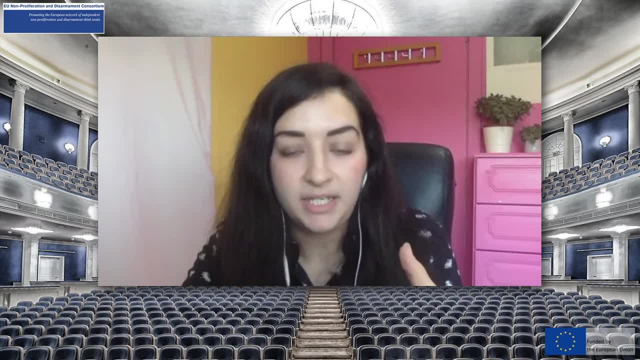 And just to say also, I mean the other pillars of the NPT. it's clear from the other pillars that further legal instruments were envisaged, And I don't think Article 6 is an exception in that. But what I really would like to sort of how I'd like to see the shift in thinking is just: 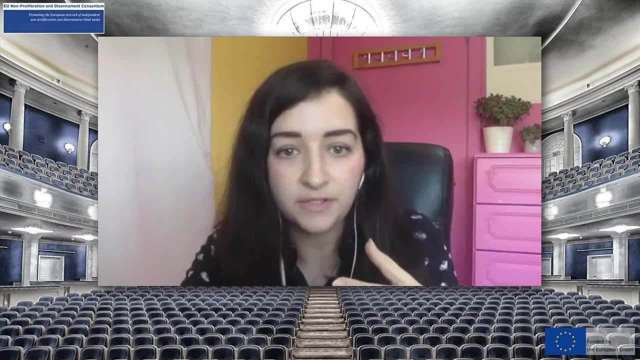 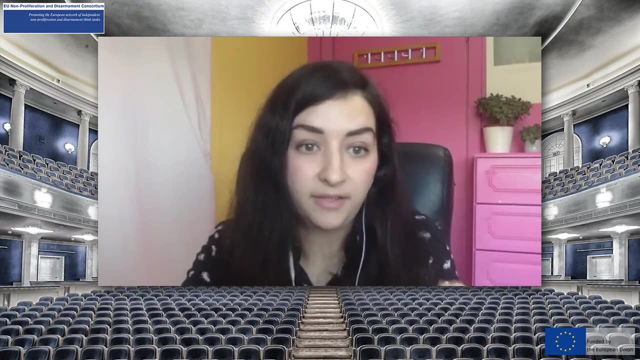 to consider What feasible options were actually available to concerned non-nuclear weapons states who are legitimate stakeholders in the NPT, about what options were available to them in you know, faced with the lack of progress on the implementation of Article 6.. And I think that you know that context is really important in that issue. 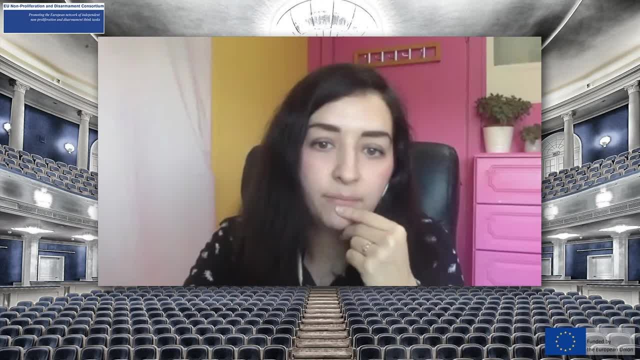 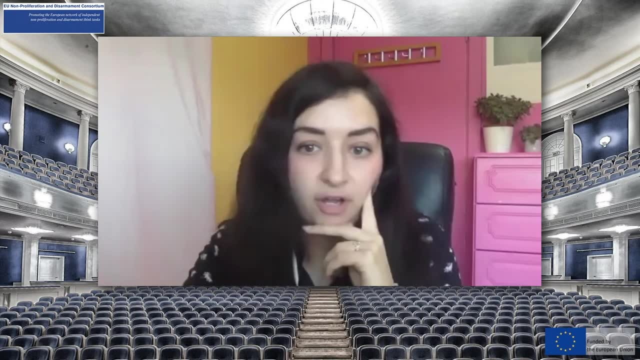 And just to sort of wrap up. Finally, There was There was really intense speculation in the lead up to what should have been the 2020 RevCon about what impact the TPNW would have, And I think there was a level of pessimism about reaching an outcome at all. 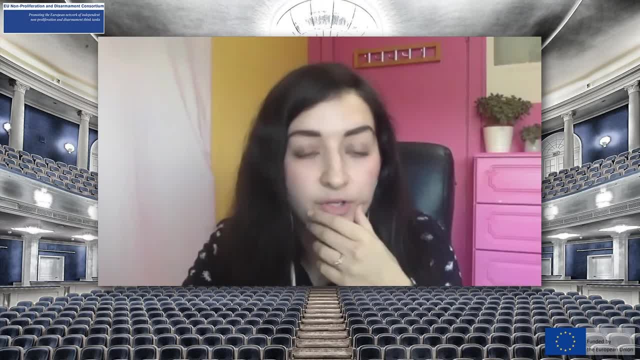 We've. you know, it failed in 2015 to reach any outcome, And I think there was already a sort of oh, the TPNW is here. now we can't do anything, But, among the many unforeseen events that we faced this year, the entry into force of 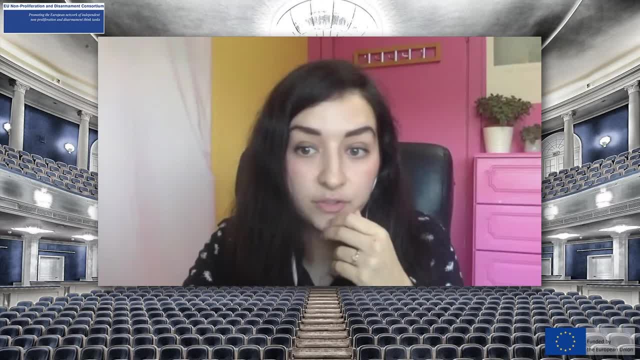 the TPNW was one that we hadn't expected to happen so soon, And now it will be in force well in advance of the rescheduled RevCon. And the fact is, the TPNW is now a legal reality which can't be ignored. 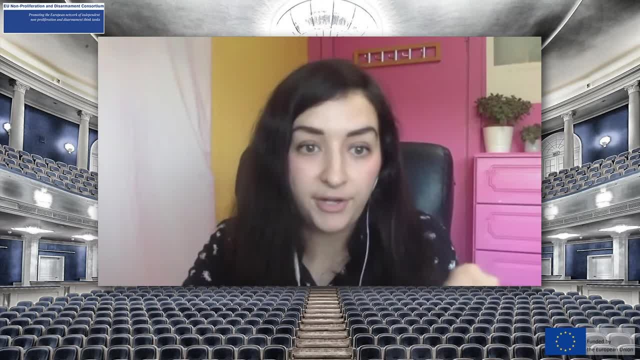 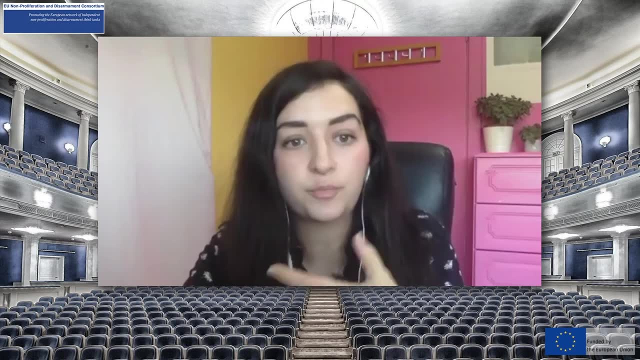 But saying that it also shouldn't become a distraction that dominates the RevCon. There's a lot of other issues that are within the NPT framework. The TPNW is one part of it that should be acknowledged, but it shouldn't be the entire. 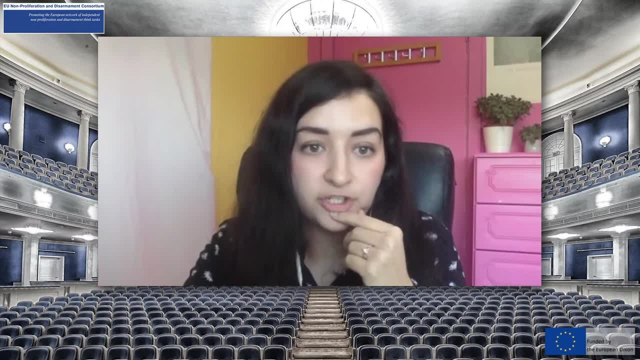 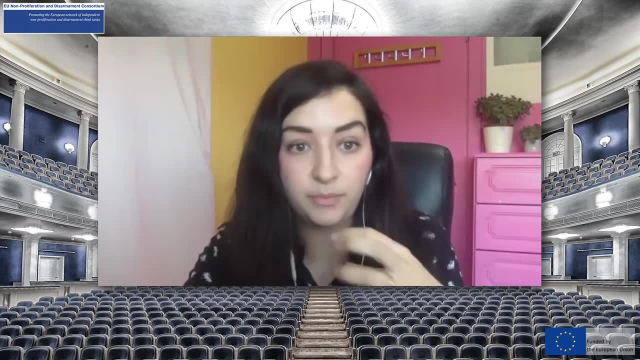 conversation And I really think it would be hugely beneficial for both the TPNW and the NPT frameworks for all states, regardless of their positions, to engage constructively. We will be in the next year or so having the first meeting of state parties of the TPNW. 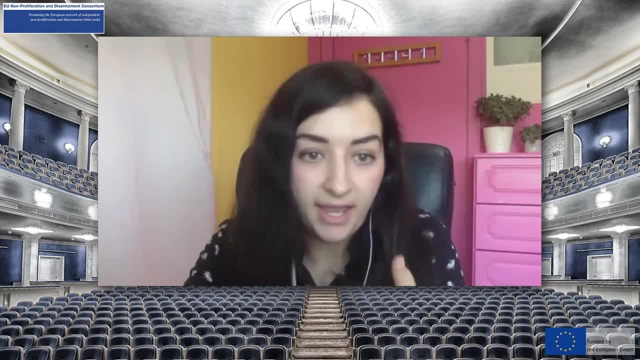 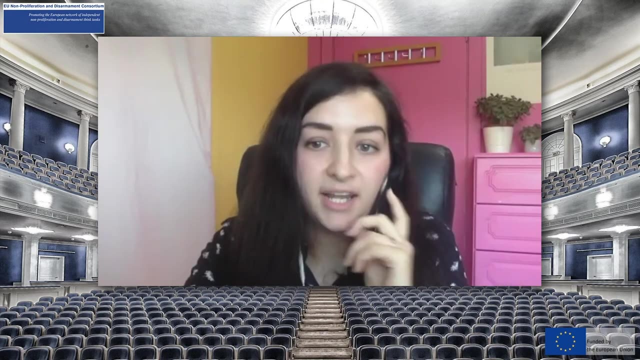 And it would be, I think, excellent if states that maybe don't agree with it still can participate and, you know, start to engage with this as a treaty. That's to say, like I don't think the TPNW is a silver bullet, but it is an important. 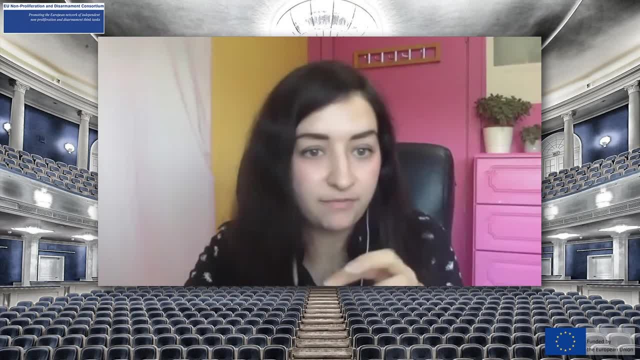 part of the complex and multifaceted steps that we need to take to achieve the shared goals that we have of a safer and more secure world, and one that's free of nuclear weapons. So thank you so much again for the opportunity to share the thoughts on that. 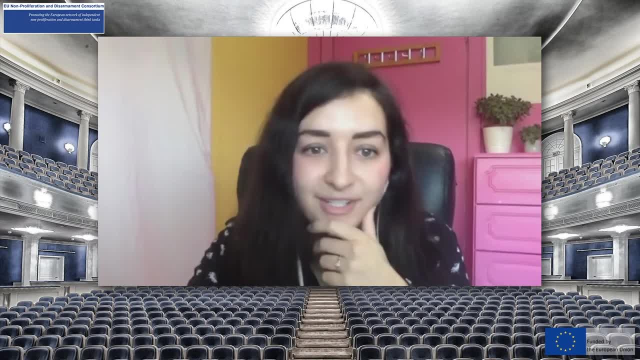 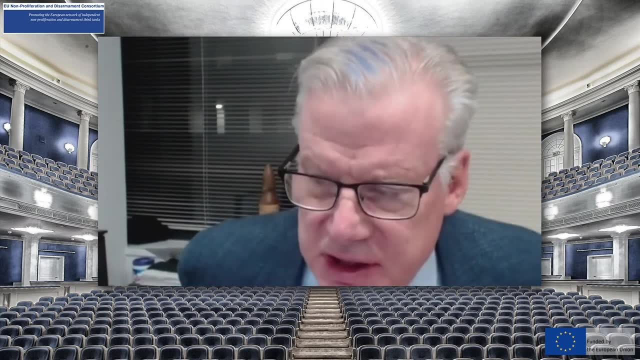 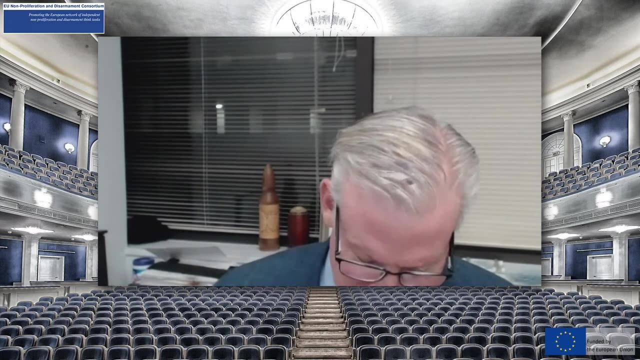 And I really look forward to the discussion. So I'll hand back to you, Mike, Thank you. Thank you, Emily Again. excellent presentation And you know there was a lot of talk about pessimism about the future. While I am somewhat pessimistic about some issues related to nuclear weapons and the 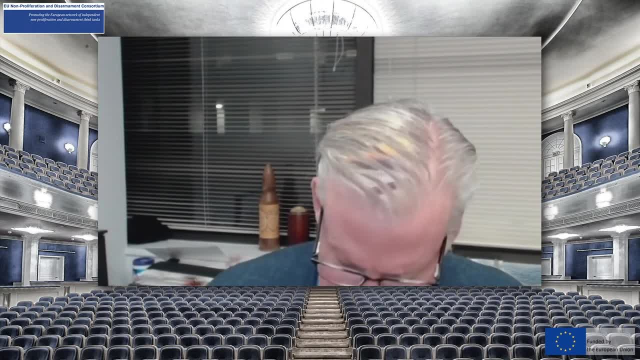 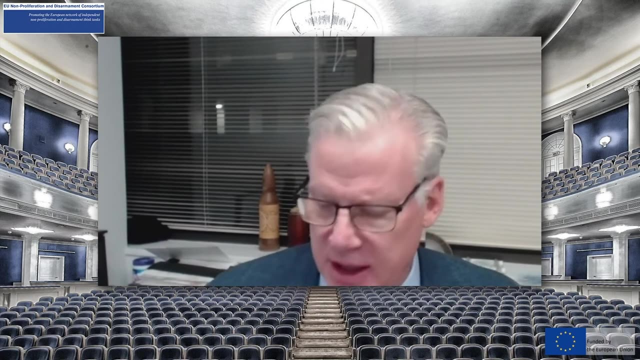 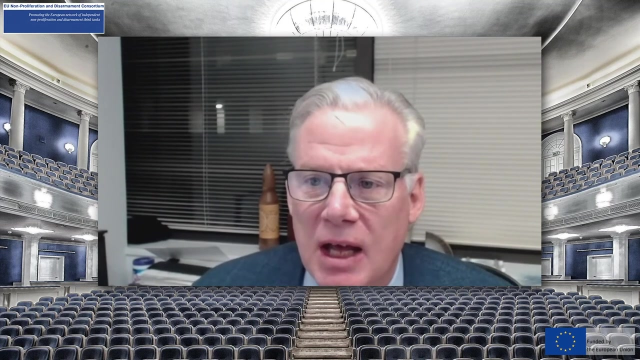 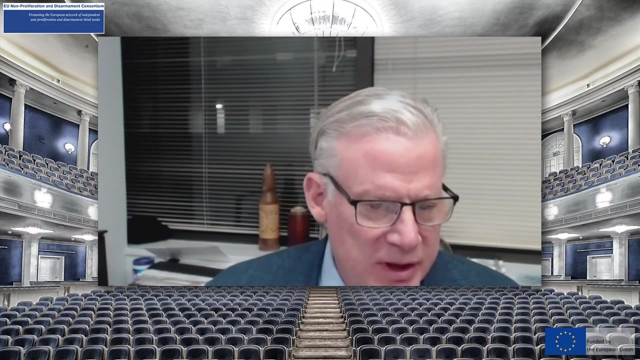 control of them. I am very optimistic that the future is bright, given the presentation So I've heard here today, So I really would like to congratulate all three of you. We've moved now to the question and answers period, and I believe that you can raise a blue hand, if I'm not mistaken, or you can, I guess, click on your- what do they call it? the video, and then kind of raise your hand and grab my attention. 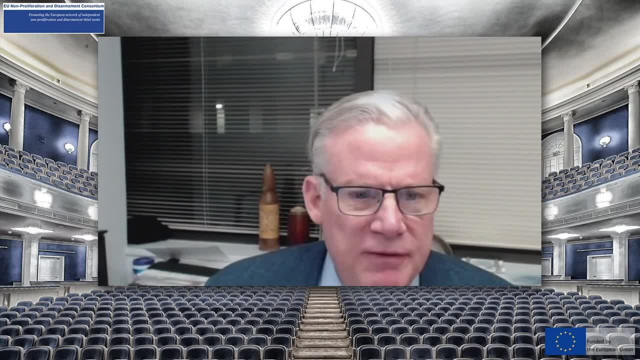 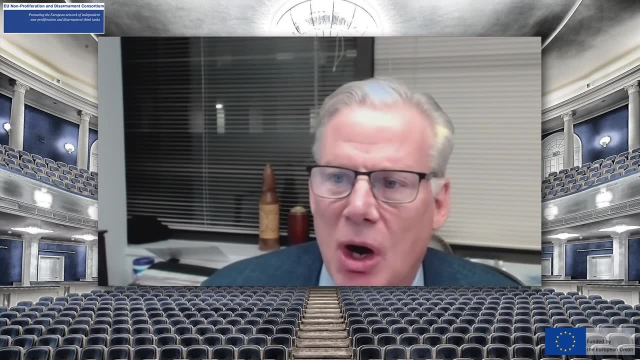 I think that's great. I think you should pop up. And, Federica, if there's another mechanism for them to submit questions through the chat box or whatever, I'd be happy to take them on. So I ask that people don't be shy. 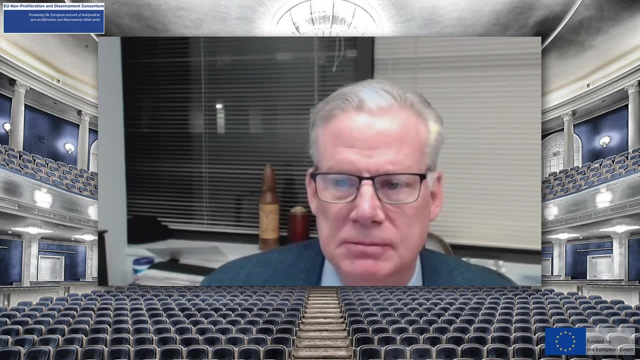 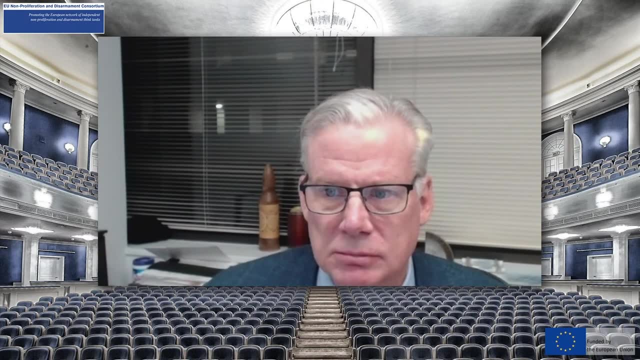 That's correct, Michael. If participants want to ask questions, if they want to do it in video, they can raise their hand and then you can give them the floor. You will see them in the attendees list. You will see the raised hand there. 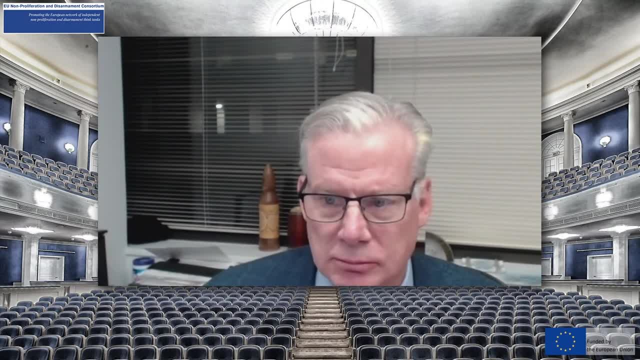 But they can also write questions if they don't want to appear in video in the Q&A box, So you might want to check that. I don't see any questions right now, but you might want to check that too. Yeah, 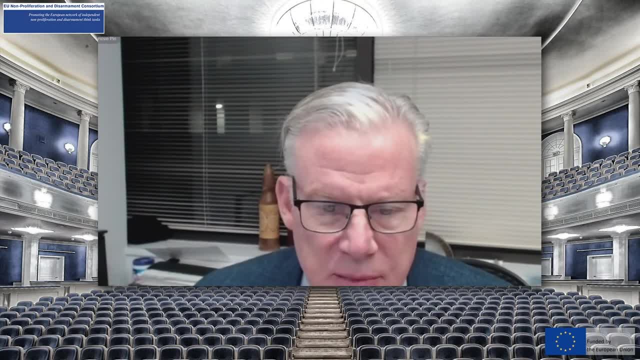 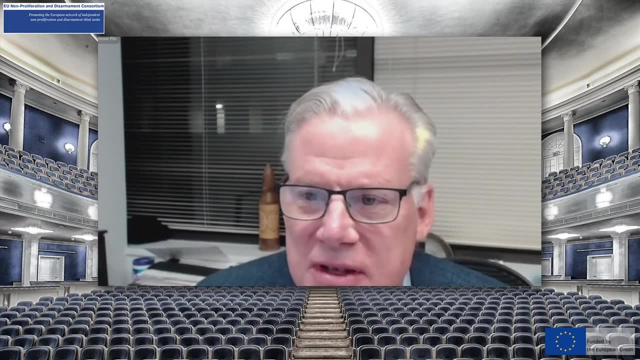 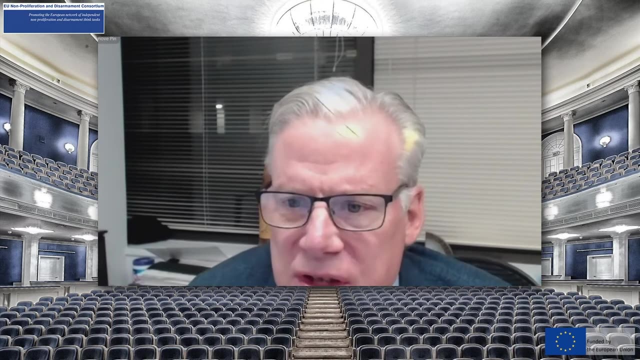 I do have some questions and as other people move forward, but I see that I have one already, So I'm going to read this question And, if there's some time left over, We have about 15 minutes. The Russian approach to this is from Ludovica Castelli. 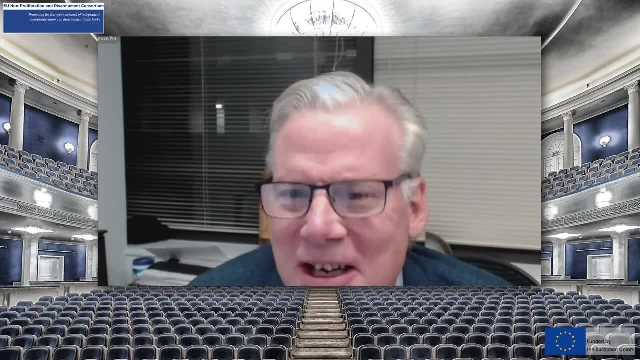 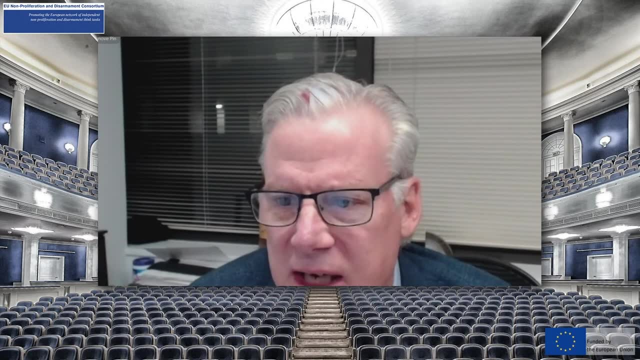 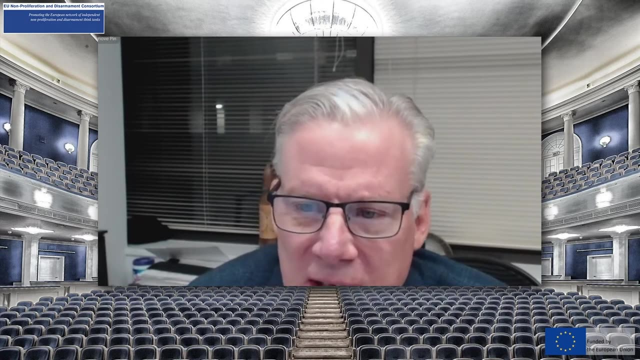 I think I got that right. maybe The Russian approach to the TPNW has been changing over time, from describing it as problematic and dangerous to the NPT during the negotiations up to ultimately defining it as harmless and useless. I guess there are a few open practical questions. An intriguing one involves Kazakhstan That is both a member of the TPNW and a Russian CSTO ally. According to the TPNW, Russia's use of the Sary-Shagan test site for ballistic missile testing can now be banned. The question would be if Kazakhstan will be pressured on this point and if, ultimately, these kind of issues will be solved bilaterally, especially when it is about countries who don't want to do this. Thank you. The question is whether the Russian side will back Moscow up to possibly take a decision that will be unconstitutional, and is the latter going to have to terrible consequences? The question also railing the TPNW as many other countries who don't want to risk complicating their relations with Moscow. 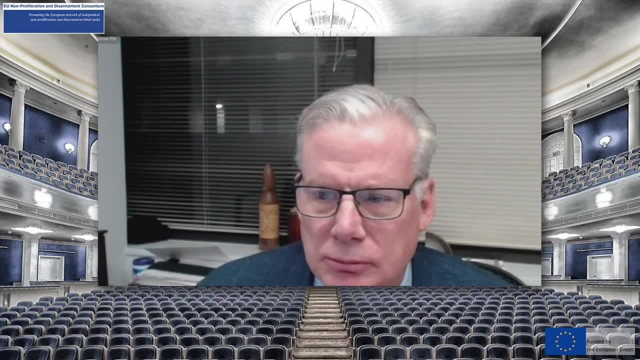 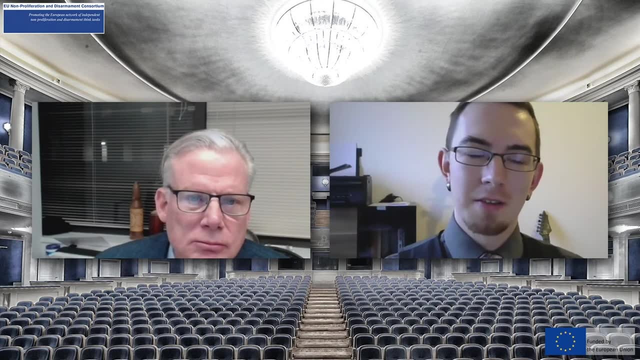 Do you have any takers on this one? I can give a few brief reactions, Okay, So first of all, on changing Russian attitudes towards the TPNW. this is weirdly satisfying that Russia has shifted from. a stance of the TPNW threatens the global nonproliferation regime and will lead to its downfall. 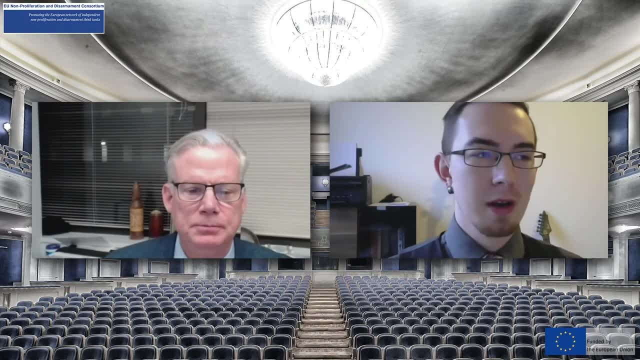 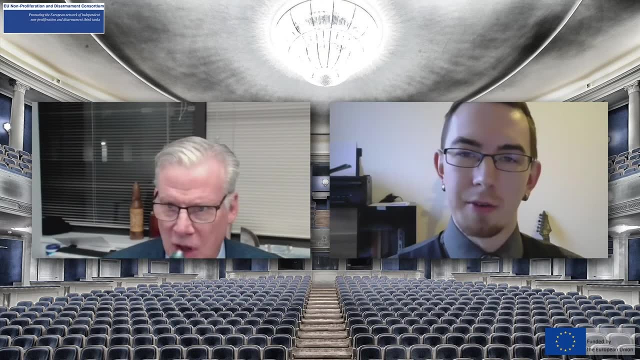 In general, just a few questions from Russia and will lead to its downfall to a sort of- for lack of a better term- apathy, So I see that actually as a positive development from this policy standpoint. The practical question is interesting involving Kazakhstan. First of all, as I'm sure we're all aware, Kazakhstan has a long history of suffering from the effects of nuclear tests, And so, despite the CSTO status and close relationship with Russia, I would severely doubt that this would impact in a serious way Kazakhstan's opposition to nuclear testing. 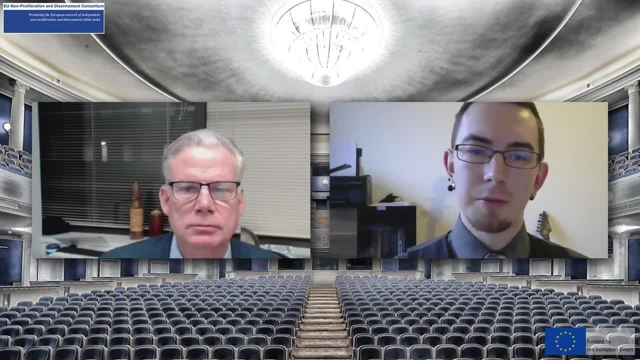 But not being a scholar on the TPNW myself. if the ballistic missiles are not armed with nuclear weapons, I don't believe that's a direct violation of the TPNW on Kazakhstan's part. But those of you who are more well-versed in TPNW, 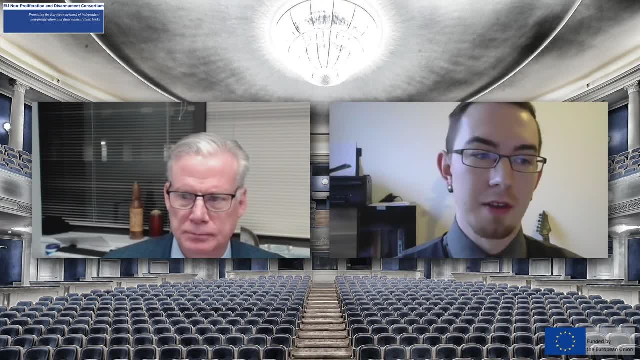 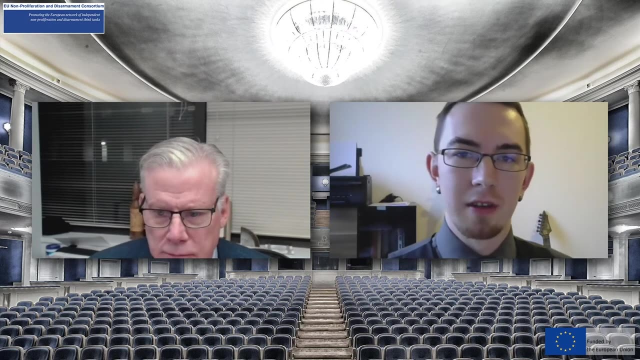 TPNW's specific provisions. please correct me if that is not correct, But again, despite the close relation between the two countries, I wouldn't expect that Kazakhstan would simply cave to allow Russia to conduct these tests, if it would indeed be a violation of the TPNW. 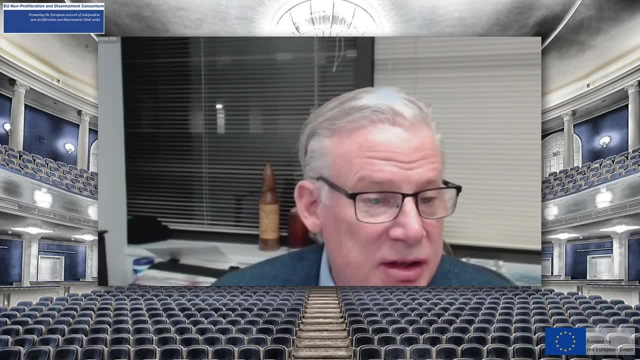 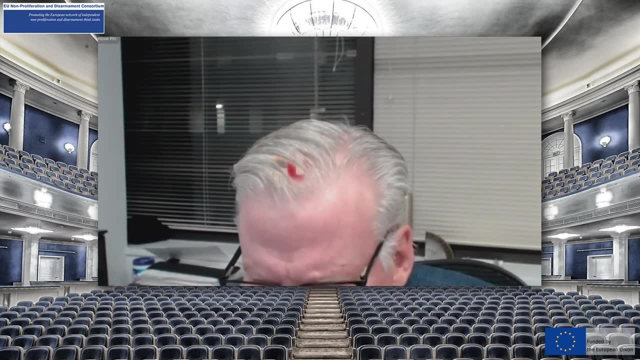 Great, Thank you. Does anyone else, either Naomi or Emily, want to say a word? I believe that if you do, I'll recognize you And that there is someone who does want to answer the question live. But first to Emily. 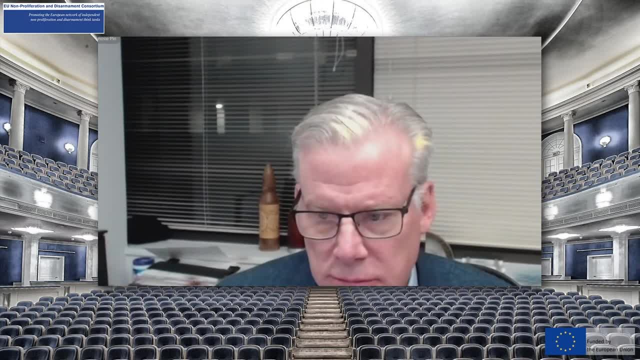 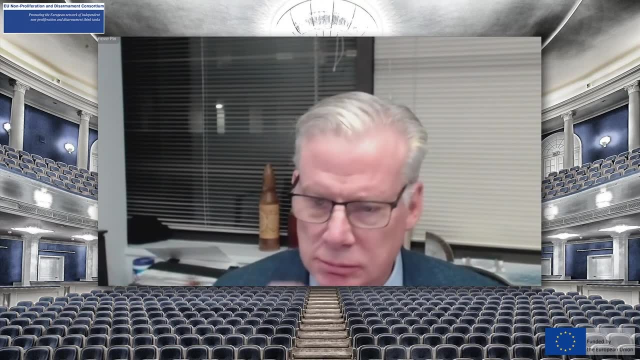 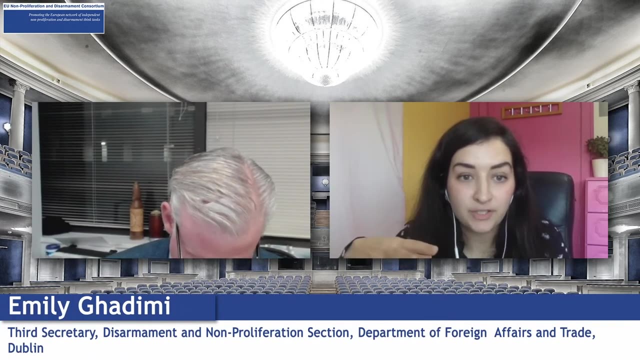 Yeah, I'll just jump in quickly on that question as well And just sort of, I think, maybe generally on the kind of changing attitudes. I'm also sort of optimistic about this. I think in some senses to have apathy, as Noah puts it, from a nuclear weapons state. 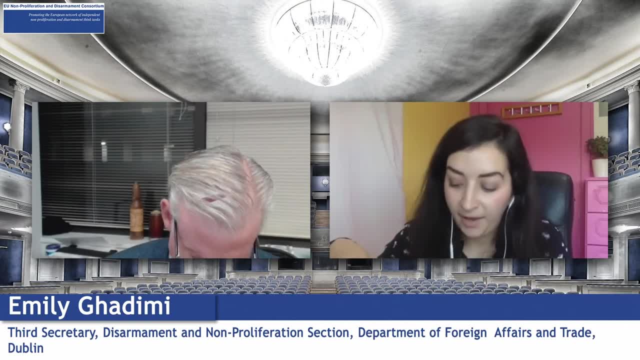 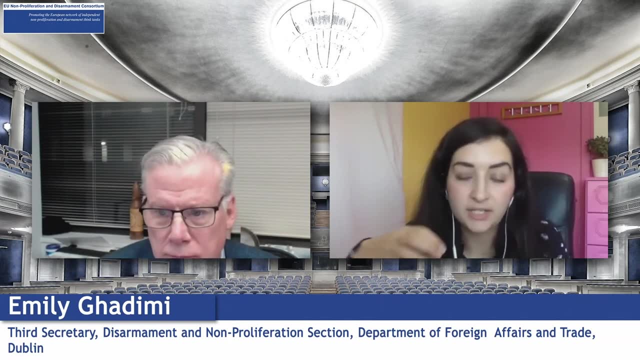 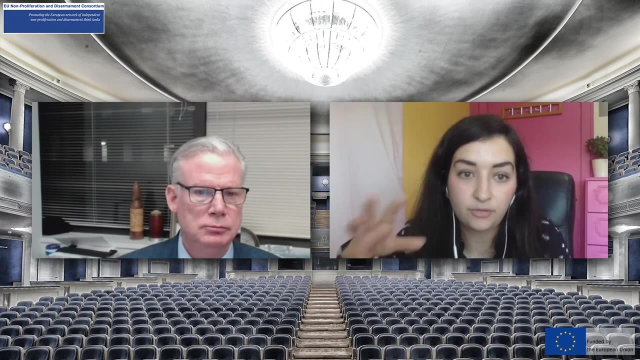 I think is possibly the best case scenario at the moment. But also I think we are starting to see a shift in views with some NATO states and with others, And I think just sort of referring to, you know, going to the RevCon next year. 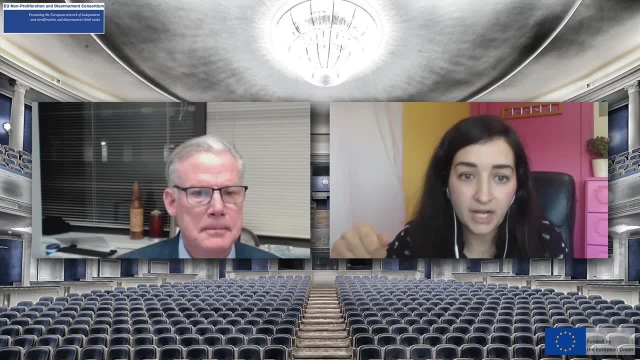 I think if we see a scenario where New START is renewed in some form and there's some, you know, some stability from that and then also this, you know, maybe a little bit more more acceptance of the TPNW, I kind of see, you know, more positive prospects for the RevCon. 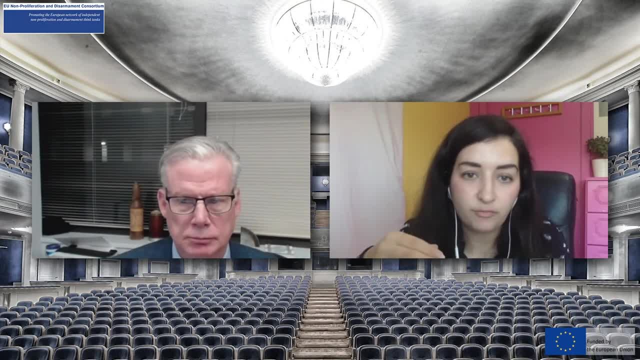 And just on the assistance point as well. I mean it remains to be seen. the TPNW is not in force yet. But I would also agree with Noah's view that, if you know, if it's not involved, like the assistance or whatever the situation is, is not involving an actual nuclear warhead. 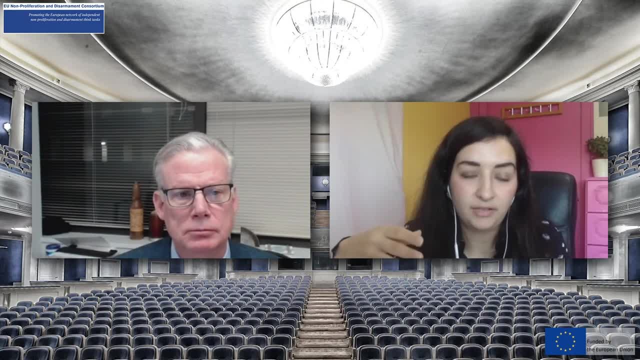 then it doesn't. you know, I don't think it will legally be a violation by Kazakhstan or anyone, And I think just in terms of existing military or other international partnerships, I think as long as nuclear weapons aren't actually involved, then this legally won't have any impact on that. 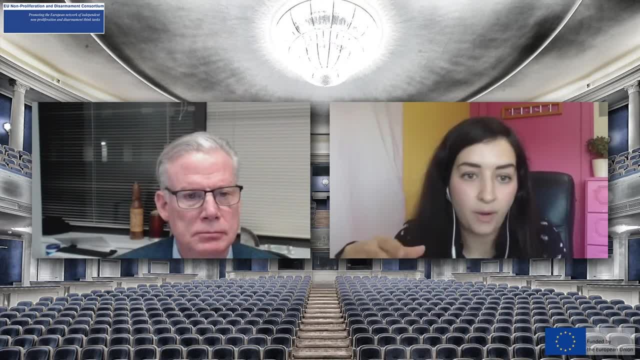 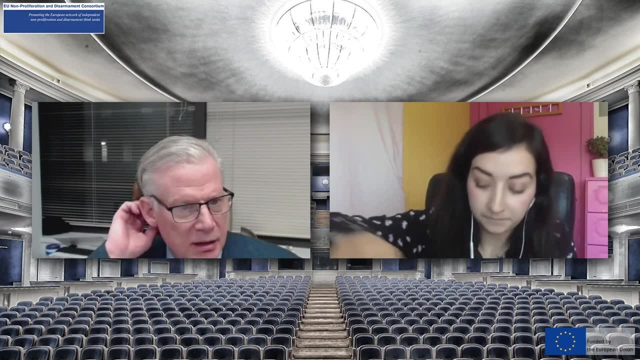 And I think it is one of the arguments that's put forward- that this sort of cooperation won't be possible now under the TPNW, And I don't think that's actually the case. Thank you, Emily. Yeah, it's a difficult question and I'm not a lawyer. 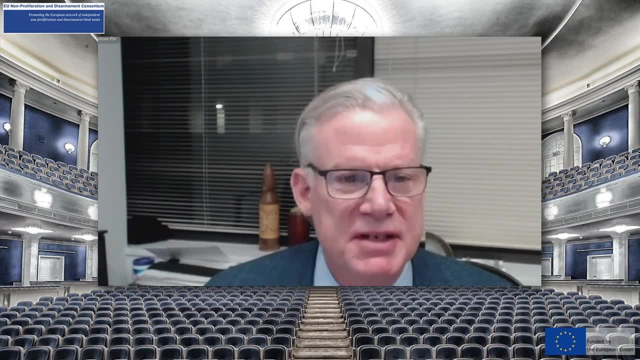 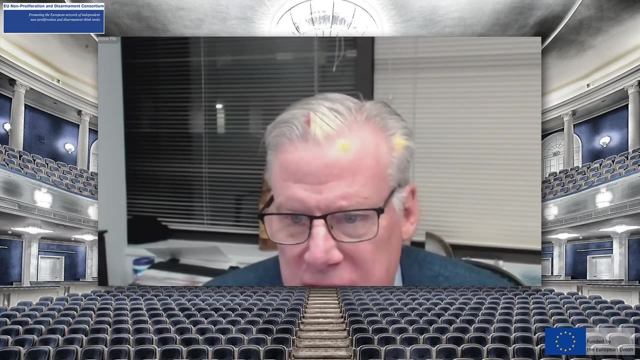 But you know, if the missile is specifically designed to deliver nuclear weapons, one could make an argument that it is part of a nuclear weapon capability. But I'll leave that to the lawyers to straighten out. We have a question from Manuel Herrera to Naomi. 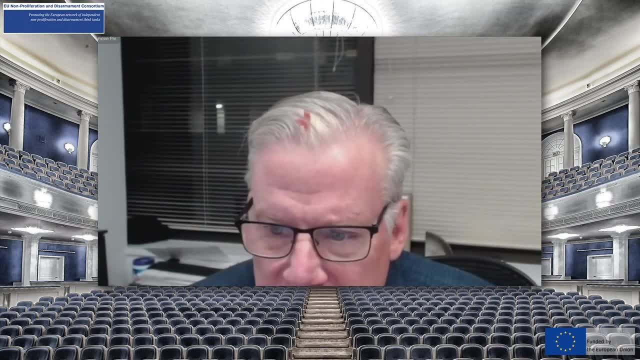 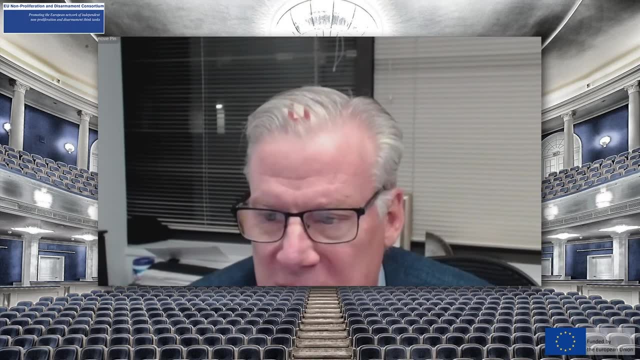 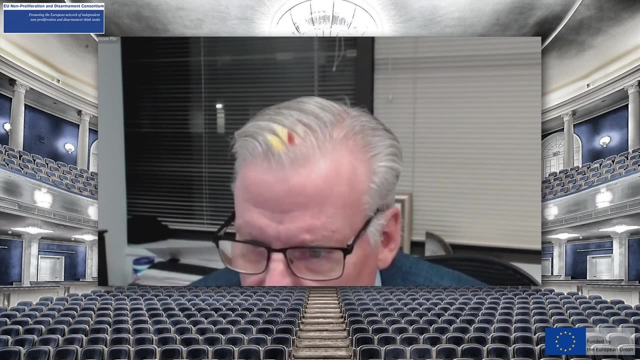 Do you think it is possible that, in attempt to circumvent the parliament, the parliaments and domestic representatives of states that, when ratifying agreements on these matters, in order to avoid the lack or absence of inclusion of states in control of disarmament agreements, 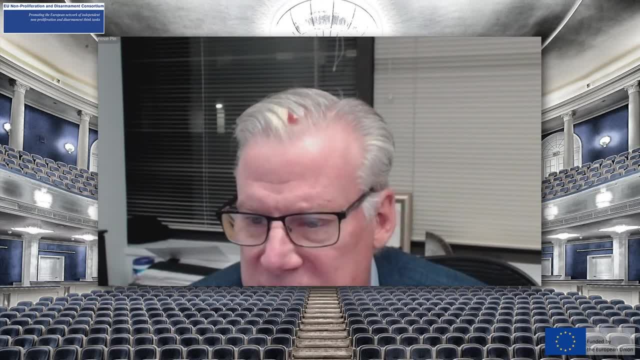 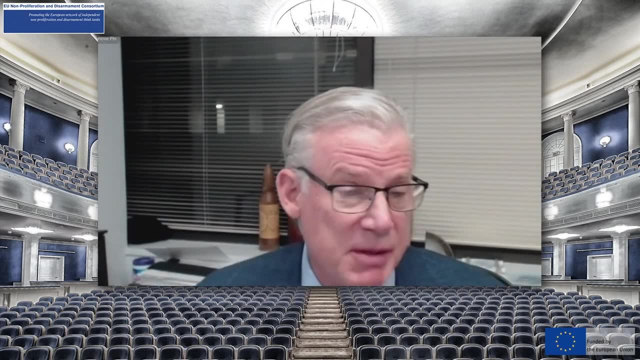 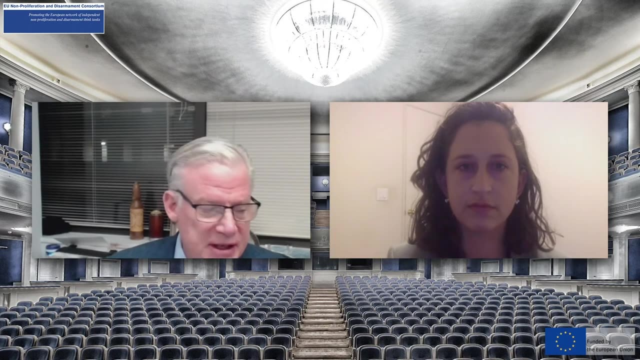 the general public in these countries feel or perceive these agreements as illegitimate or undemocratic? That's a very interesting question and it goes to something that I also wanted to raise with Naomi is, you know, with the domestic challenges as we saw with the JCPOA, because it wasn't ratified by the Senate? the next president could come from another party, can come in and, just you know, withdraw from the treaty quite easily with with little pain. So I welcome your thoughts on on that, as well as the question from from Mr Herrera. Great, Thank you. 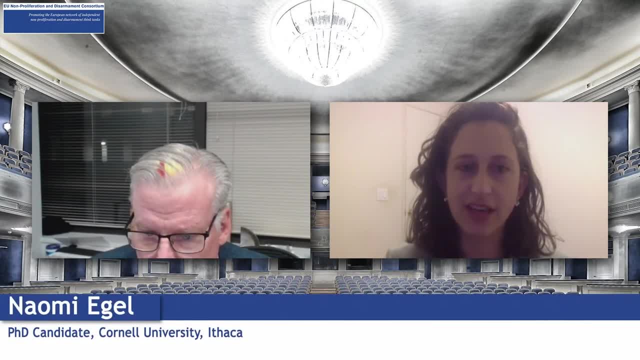 So I think that, from a question of a healthy democracy, that is definitely a concern, But I'll say that it depends on what the alternative is Right. And so if people feel that they are not being satisfactorily represented by their elected representatives, who are supposed to ratify treaties, 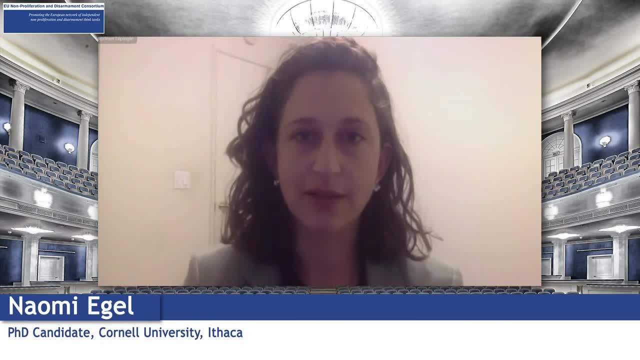 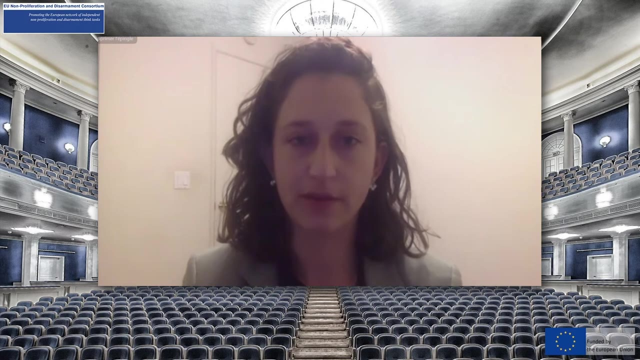 then that's a bit of a different situation. So if we're assuming that people are happy with how their elected representatives are representing them, then yes, sort of going around and work around. but I think that the challenge for treaty ratification does have troubling implications for popular accountability and popular satisfaction. On the other hand, if the problem lies with domestically elected representatives not representing their constituents, then perhaps if the constituents feel that the executive making these agreements better represents them, then perhaps there's less dissatisfaction with it. That's obviously a question that depends a lot on the situation. 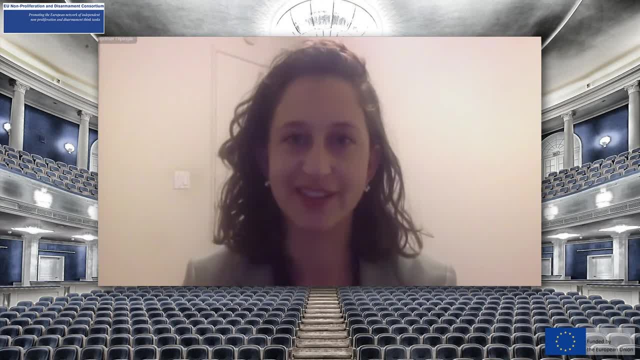 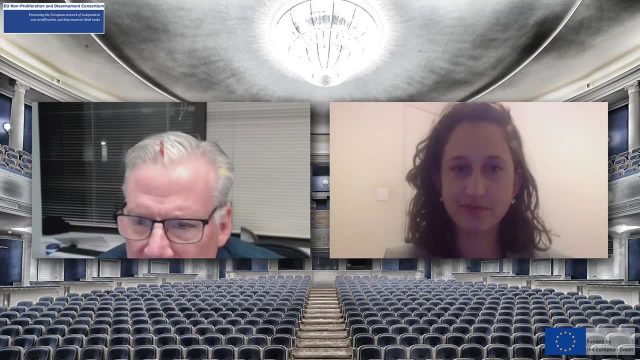 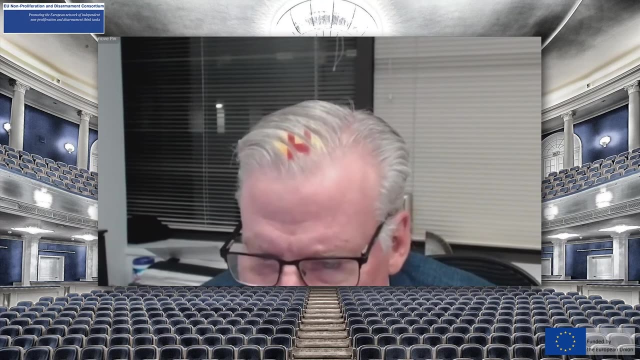 It depends a lot on the particular domestic situation of a particular country, Very diplomatically put. We have two other questions, one from Sybil Bauer and one from Giovanna Maleta. I'm going to ask Giovanna's first because it ties back into the question you just addressed, Naomi. 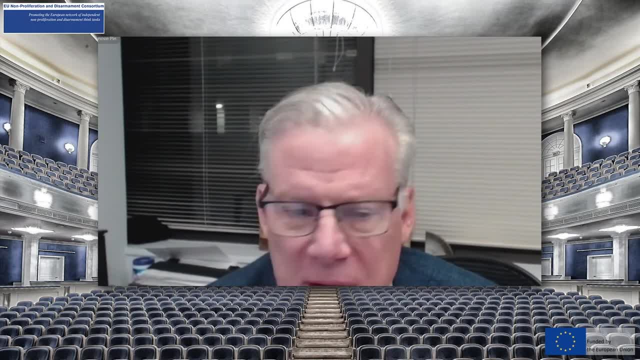 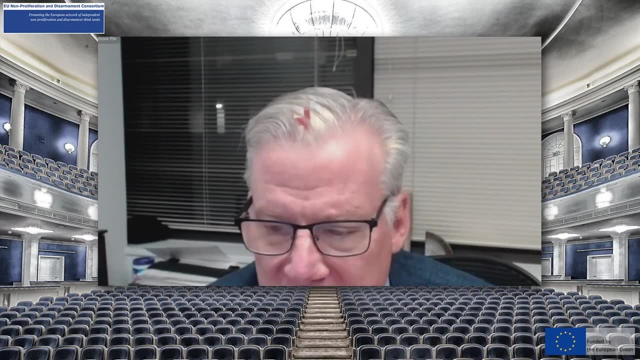 But I'll open it up to to all three of you. But I'm going to present both of them and the questions at the same time to save time, And you can. the speakers can chime in as they wish. So from Giovanna, even if the Biden administration will engage again in arms control diplomacy. do you think this would be enough to restore trust in US, the US ability to fulfill the agreements they participate into in this field, or, more generally, enough to restore trust in international law? For example, what kind of assurances would Iran have? 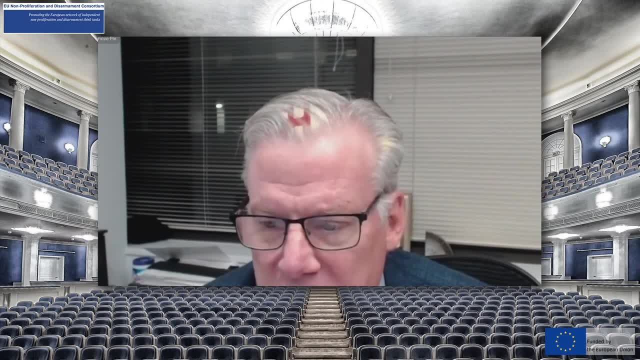 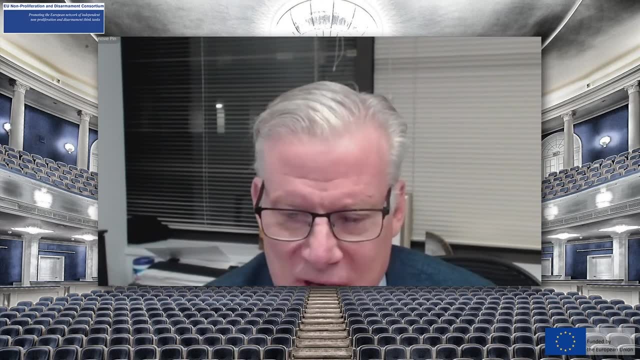 What kind of assurances would Iran have that a future US administration beyond Biden would abide by the provisions of the JCPOA? I think that's a very pertinent question because in our track to track one point five discussions we have with the Iranians. 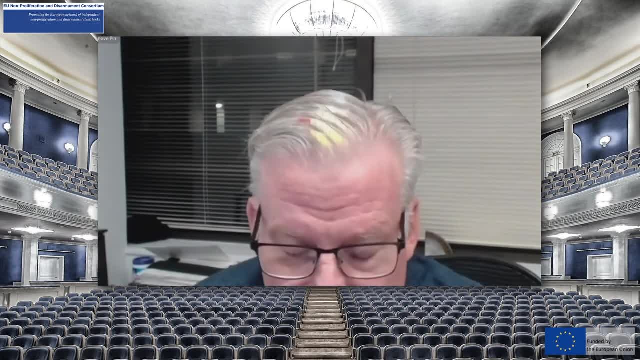 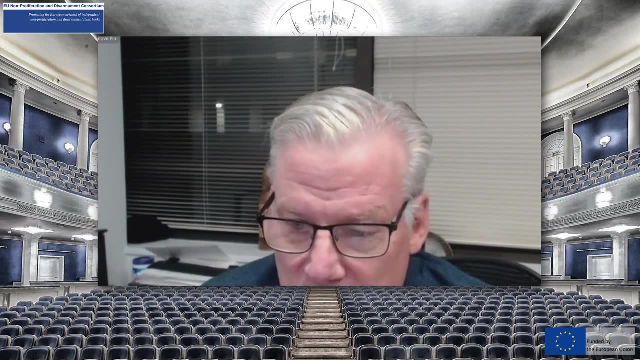 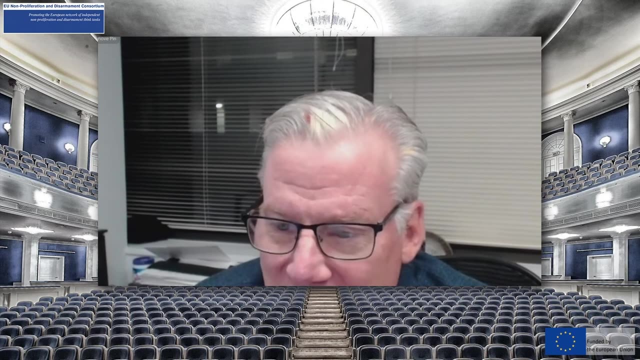 they have raised this very, this issue very specifically when when people talk about Biden as a when it was a potential president elect, whether he would just rejoin the JCPOA, And they have some reservations Along those lines. And then from Sybil, given your refreshingly optimistic, constructive outlooks. 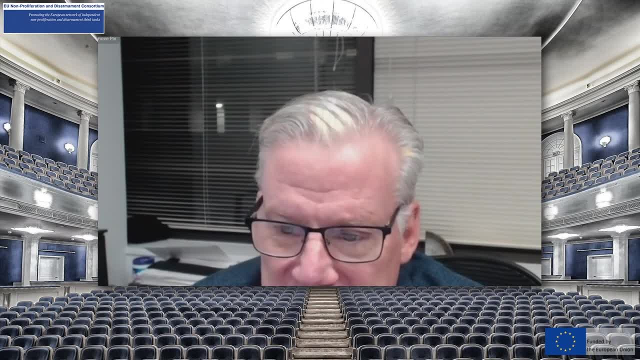 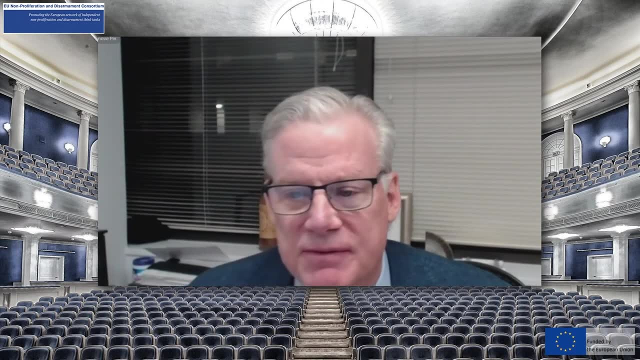 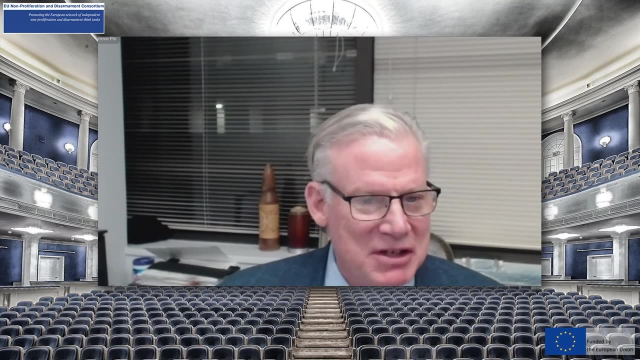 what kind of nuclear arms control landscape do you think could be feasible if policymakers are similarly constructive, say in the next 10 years from now? So I'll start with Naomi, since the follow on question is kind of directed to the initial question you took on, and then move to the other two speakers. 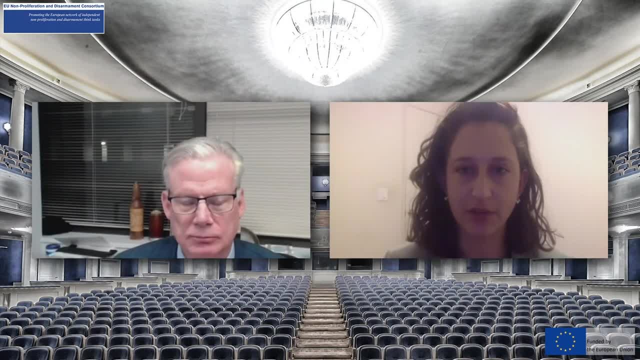 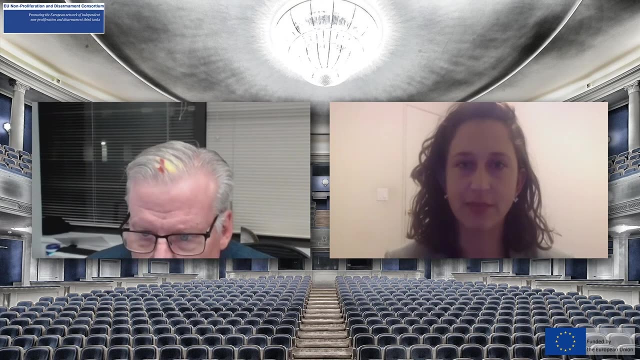 Great, So I'll take them in the order you posed them, starting with the Biden administration question and then moving to Sybil's question. I think this is a really good point And I think that in the US in particular, I'm often struck by conversations that say the Biden administration will rejoin the JCPOA, as if it's the US decision alone to make. 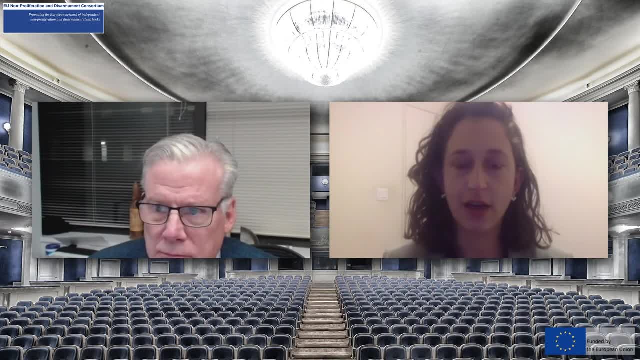 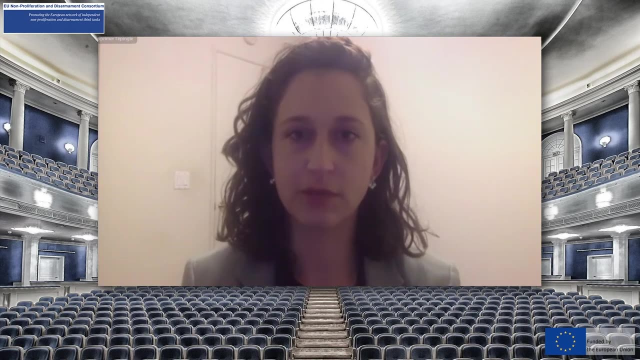 And, of course, it's up to all the parties of the JCPOA to let the US rejoin, And I think that it's unlikely that. this is, of course, my own, But from my perspective, I think it's unlikely that Iran is going to let the US join without any immediate concessions before joining. 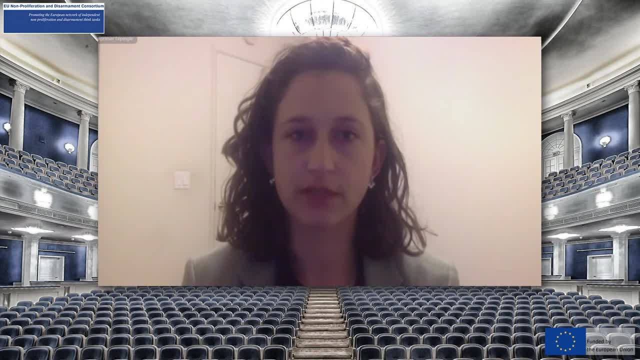 And so I would see things like sanctions relief being a prerequisite for joining, potentially In terms of, more broadly, that is. that's the big question, isn't it? And I am not sure how you rebuild trust with such a whiplash between administrations. 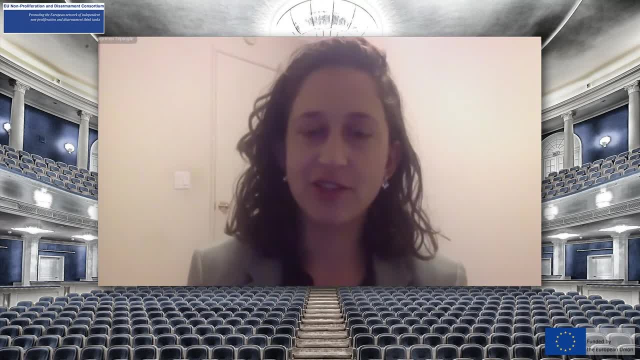 In terms of Sybil's question. being contrarian, I'm contrarianly optimistic. again, I actually see room for regulating hypersonic vehicles under a follow-on to New START. I think the fact that Russia has agreed to include its avant-garde system under New START- and essentially count it as an ICBM, if I'm not mistaken- is encouraging and promising. 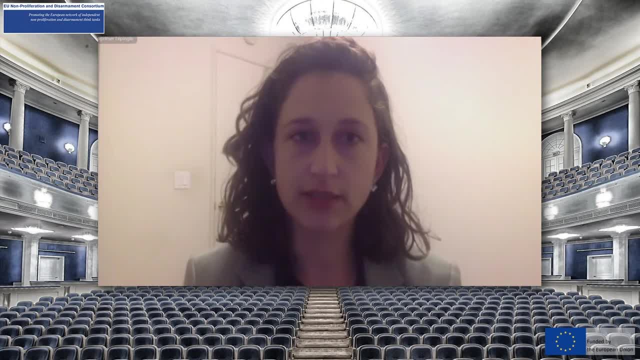 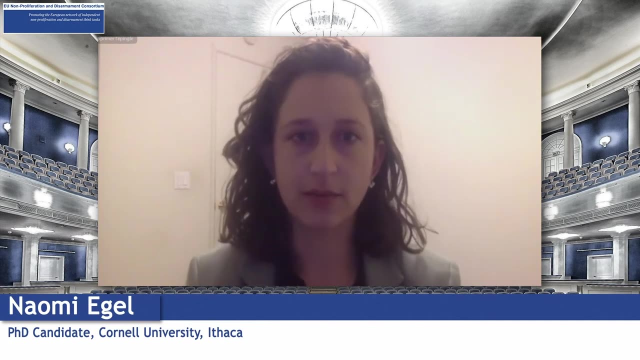 And I think that this offers an important precedent And I hope that future follow-on to New START could take over And I think that future follow-on issues of hypersonic vehicles. I think that the similarity- although they're obviously different than ICBMs- they are more similar to ICBMs, I would say, than something like cyber or autonomous weapons- are to sort of things that exist already, that aren't new in emerging technologies. 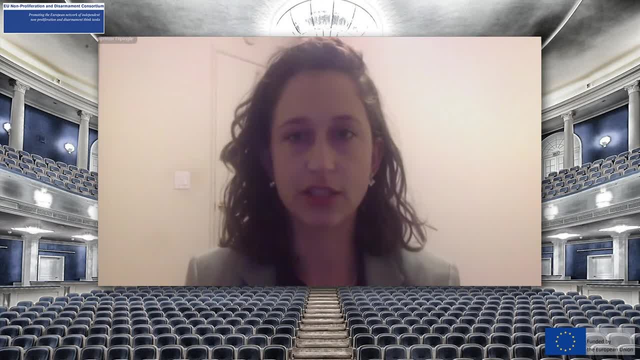 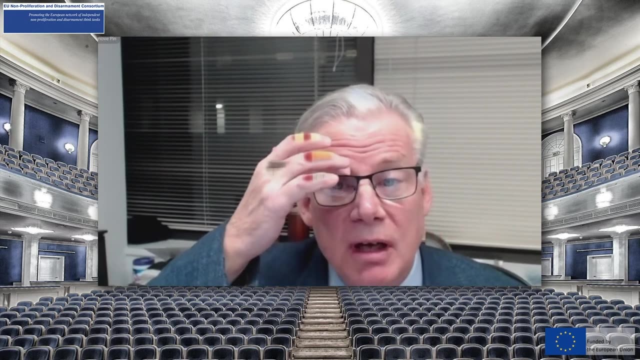 And so I think that if we're thinking about emerging technologies to be regulated, I would say that hypersonics seem to me to be the most promising to be regulated under future arms control in the next 10 years. Thank you, Emily or Noah, do you have points that you would like to make in follow-up to those two questions? 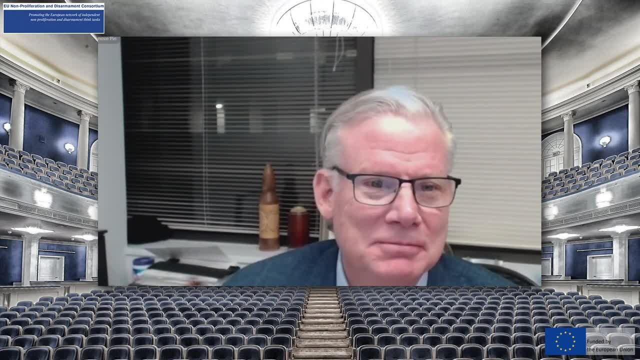 I certainly have thoughts, But, Emily, if you'd like to go first, you're more than welcome to No, Okay, You're unmuted, so let's go with you first, Sure, As far as the question posed by Giovanna, I think that Naomi sort of hit the nail on the head. 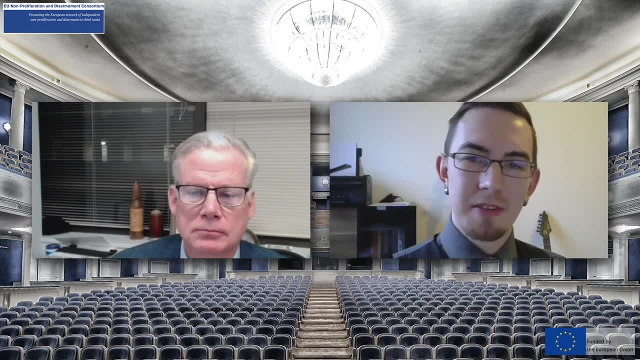 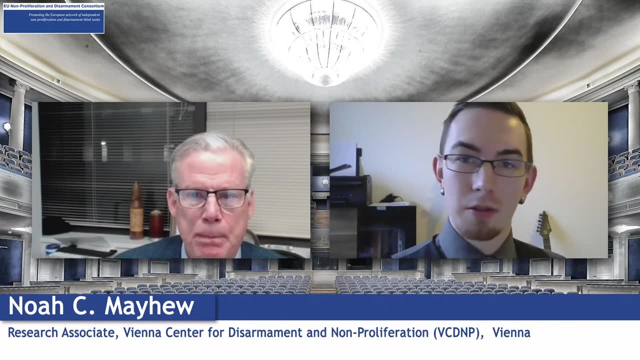 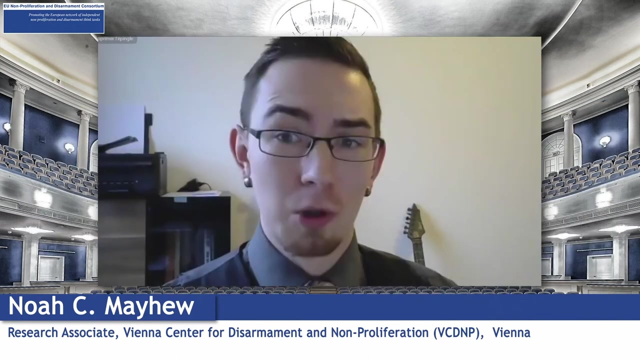 In a broader scheme. It's sort of a sad fact That's the American system. But having said that, so to say, a new president can make the rules with things like this, but in a very sort of simplistic way. But having said that, something I hope we all understand is that the Trump presidency- his politics aside, the Trump presidency was not normal. 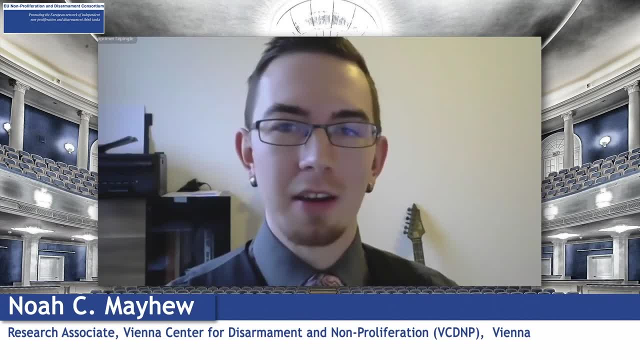 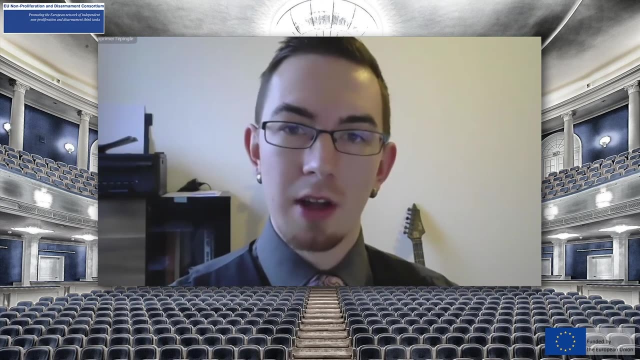 I saw a report recently that advocated for many of the domestic US systems procedures- let's put it that way- on how these things are done are based on norms that we on a domestic level have never had to question before because we've never had Donald Trump as president. 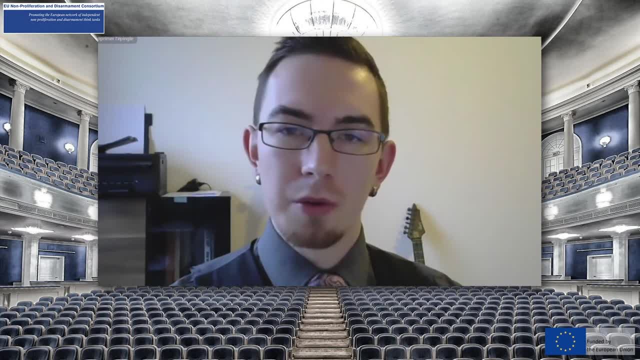 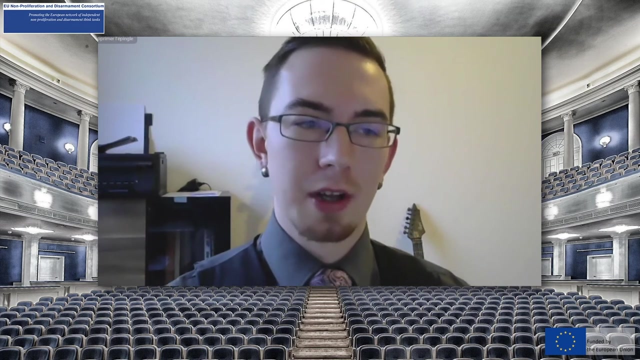 Now, that's not suggesting that, following Joe Biden's presidency, there could not be another person such as Trump who's happy to just rip up the playbook. But unless some of these procedures and regulations- Right that are, you know, ratifying agreements or acceding to agreements or whatever- are more concretely rooted in the US system, that's just the reality that we're going to have to live with for the time being. 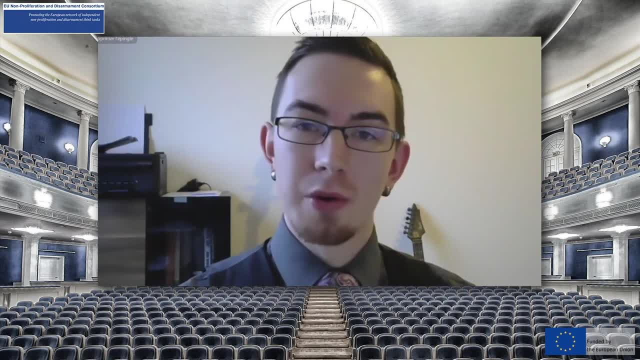 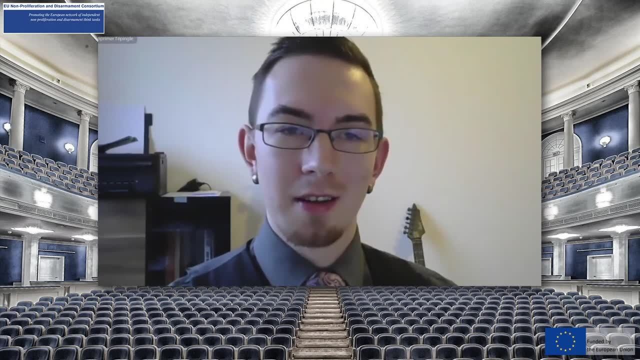 And I agree with Naomi: After such a whiplash, going from someone like Donald Trump to someone like Joe Biden, restoring trust is going to be difficult, And you know I don't have an answer for that either, But you know. 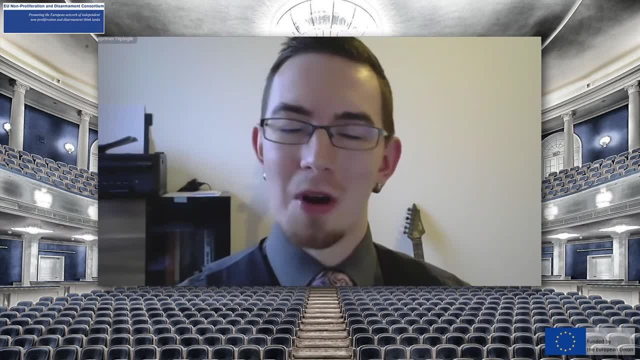 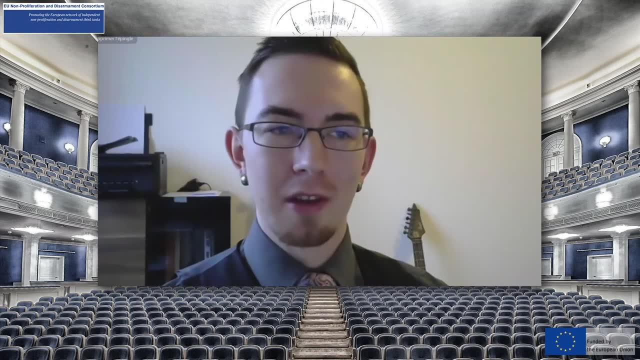 I hope that this will serve as an example of what not to do in the future. referring to Donald Trump's presidency, Because, again, my personal views on the man aside, his policies and arms control were indeed been very destructive To Sibylla's question- there are lots of possibilities. 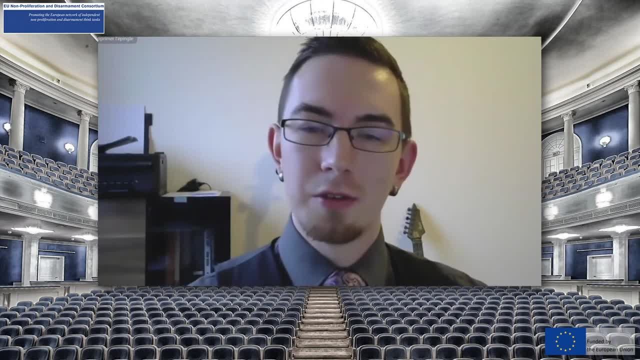 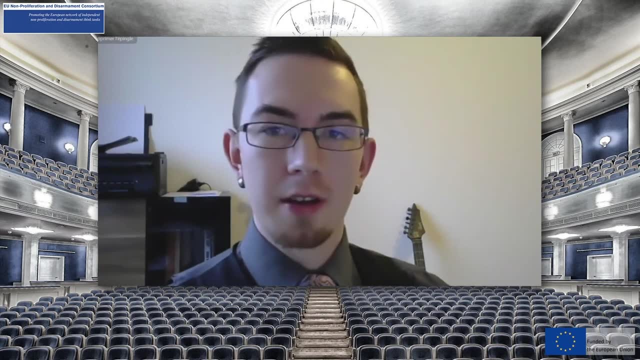 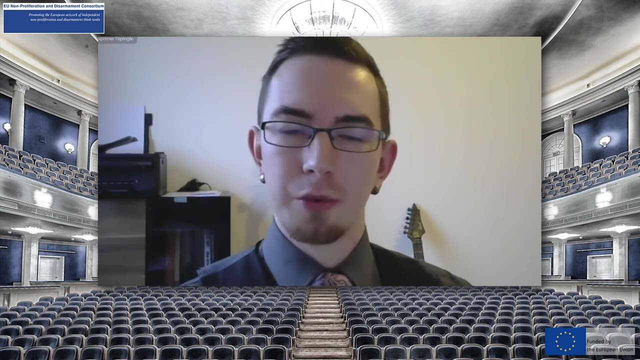 As I said, I think a follow-on treaty to New START could do a lot to address some of the concerns that people have raised in terms of hypersonics, in terms of perhaps other new and emerging technologies, although I agree with Naomi that hypersonics are certainly sort of easier to encompass in an arms control. 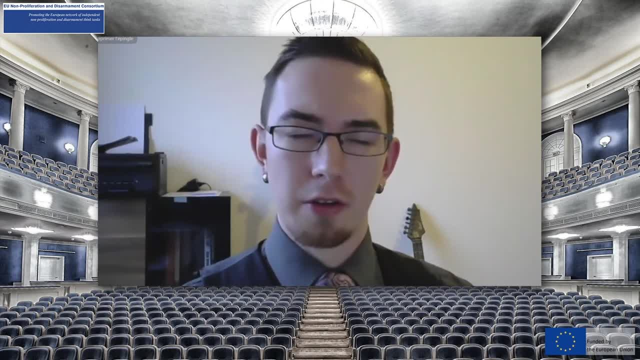 treaty in the traditional sense than perhaps other emerging and new technologies. This is also the reason that I said during my presentation that I really believe that a better way to go about a new arms control landscape would be to focus on ceilings for again. X. number of: 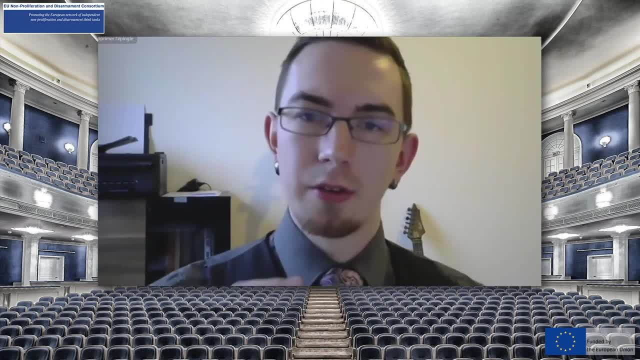 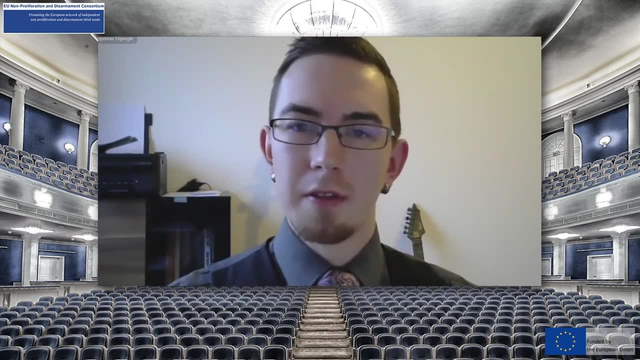 nuclear weapons on X, number on Y, number of delivery vehicles on Z kinds of basing would be a much better way to go about it than the classic US-Russian model, which has of course been just reductions And the reason I think ceilings is because it would be sidestepping the verification question and transparency. It would be much easier to motivate other nuclear-armed countries to join an arms control framework if, basically, it didn't ask them to do anything, But this doesn't mean that they wouldn't. 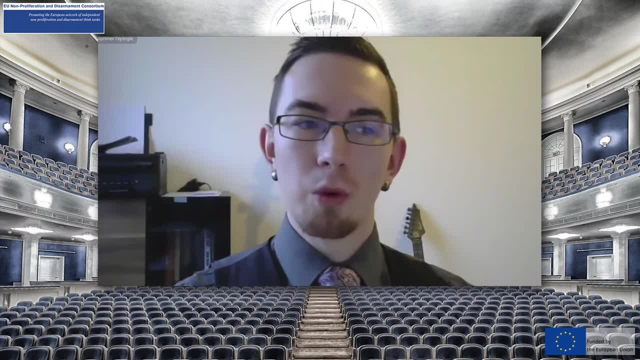 be contributing to the landscape overall. Imagine a world where all of the nuclear-armed- or at least the NPT nuclear-armed- nuclear-armed- countries would be contributing to the landscape overall. Imagine a world where all of the nuclear-armed- or at least the NPT nuclear-armed? 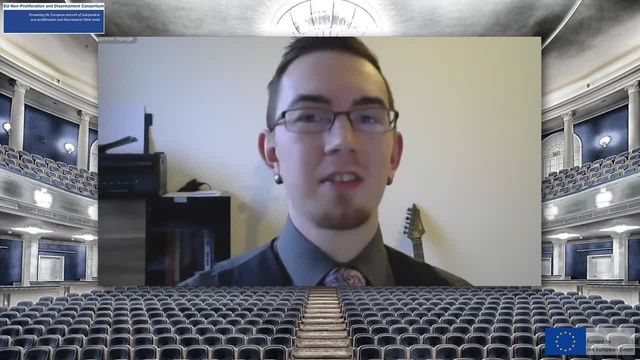 nuclear-armed states were under an obligation to not exceed a ceiling. Well, the US and Russia will have to reduce, but probably China, France and the United Kingdom could sit comfortably where they're at. This would be a positive motion in the non-proliferation regime, And if we don't limit 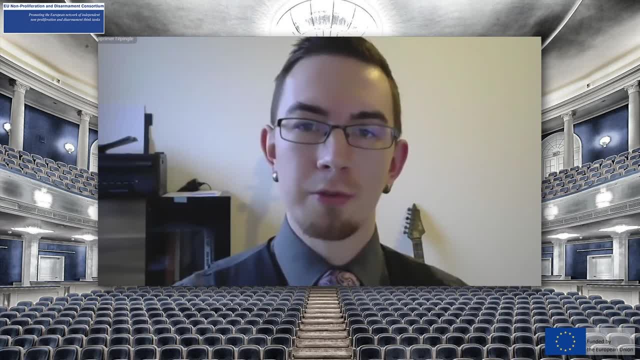 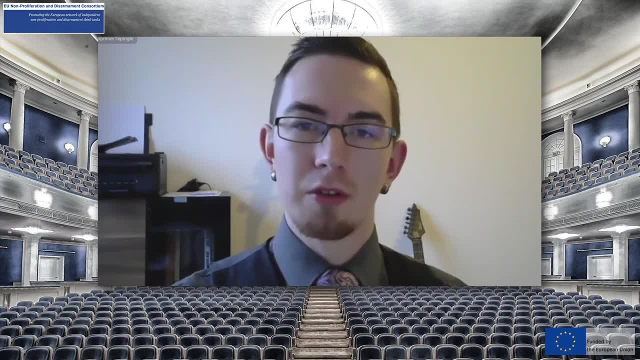 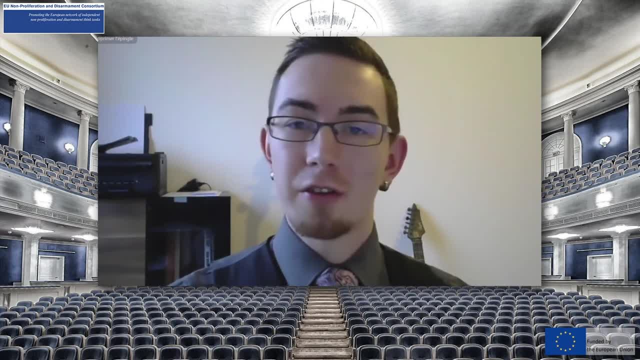 framework. Now verification I won't get into because that's a whole mess, but that's obviously something else that would need to be hammered out. And, going back to my presentation, a reassessment in how we look at each other's interests and how much we value arms. 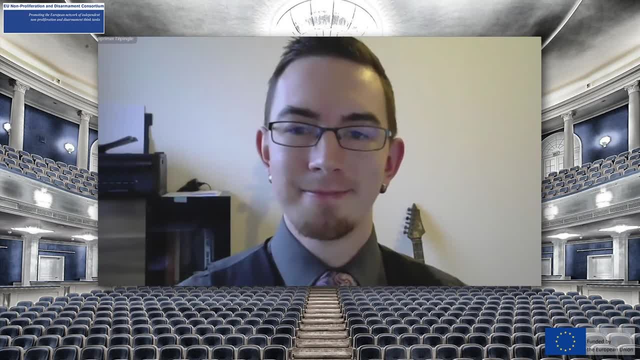 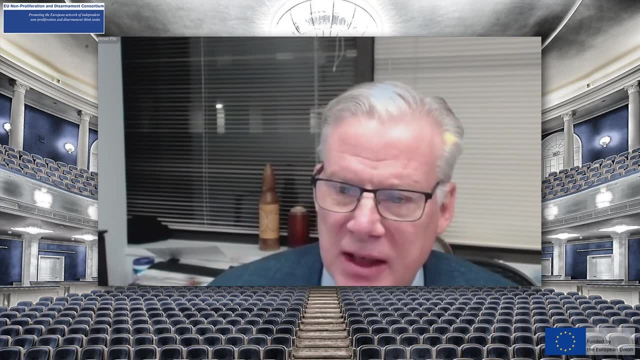 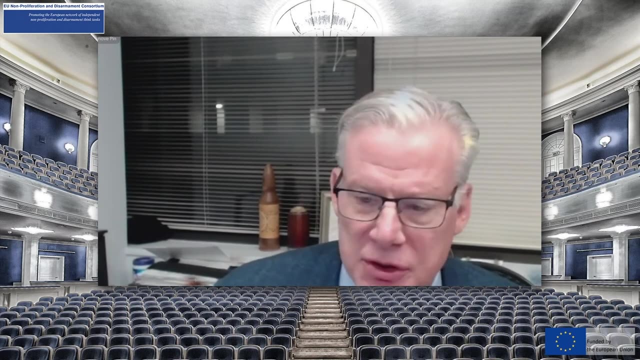 control for its intrinsic contribution to nonproliferation. Thank you, Noah. We're about four minutes over, but we started a little bit late So I'm probably not going to be able to get to the other questions directly. But before Emily, before you talk, I just wanted to ask, kind of. 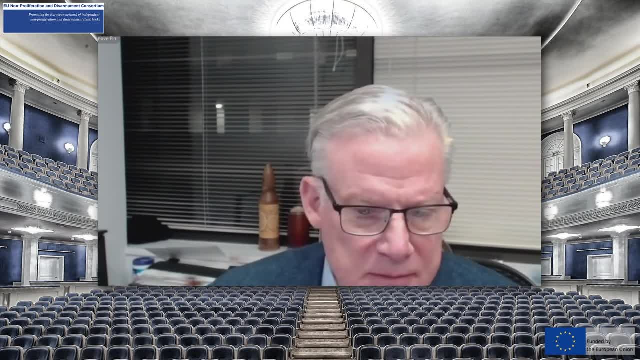 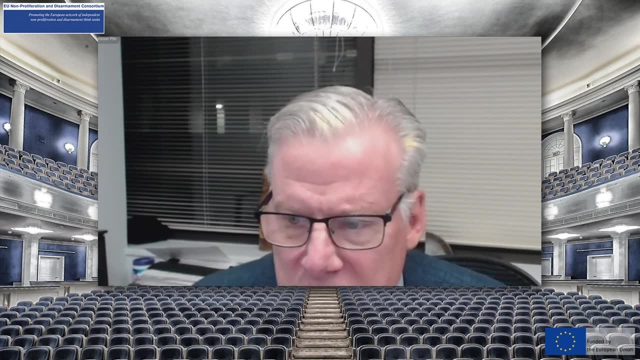 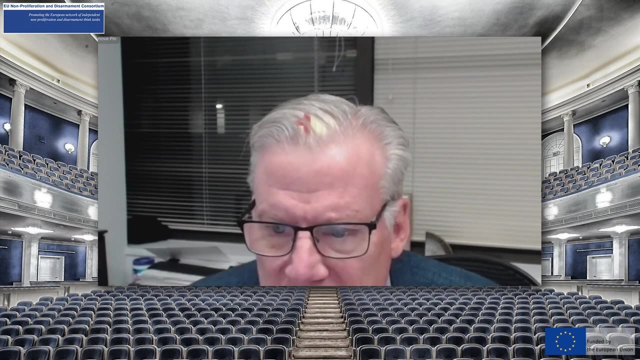 summarize the questions. One of them is about the modernization programs that are underway, without getting into too much detail. Another question was posed- let me see. it was arms control treaty, you know. or if they're truly multilateral, would they extend beyond the P5 or? 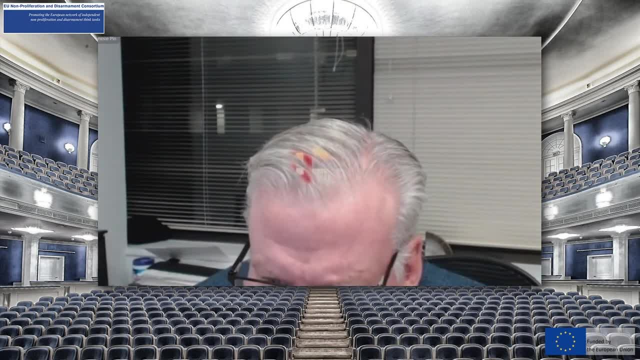 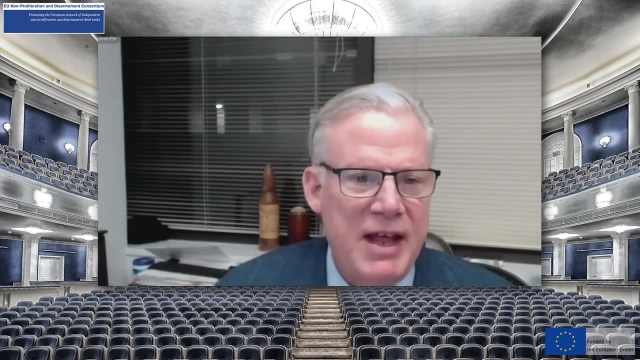 N5? And the role of big powers that they play in reducing arms and how that would impact perhaps India and Pakistan. So what I'd like to do is I'm going to hand the floor to Emily. You can answer any or all those questions very succinctly, And then I'm going to hand the floor to you, Emily. 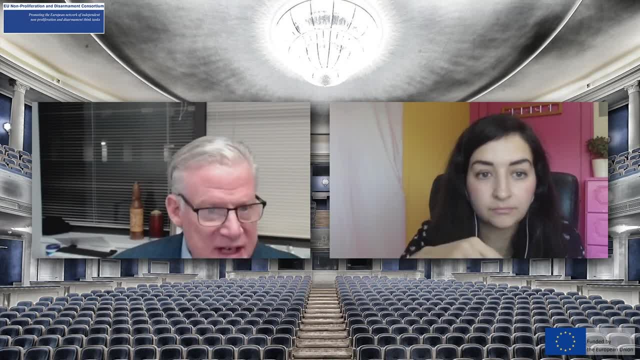 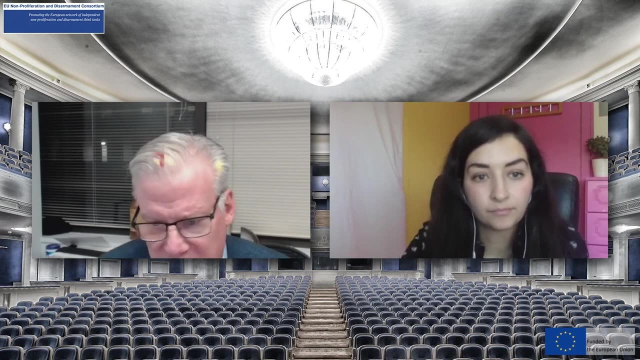 And if you have any other, like a summary statement that you want to make, to go ahead and do that, and I'll do the same then for Naomi and Noah. So if you could limit your comments to about two or three minutes so that we don't delay the next session and make the break all too short. 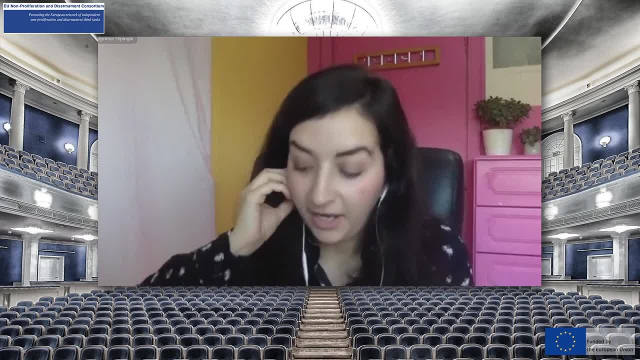 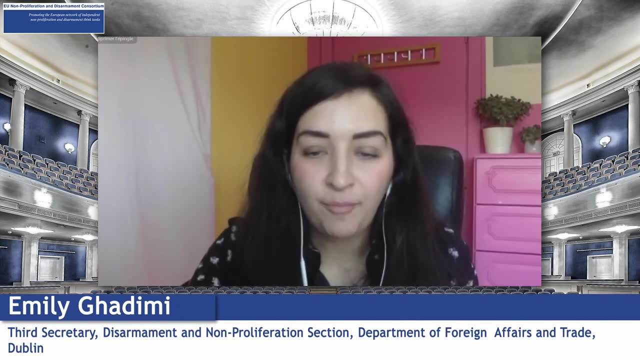 I would appreciate it. So, Emily, Thanks Mike. Yeah, I'll keep it very short, actually, because I think there's a lot of technical expertise that Naomi and Noah have, But just to just to sort of make a general point on that sort of trust piece in international law. 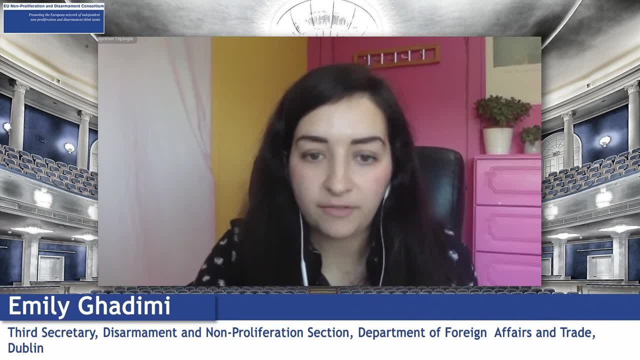 and in multilateralism. I mean, I think the first question of if the Biden administration will engage in arms control diplomacy, I mean I don't think that's an if. They've indicated that that's the direction that they want to go And I think it's very, very positive And indeed like 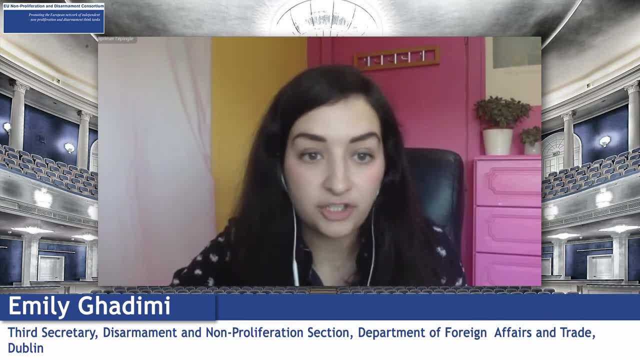 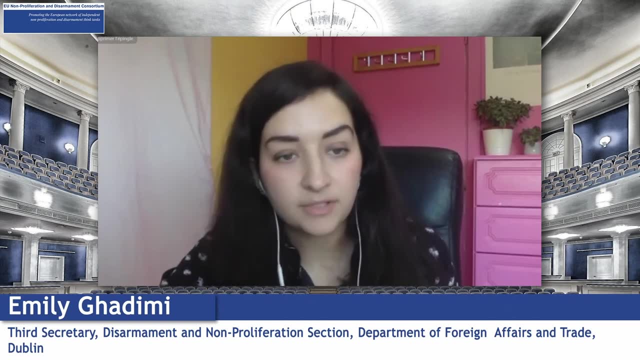 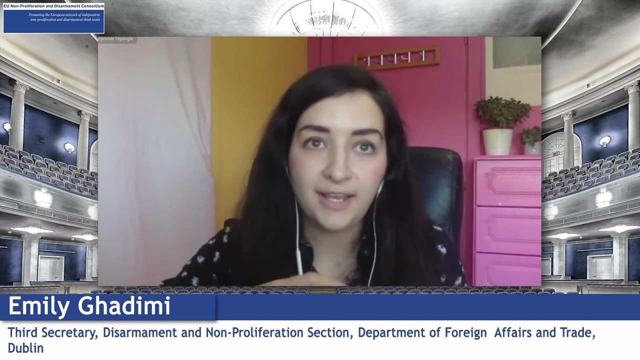 specifically on the JCPOA. I think there are certainly challenges involved in that. I don't think that Iran will be, you know, waiting with open arms for the US to come back, But I think there are pathways to do that, And I think just in sort of summarizing or giving like a kind of 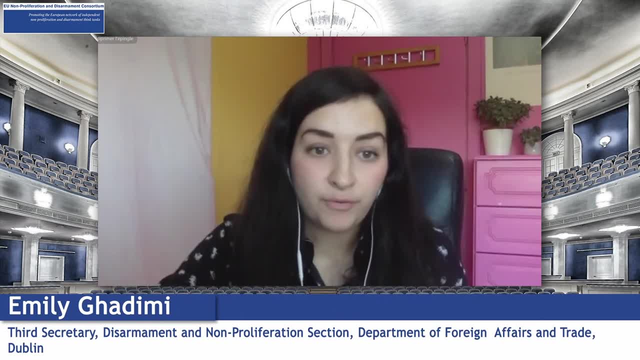 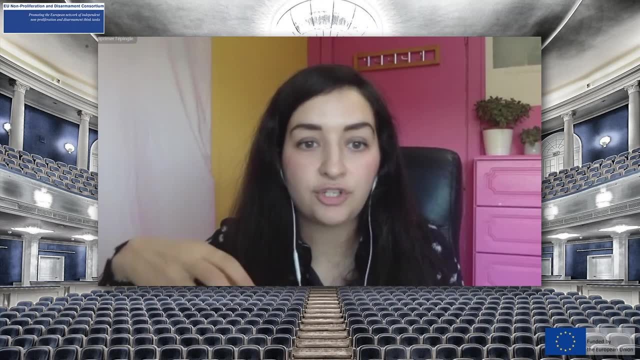 a vision for what I think would be good going forward is actually, you know, a point that we've touched on a couple of times is to engage states and broader stakeholders in these issues that have been, you know, not only in the past few years, but are often just negotiated by either the two. 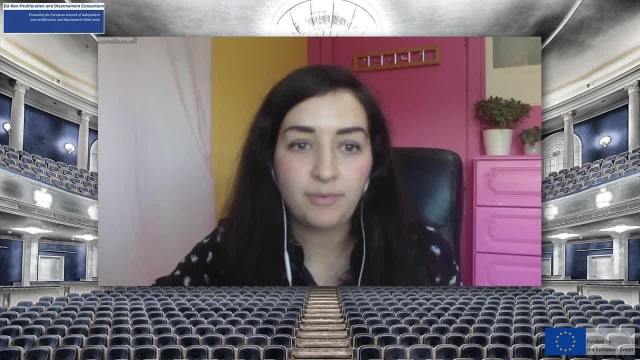 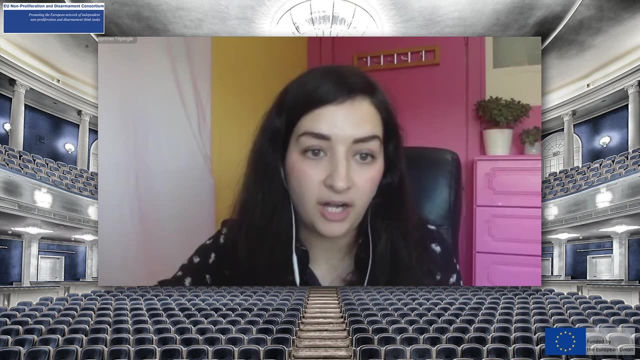 largest nuclear weapon states, or you know the P5. And I think what maybe the Trump administration has shown us is, you know, an opportunity for other stakeholders to step up into a leadership sort of role that, like that, these agreements are not entirely reliant on the political winds. 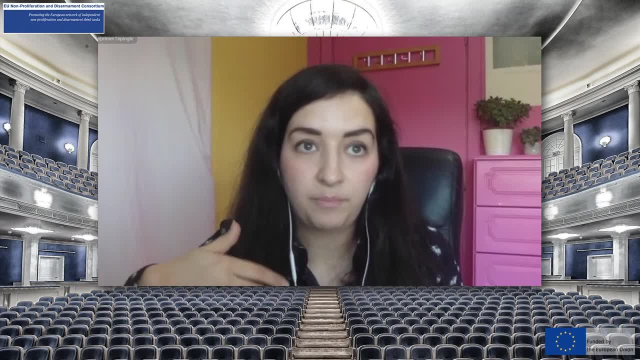 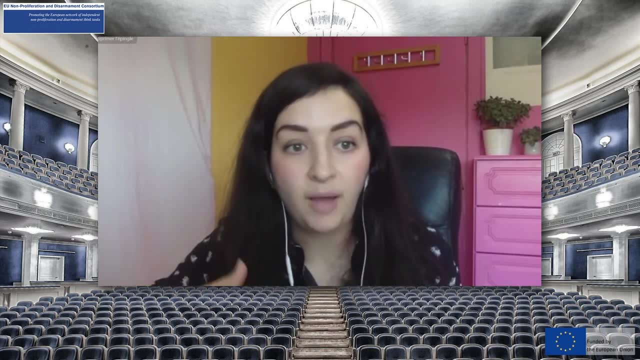 shifting And what I would love to see in the next, you know sort of following the next administration, is that we do actually, you know, maybe it is the EU stepping into a kind of a more leadership role on arms control, because a lot of these issues really do impact European security. But I think 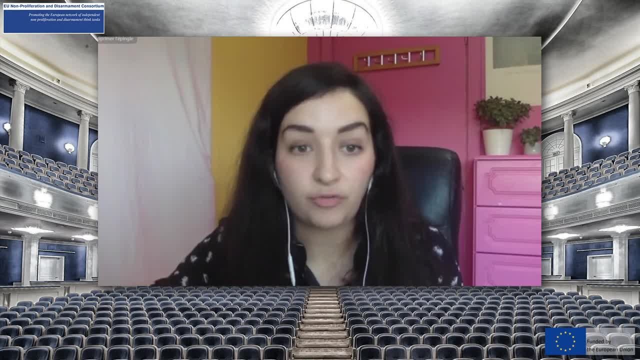 to sort of not have these agreements really reliant on one actor. of course it's important that the largest possessors of nuclear weapons are engaged in these issues, But it also affects all of us And I think you know. the TPNW shows that you know smaller. 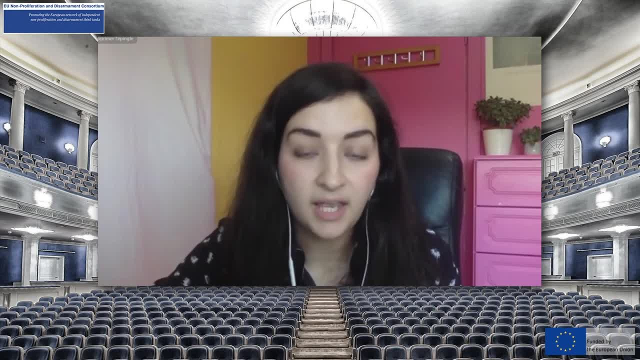 states do also have a voice and our stakeholders in this, And I'd like to see that kind of go forward as sort of more of the norm of how we engage in these conversations. But I think I'll leave it there because I'm sure there's other insights to be shared. But thank you so much again. 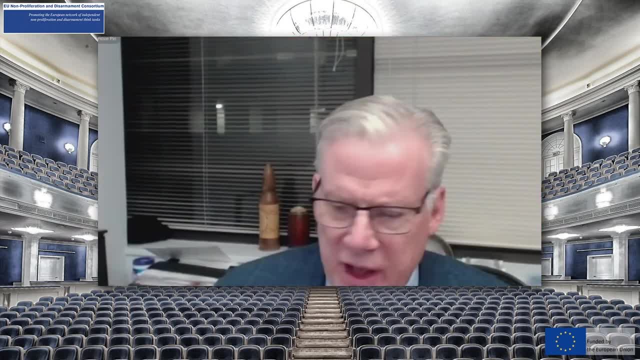 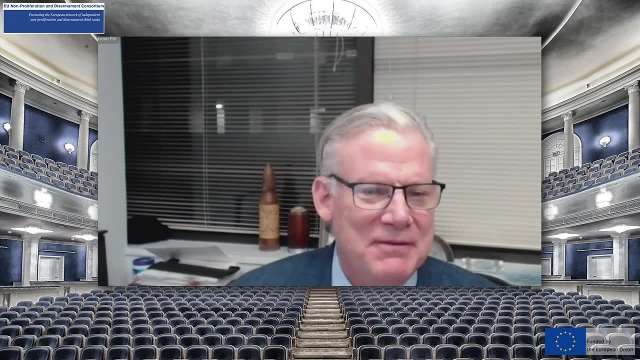 Great. Thank you, Ebony. Naomi, we have about. well, we're playing over. If you could just keep your comments to about 90 seconds or less, if that's at all possible. I hate to shortchange you, but you know the time is the time. So, Naomi. 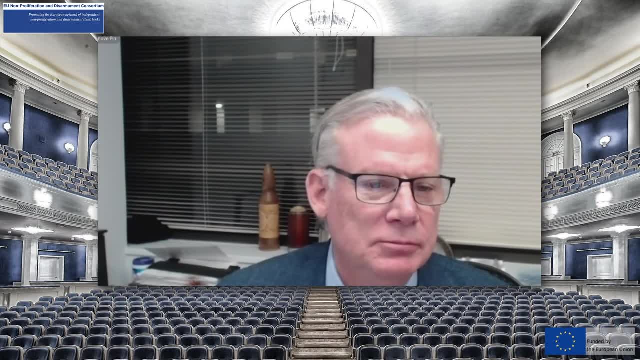 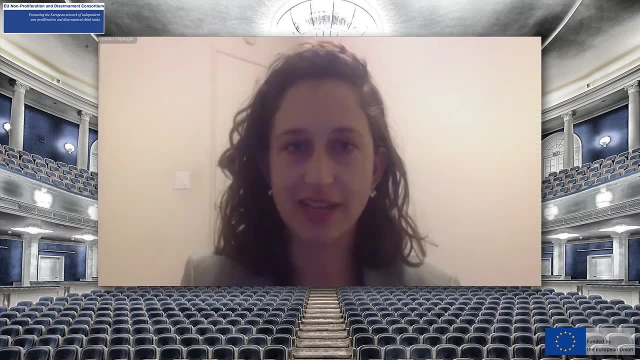 Happy to do so. So I'll just briefly respond to Sonia's question And I'll just say that certainly treaty withdrawal does set a negative example, But I'm more skeptical about sort of what role the big powers, as you put it, could play to reduce the arms race. between India and Canada. I think that's a really important question. And I think that's a really important question And so I'm not sure that treaty withdrawal necessarily has a direct impact on that. Now, if there was a multilateral treaty involving India and Pakistan and the United States and Russia, that might be. 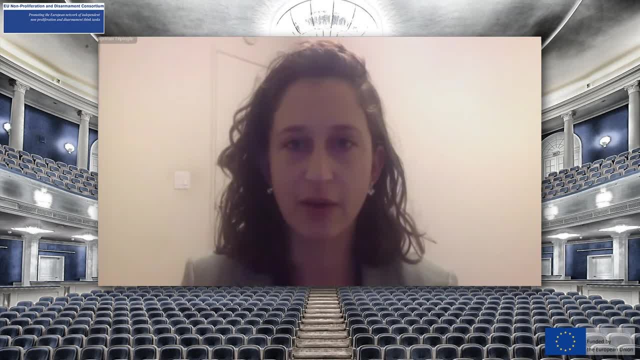 different, But that's not where we are right now. So I don't see too much of an impact on US withdrawal from treaties on the relationship between India and Pakistan. And then I'll just very briefly say that unfortunately I won't be able to attend the rest of the workshop as I'm in 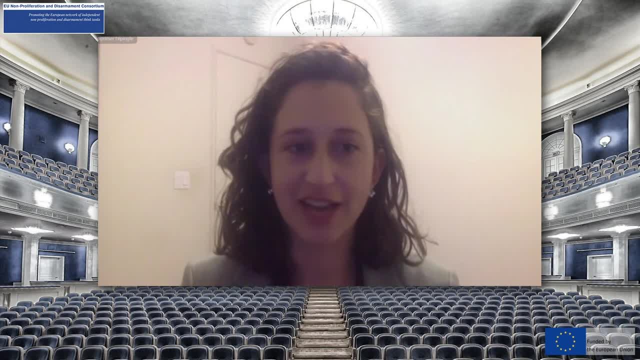 the US And it's quite late, But if anybody would like to chat more, I'll be checking messages on the platform And thank you all so much for the wonderful questions. Thank you, Naomi Noah. same to you In 90 seconds or less. I apologize for the shortness. 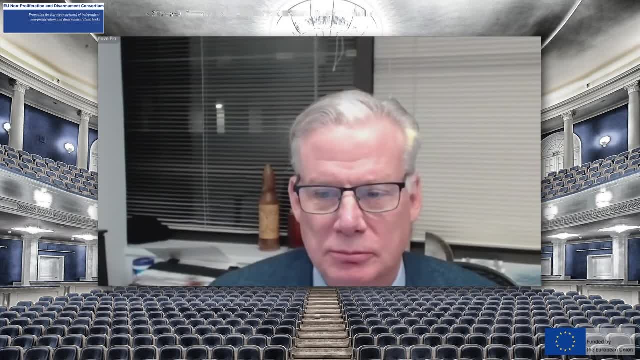 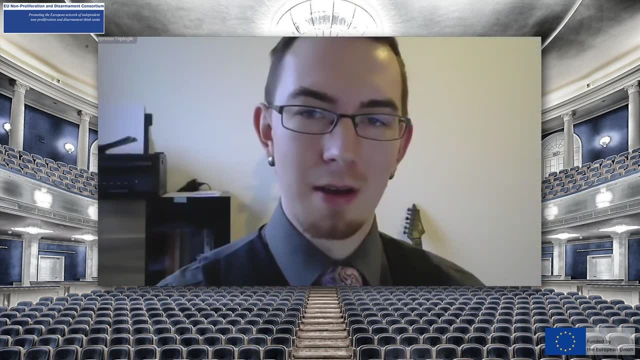 Oh, no problem, I will briefly look at these three questions remaining in the Q&A function. Modernization can't do much about it, Biden's not going to stop it, Trump didn't stop it, And you know. that's just sort of where we are. Prospects for European strategic stability. 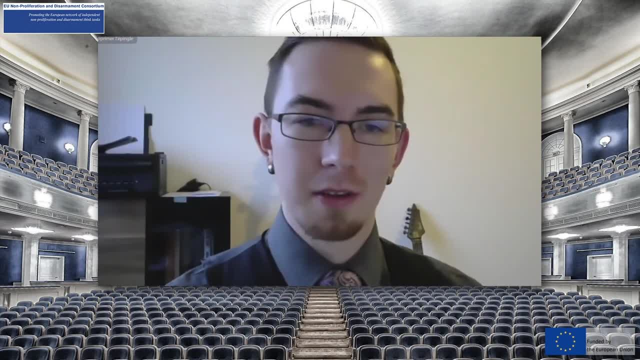 and post-INF scenario. As I said, I'm desperately hoping that there will be some sort of- at least politically binding statement about deployment of INF-type missiles in Europe, And I think we really need that. But European security can be well armed by Europe, as I said, 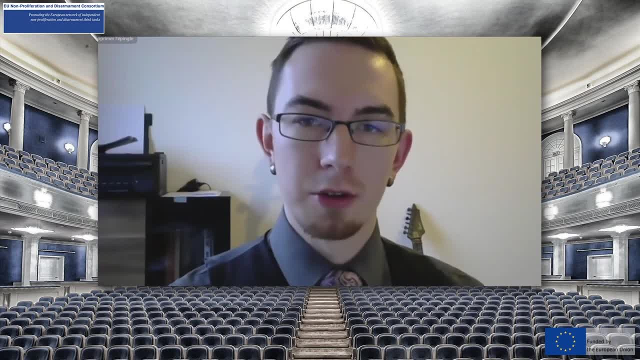 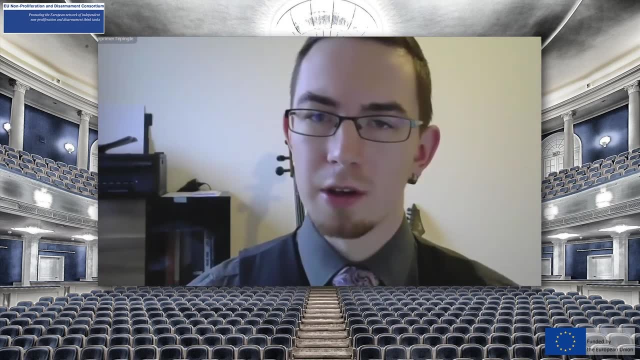 earlier taking a much more active voice in multilateral security affairs, which Europe is already starting to do. I want to mention, in addition to a conference held a couple of weeks ago by the German Federal Foreign Office on Arms Control and Emerging Technologies that received 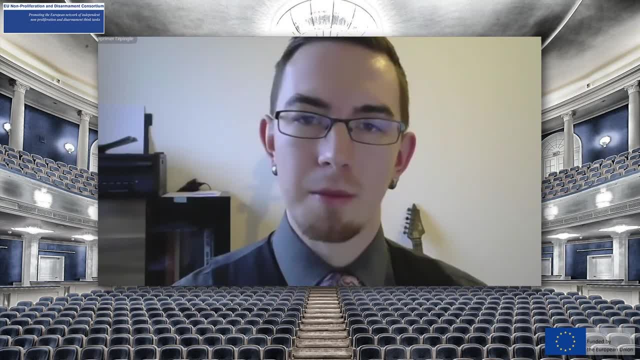 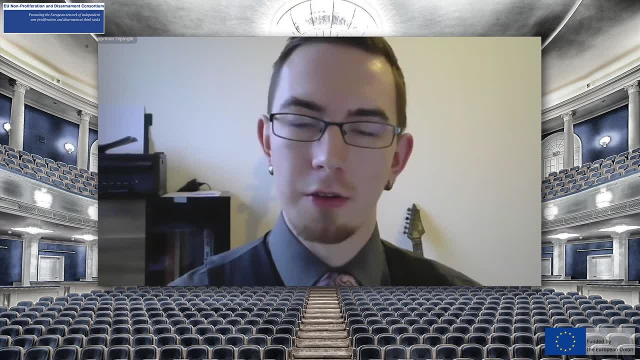 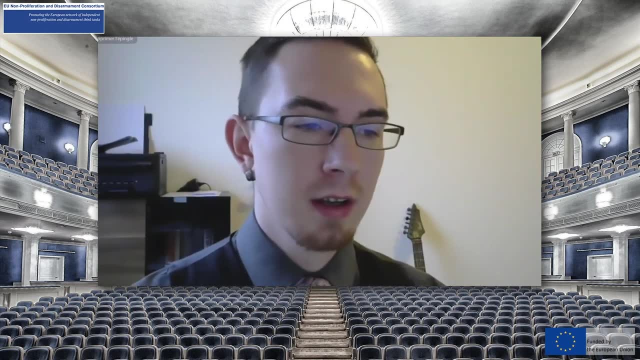 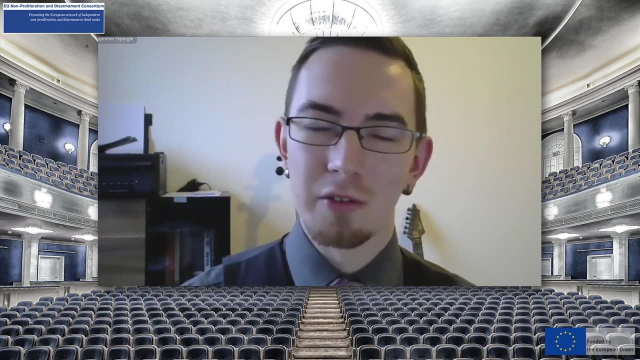 But that will remain to be seen how effectively we can take each other's interests into account while having that discussion and what verification would look like. I think Naomi hit the nail on the head with the India-Pakistan question. I'll agree with her that withdrawing from treaties is not a particularly effective way to show leadership. 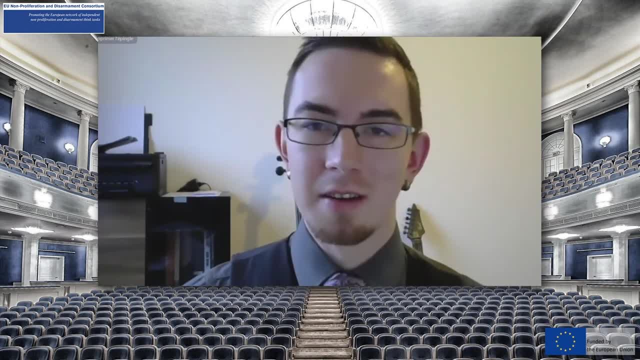 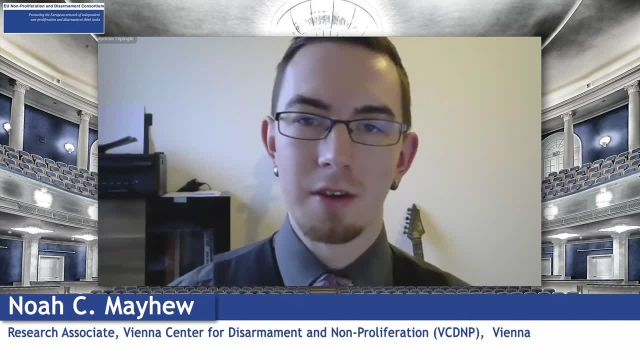 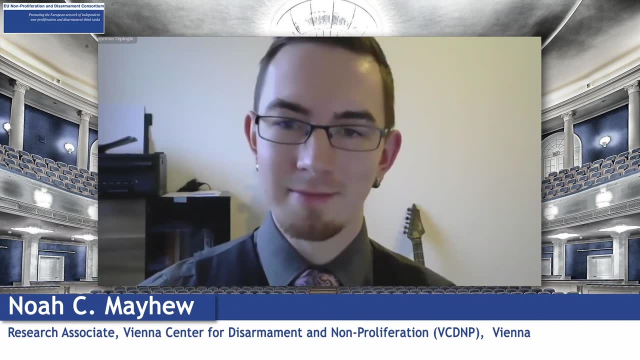 appreciate that. All of my info, email address and whatever is on the VMC DNP website. please feel free to write to me and I'll be happy to chat. Sixty, there we go And now. thank you very much to all of you for listening. Thank you, Noah. I want to. 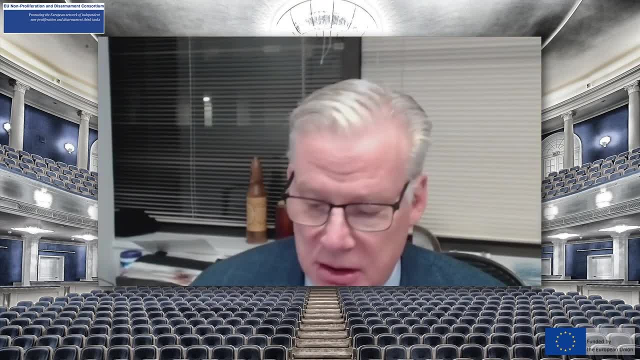 congratulate and thank all three speakers. I've been very, very impressed with not only your knowledge but the conviction with which you express it and the factual basis for your conclusions. I think you're asking for something. Thank you very much. You made a really parts time point to be here. so good to see you. Thank you Over and. 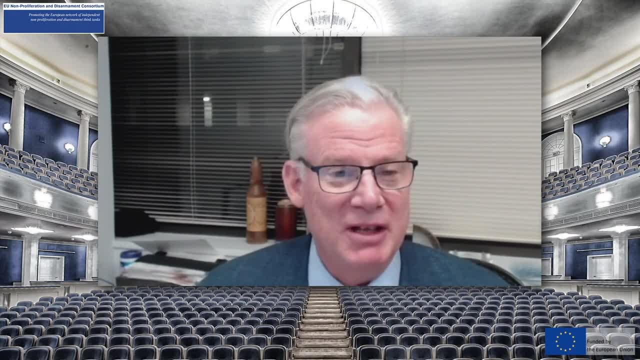 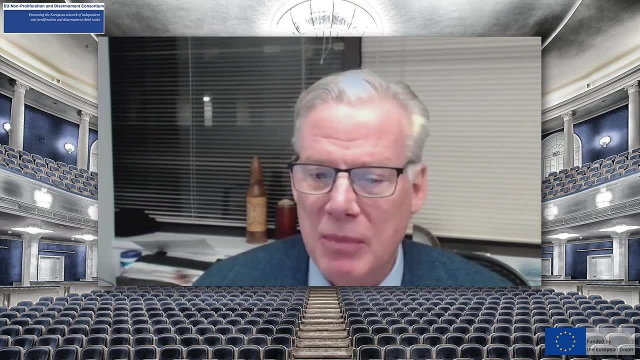 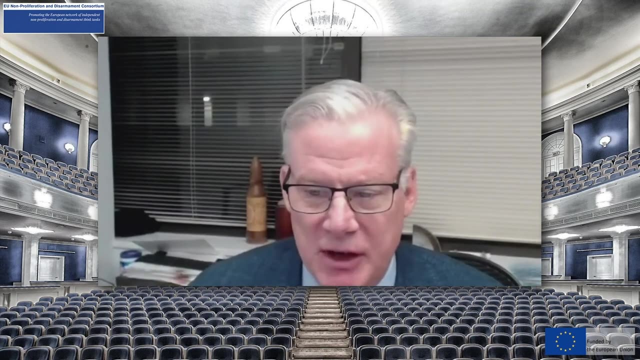 I think the future is really bright when I look and see some of our emerging next generation specialists in this area, And I would also like to thank those that posed questions from the audience and, of course, to Federica for her organizational skills and getting us all online here.